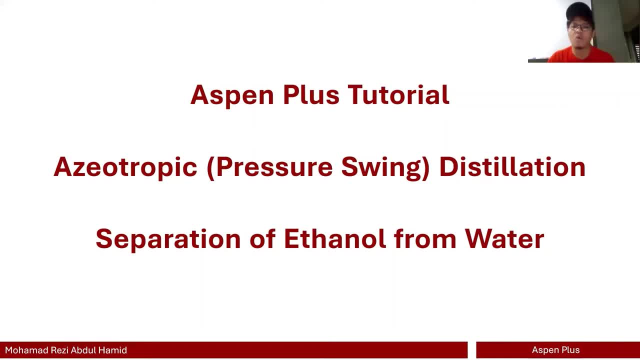 But for these videos I'm going to focus more on pressure swing distillation method. The same goes with the chemical or binary system. There are a lot of binary mixtures that exhibit azotropic behaviors, which we will explore later, But in these videos I'm just going to focus on the ethanol water binary mixtures. 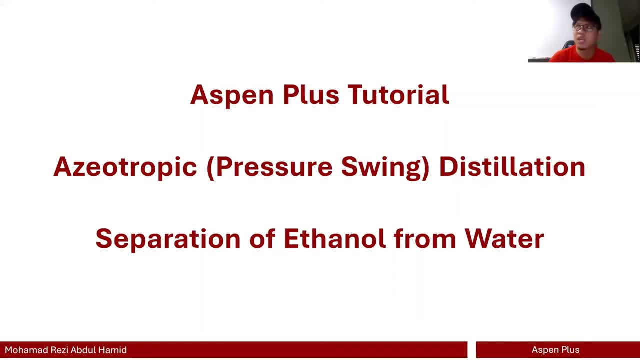 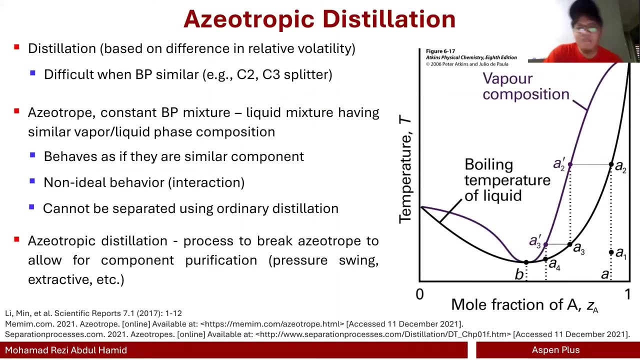 And we will try to separate the mixtures using a distillation column block in Aspen. So, without further ado, let's begin. So I'm going to begin my videos by giving you a brief introduction about azotropic mixtures, as well as azotropic distillation. 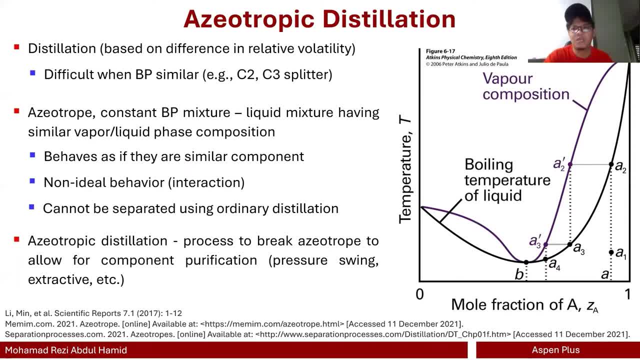 This is not a detailed description about the behaviors of the molecules from the microscopic point of view. This is just a general introduction. We all know that the separation processes using distillations are all based on the difference in relative volatilities. Now, the higher, the larger the difference in relative volatilities, the easier for them to be separated. 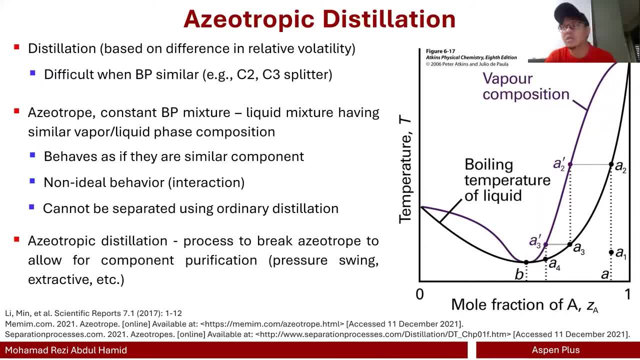 Now things become more difficult when we consider mixtures having a relatively similar boiling point, For example. obviously, when we talk about similar, Similar boiling point separation- for example, C2 splitter as well as C3 splitters to separate ethylene from ethane as well as propylene from propane- these two mixtures are quite difficult to be separated because they have a relatively similar boiling point, or where the difference in boiling point are just three to four degrees Celsius. 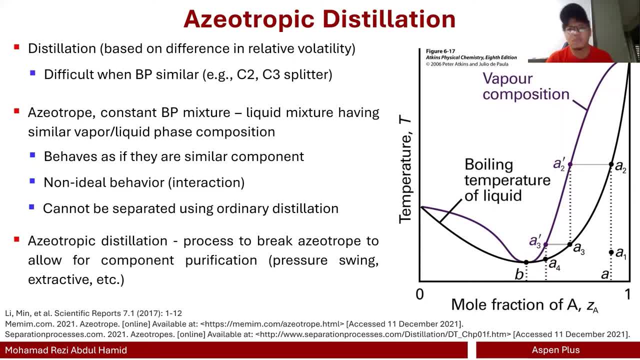 Now, it is not because of this. It is not a surprise that our mixtures have a relatively similar boiling point. It is not a surprise that our distillation column, or C2 or C3 splitters, can have a number of stages, up to 200, and they operate under high reflux ratio, which makes them one of the most energy-intensive separation processes. 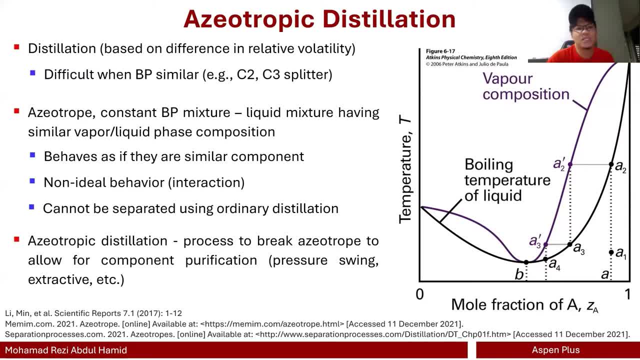 Now, what is azeotrope? Okay, azeotrope is basically a constant boiling point: mixtures: At this condition, the mixtures behave okay, even though we have two mixtures, two components. At this condition, the mixtures behave okay, even though we have two mixtures, two components. 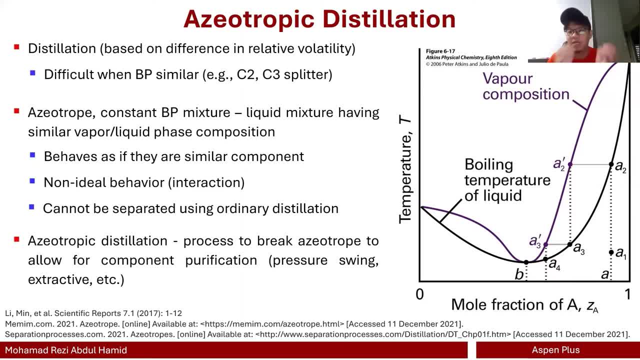 At this condition, the mixtures behave okay, even though we have two components. At this condition, the mixtures behave okay, even though we have two mixtures, two components. At this condition, the mixtures behave okay, even though we have two mixtures, two components. 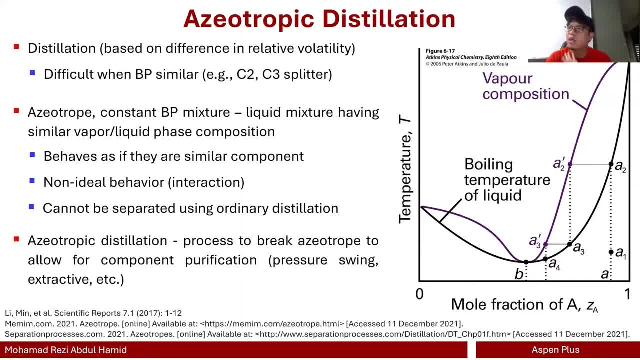 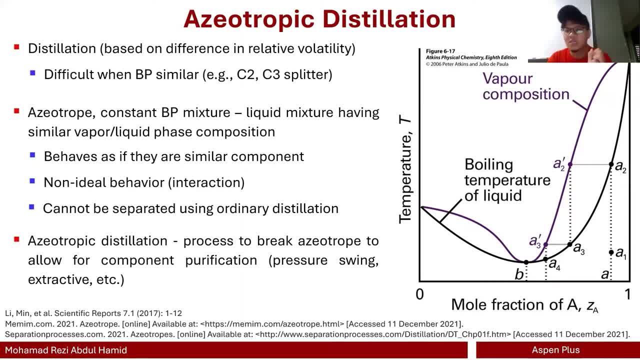 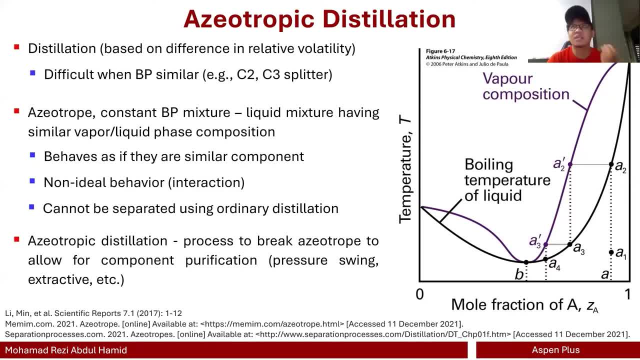 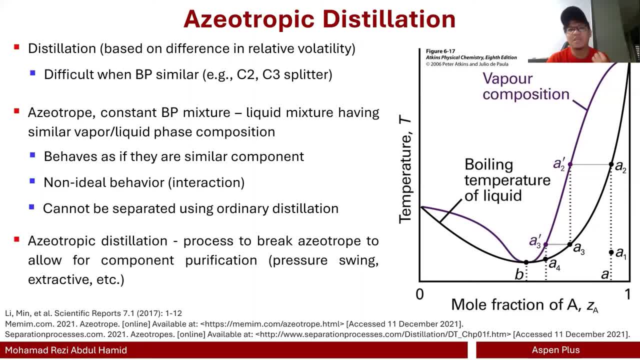 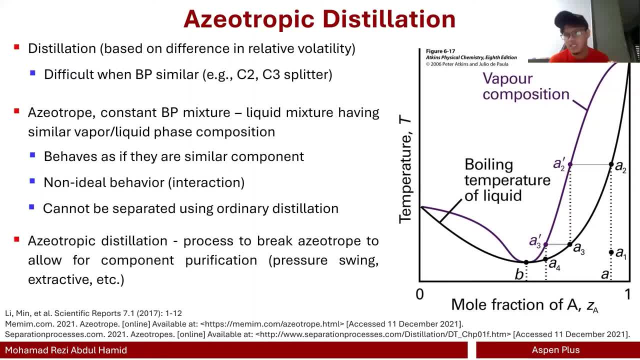 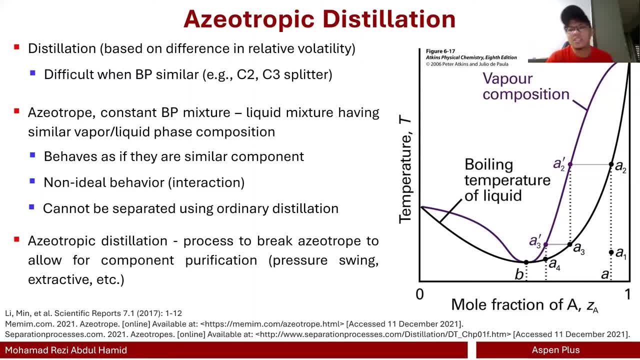 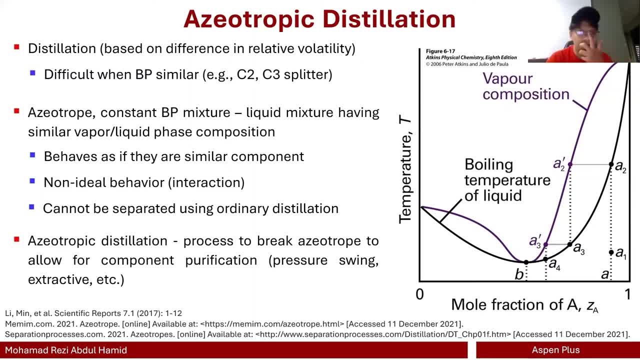 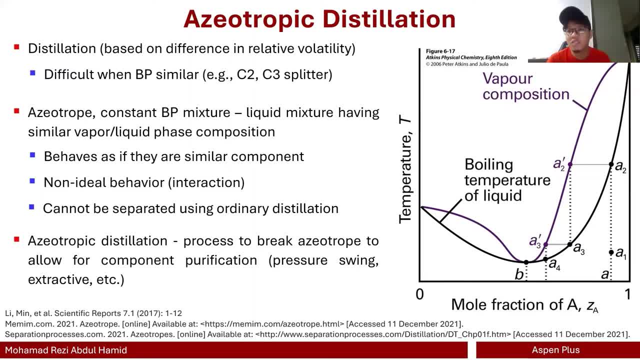 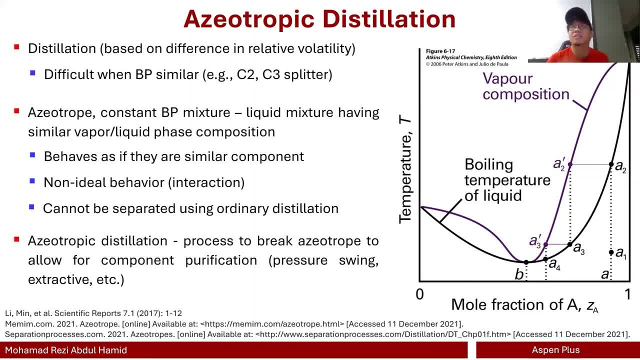 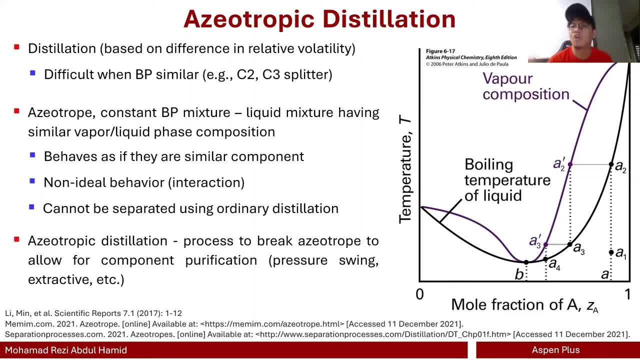 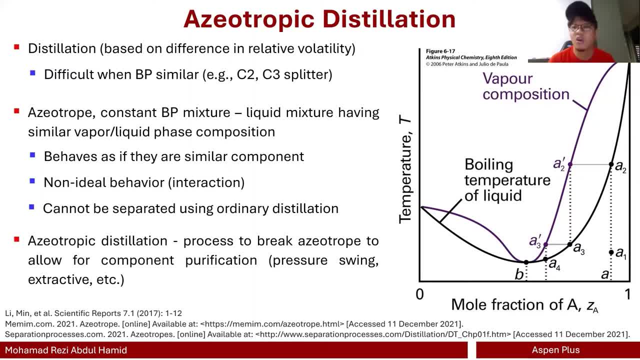 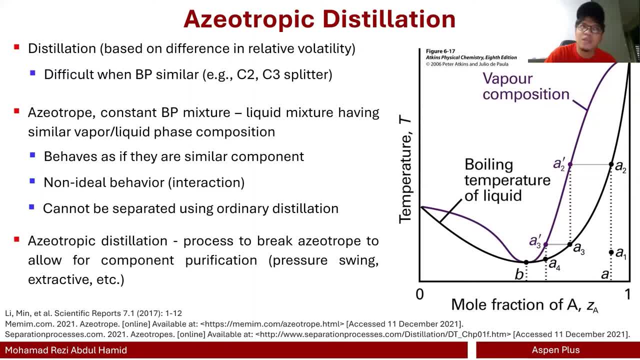 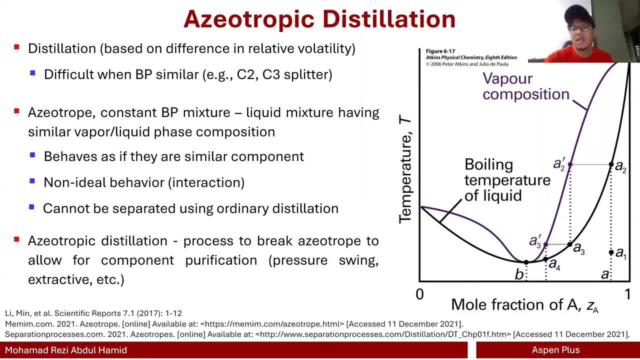 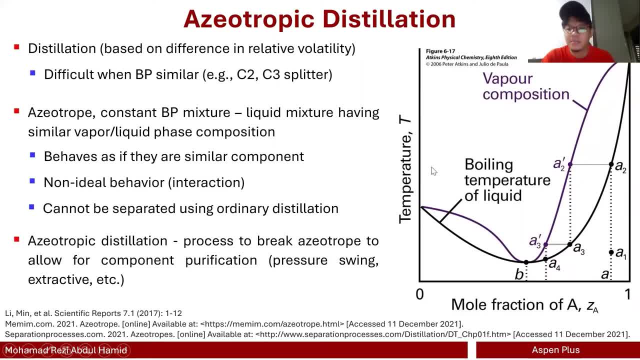 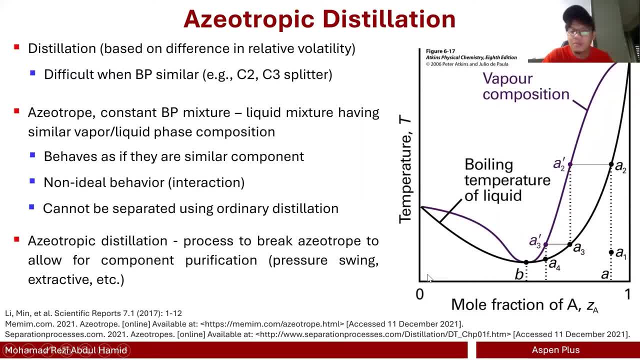 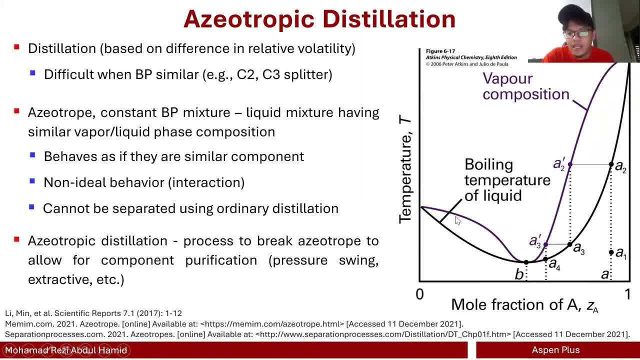 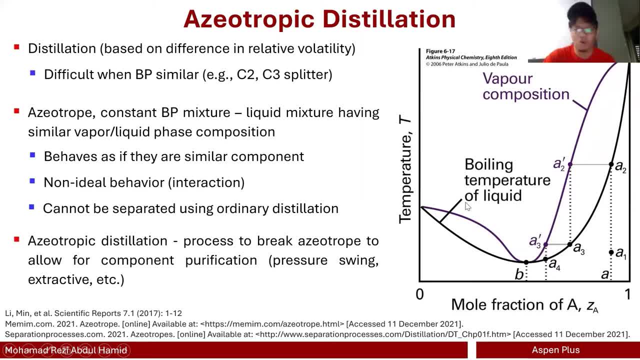 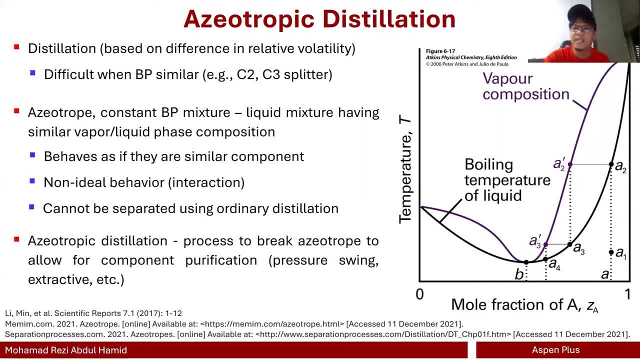 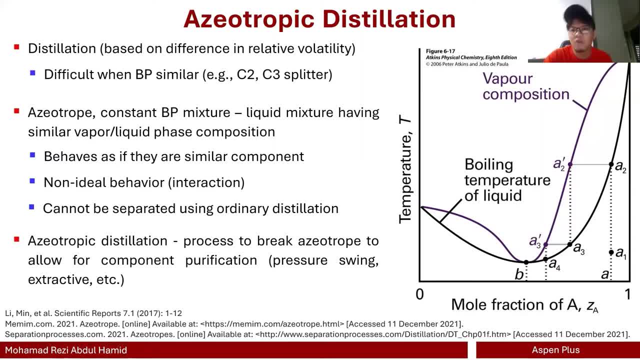 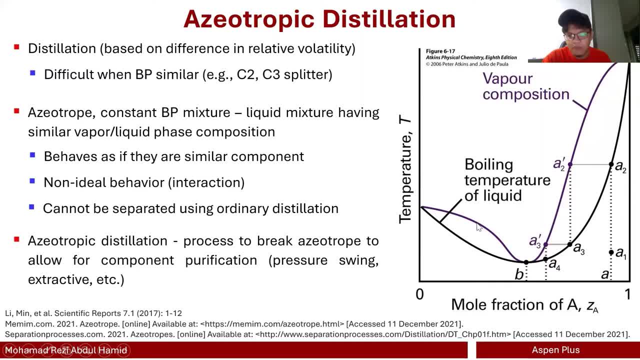 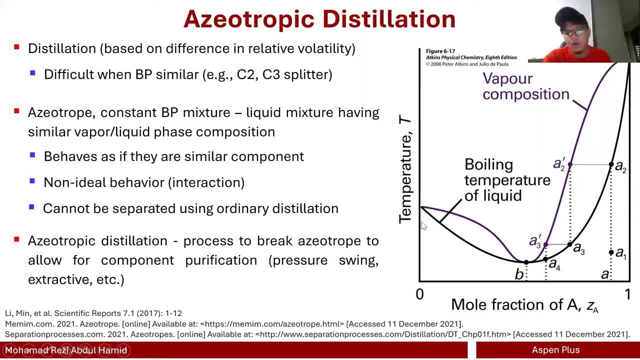 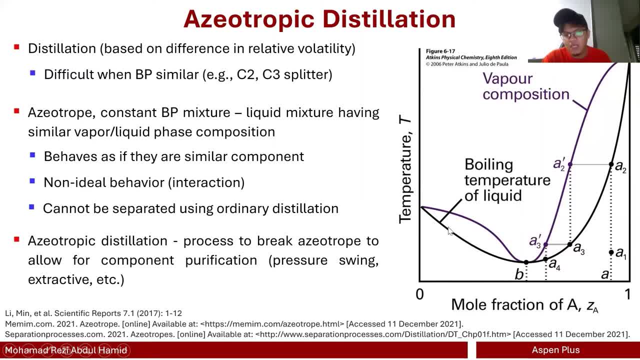 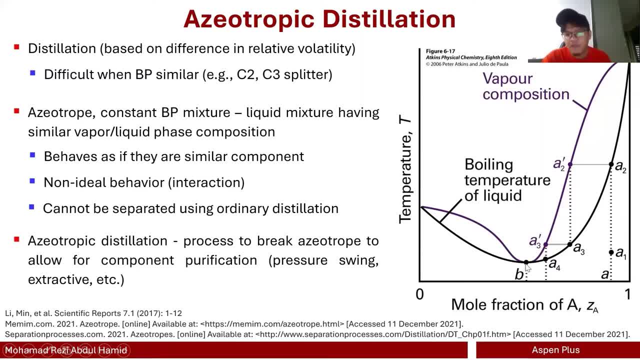 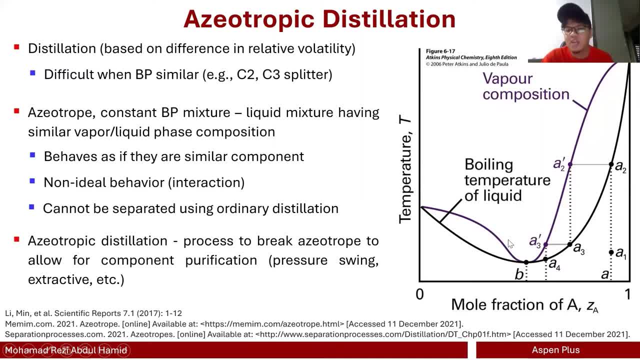 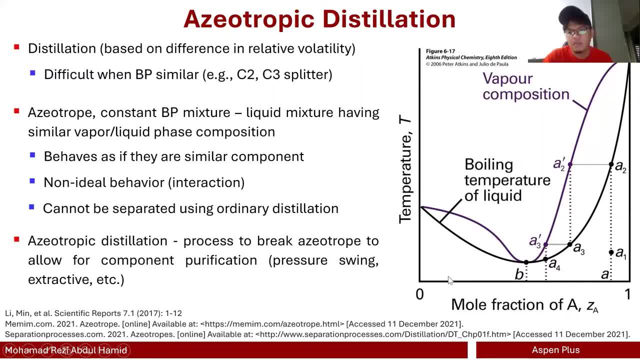 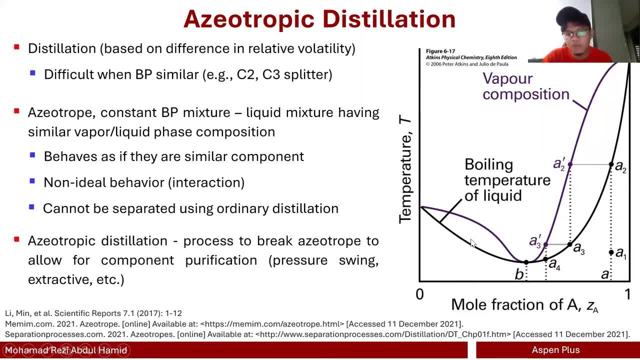 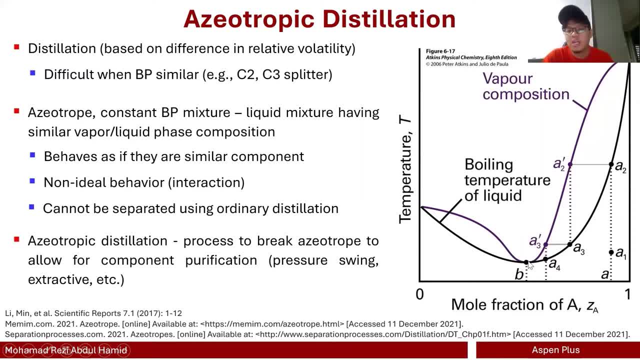 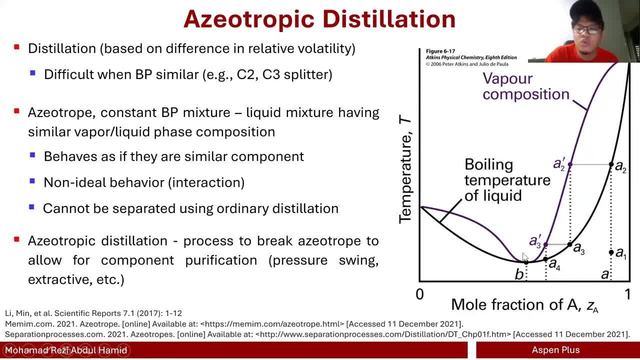 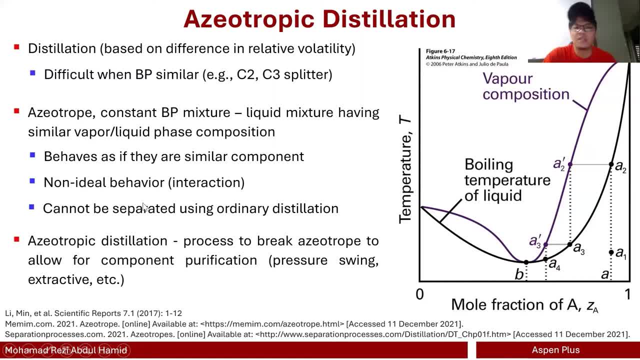 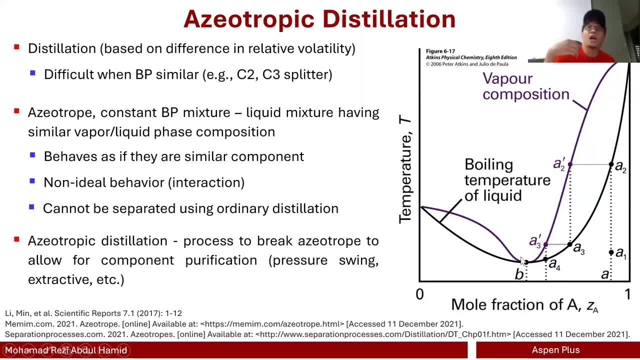 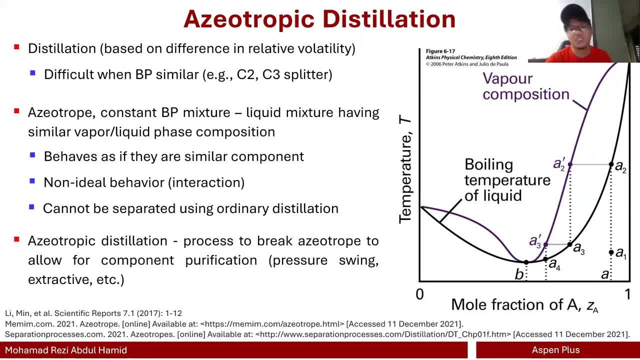 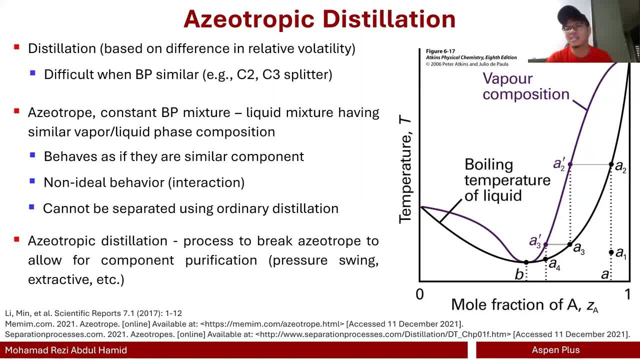 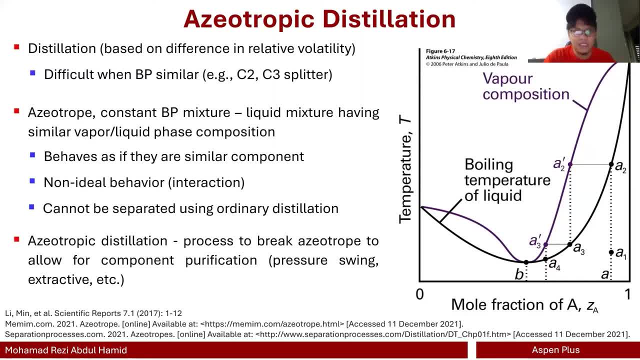 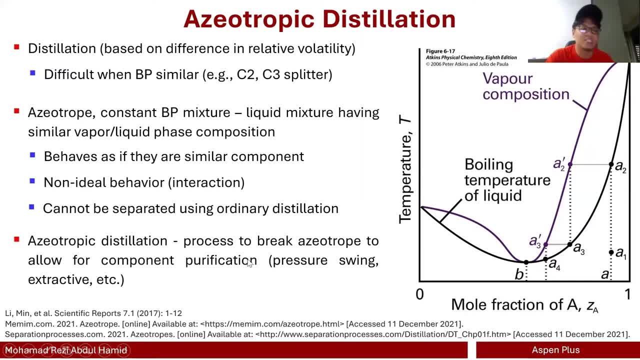 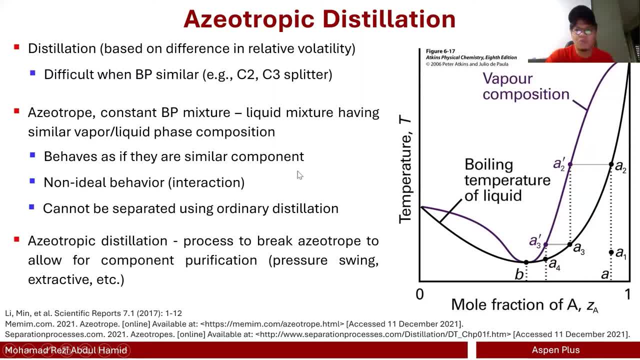 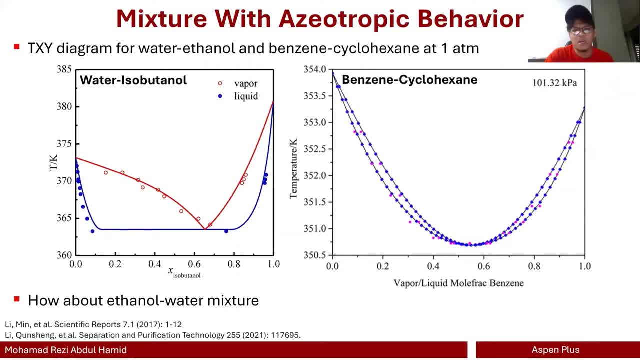 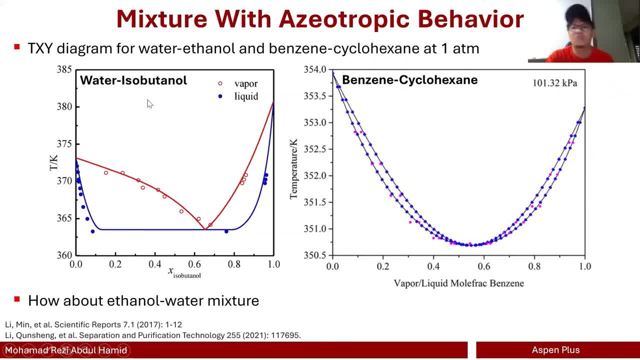 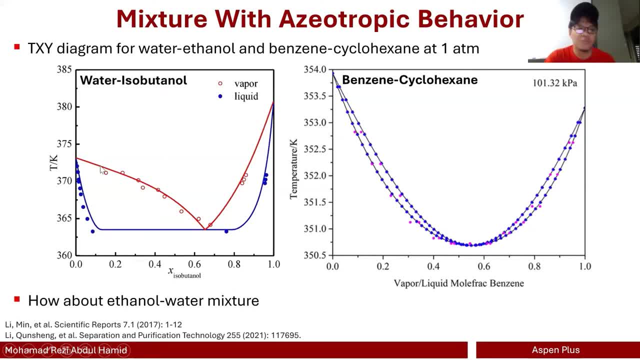 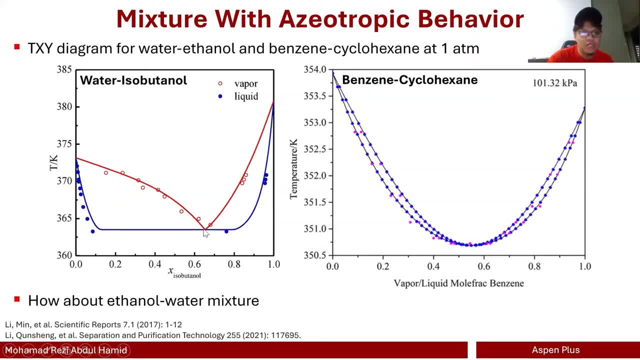 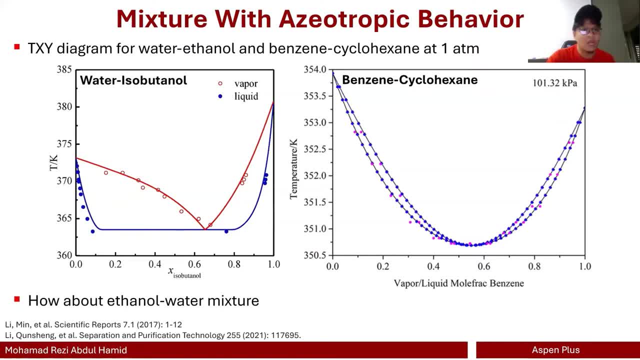 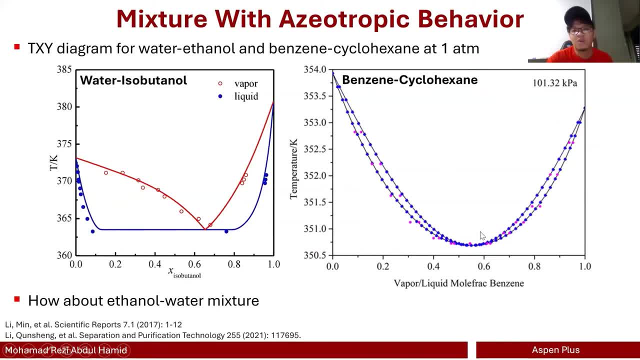 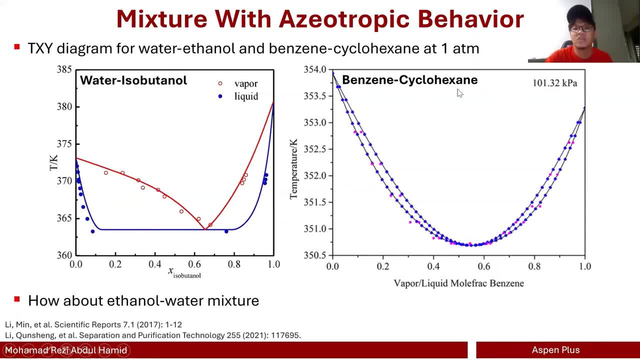 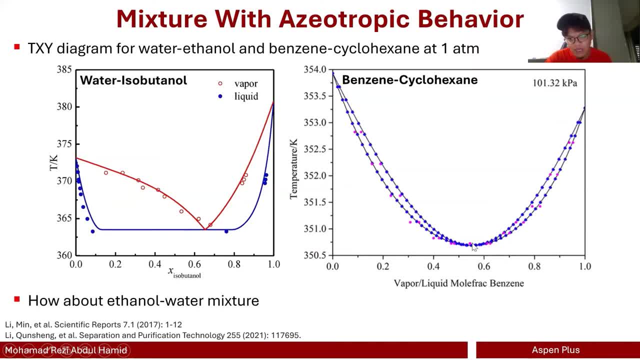 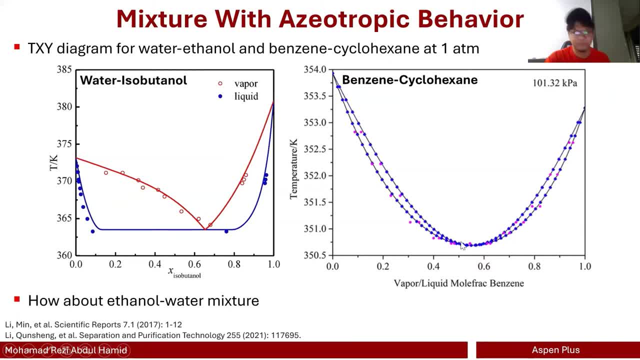 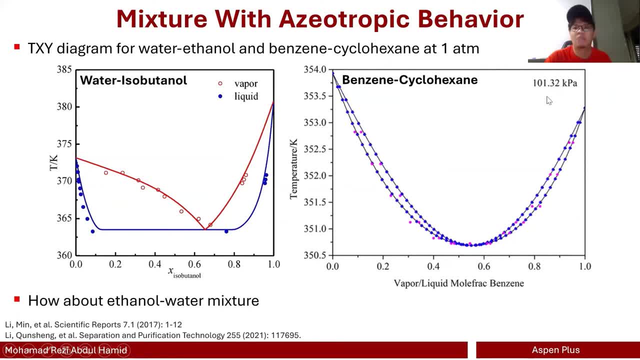 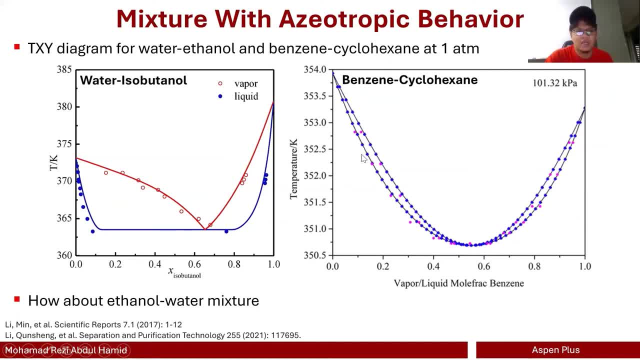 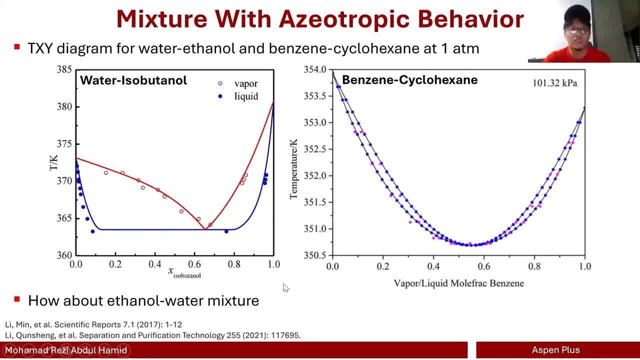 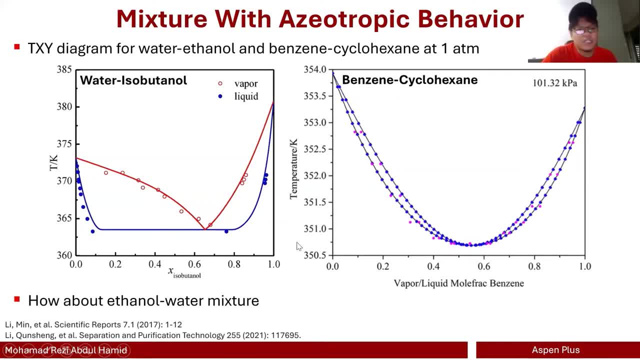 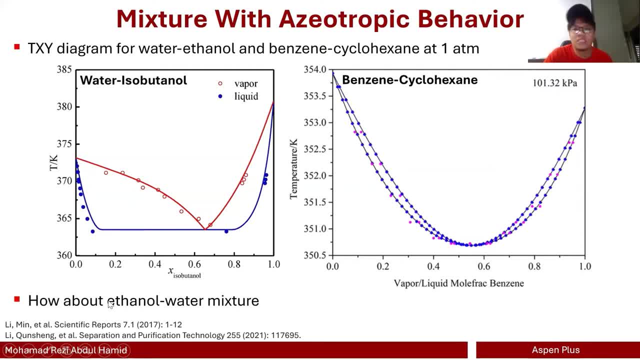 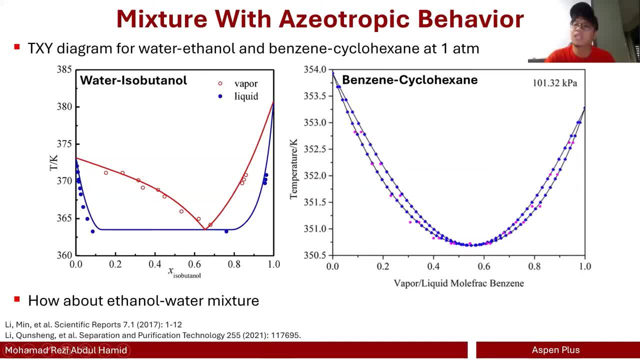 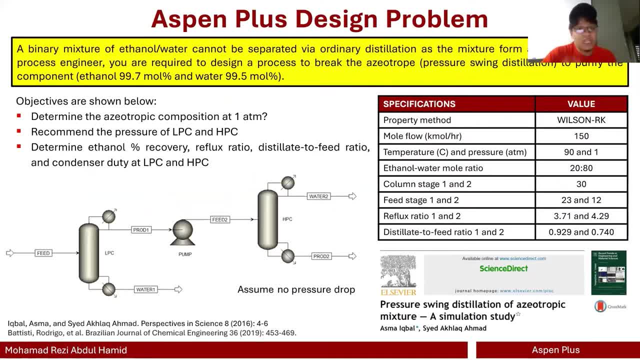 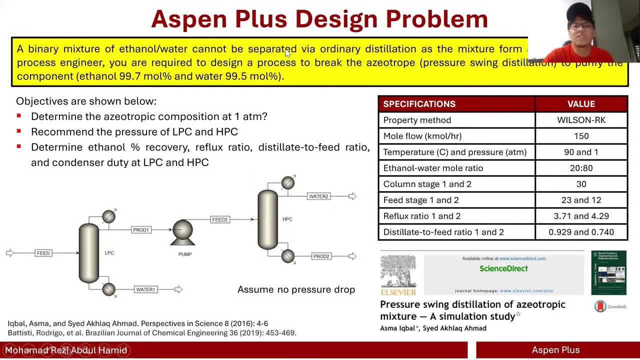 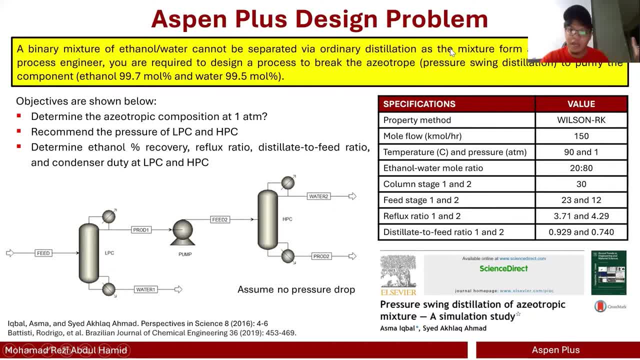 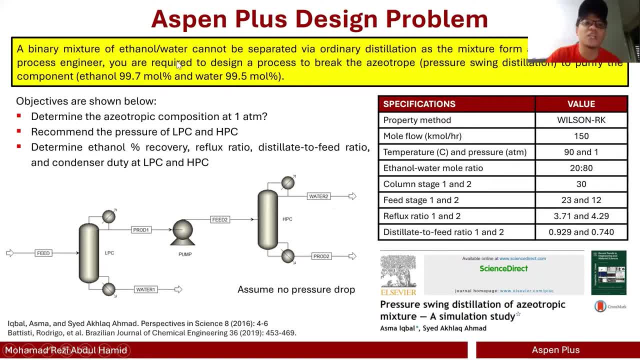 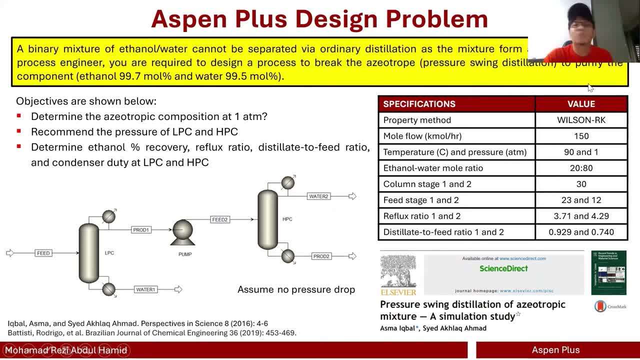 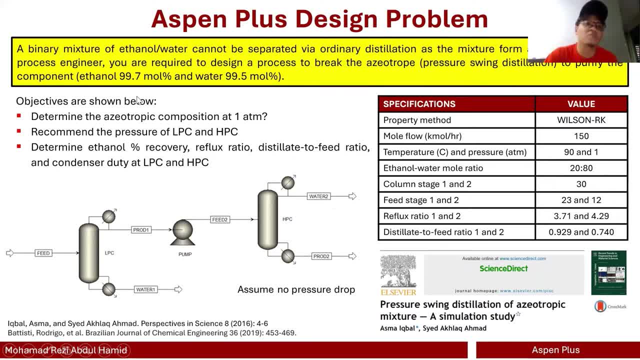 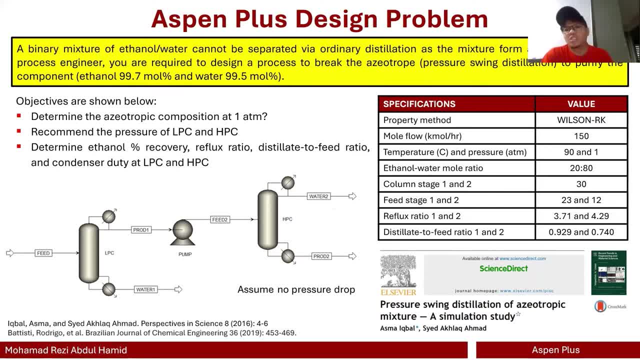 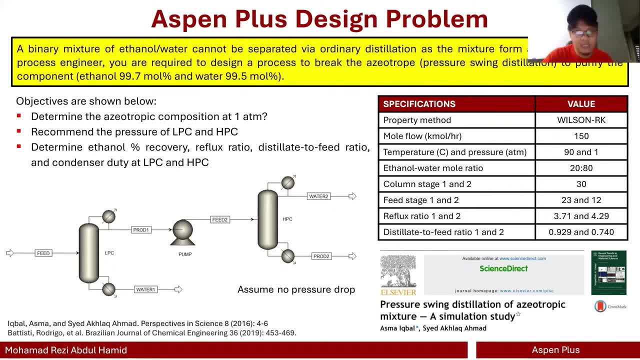 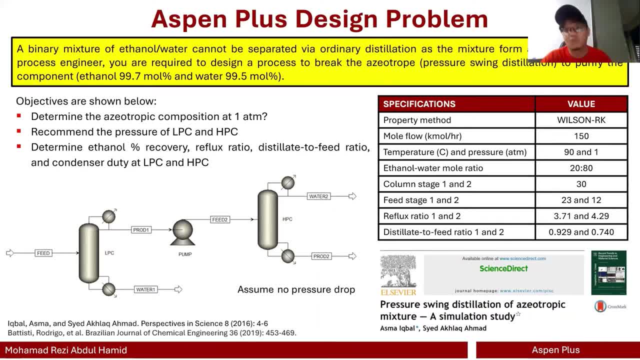 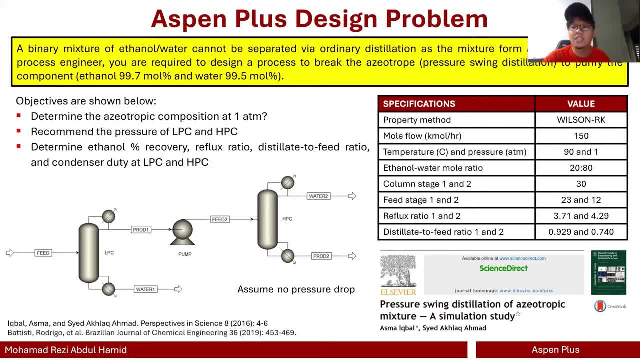 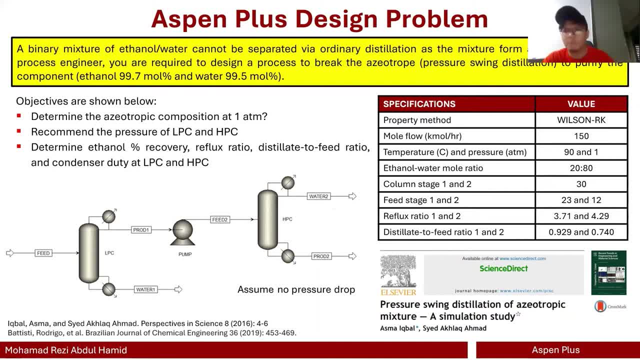 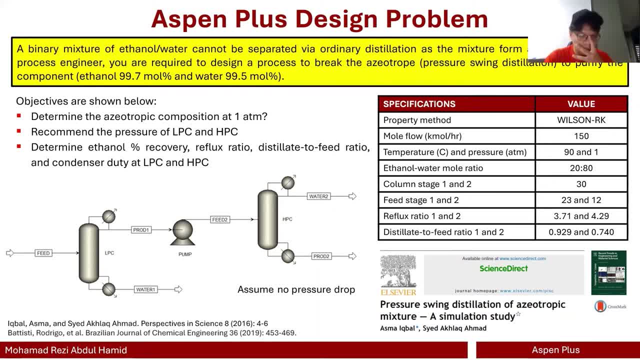 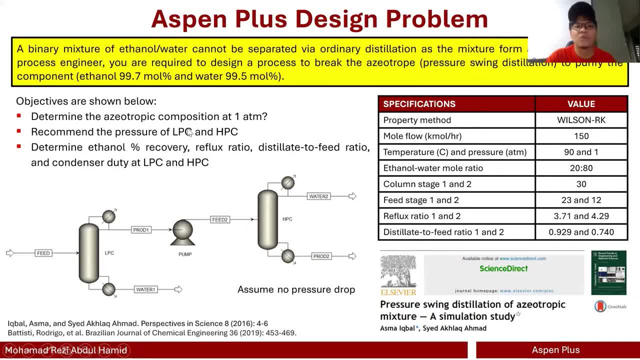 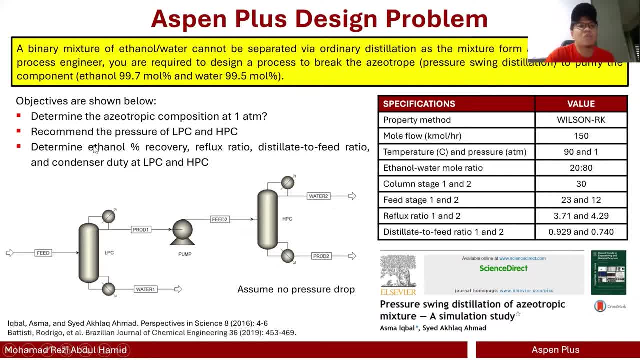 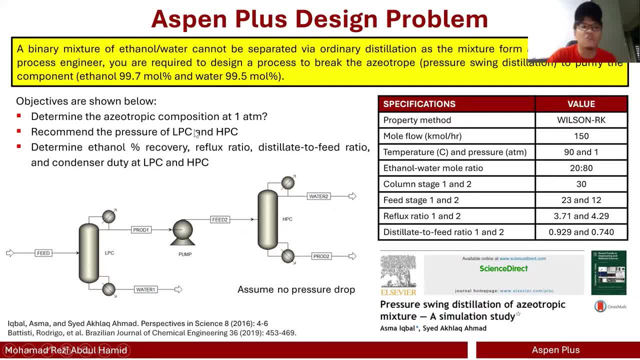 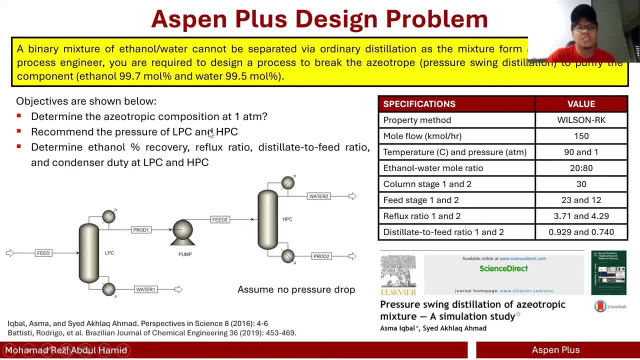 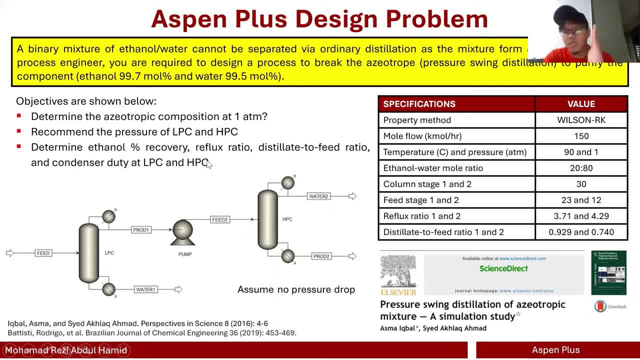 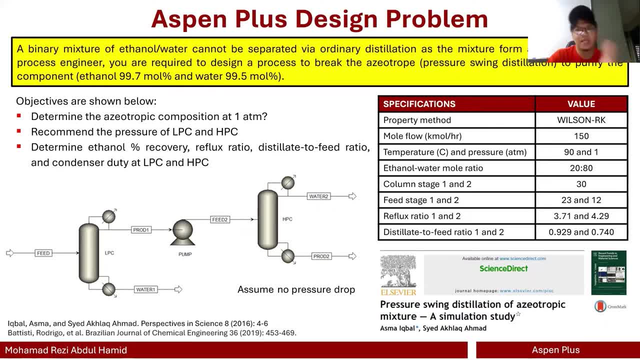 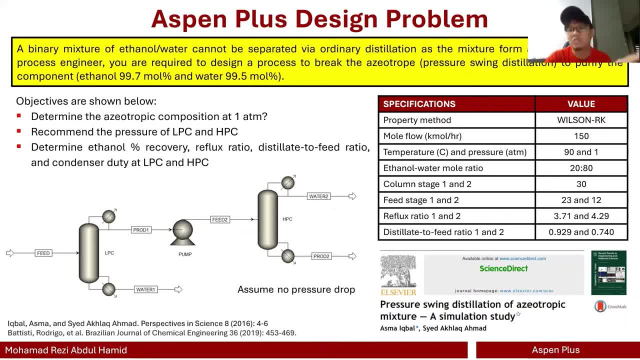 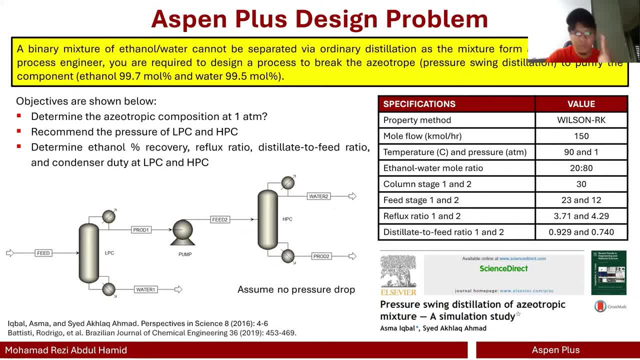 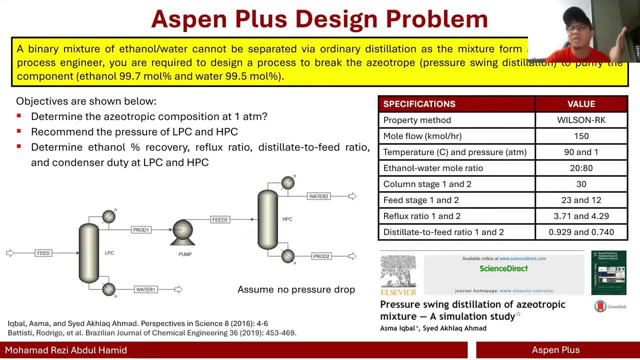 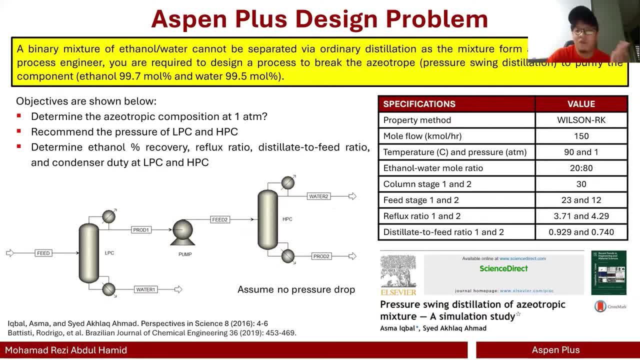 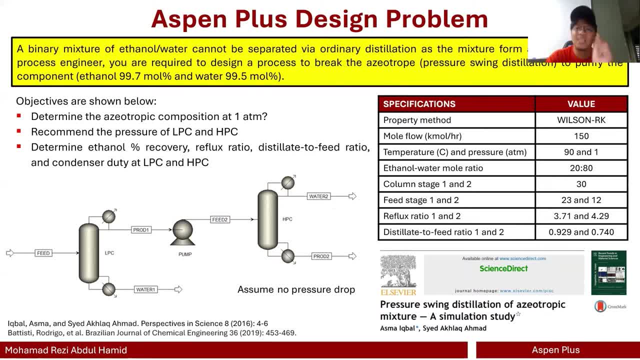 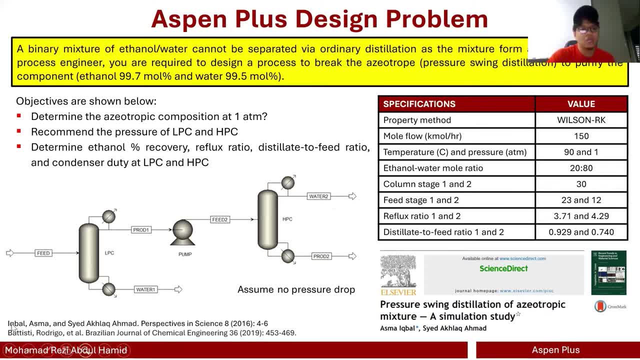 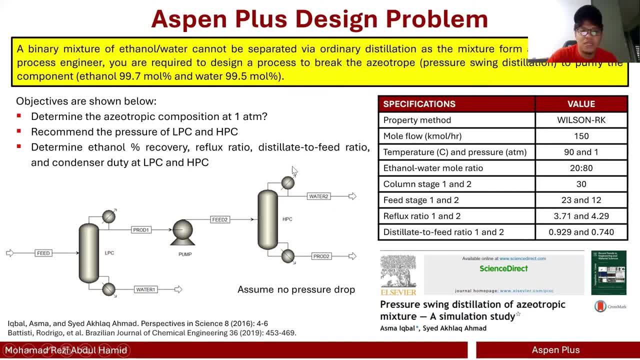 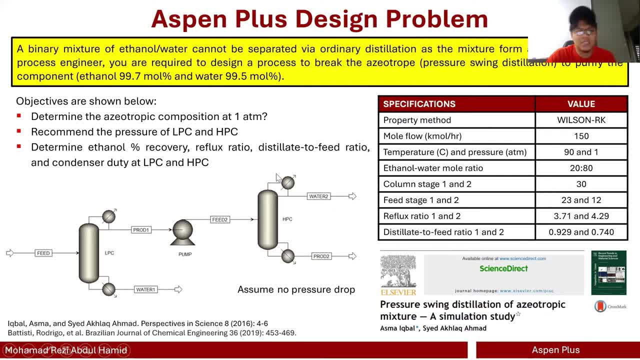 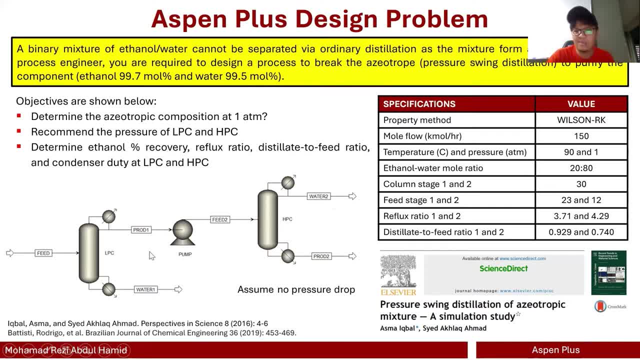 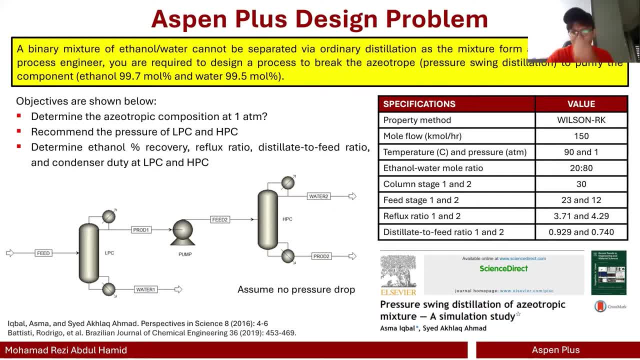 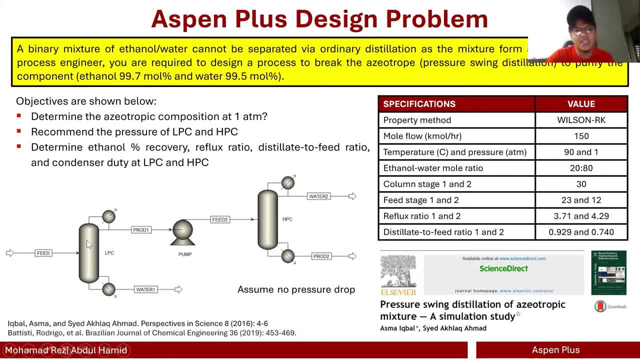 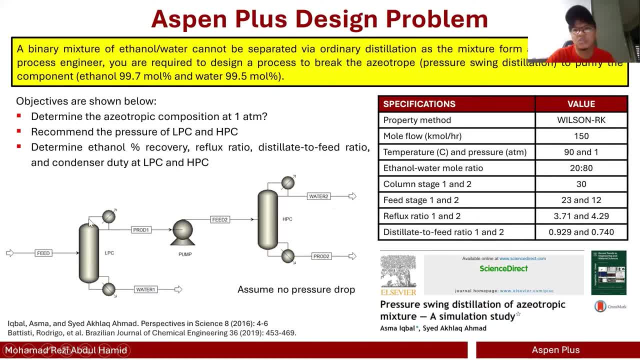 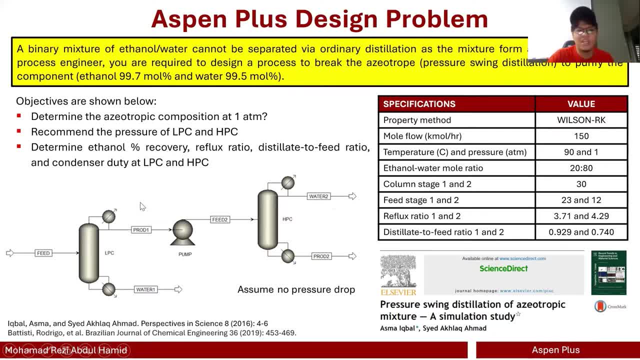 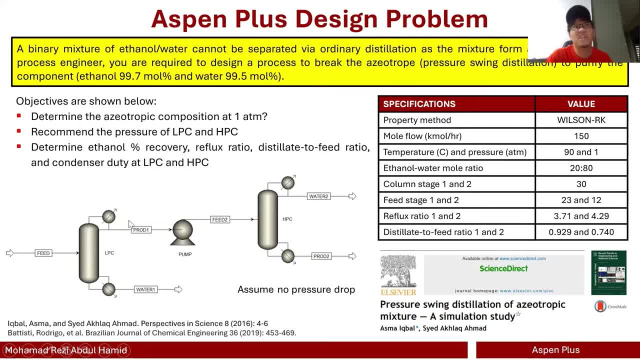 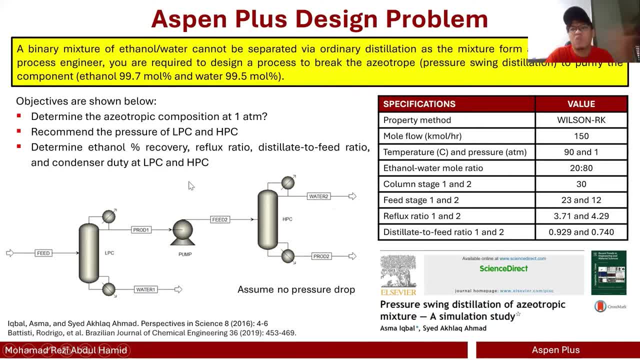 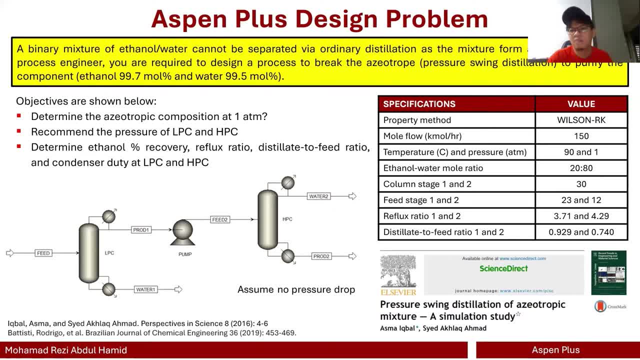 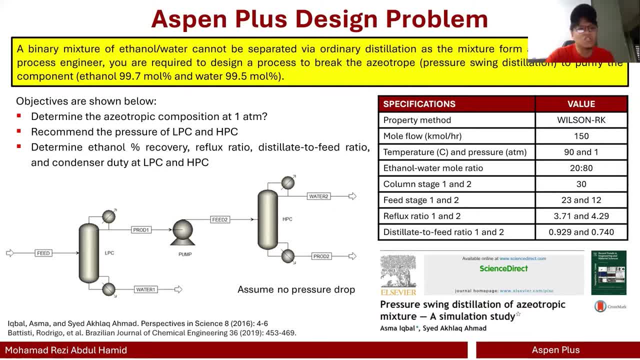 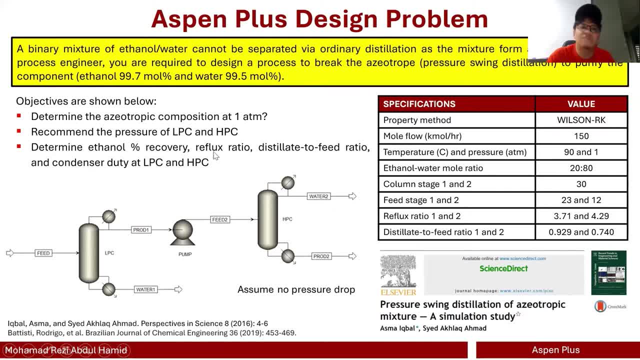 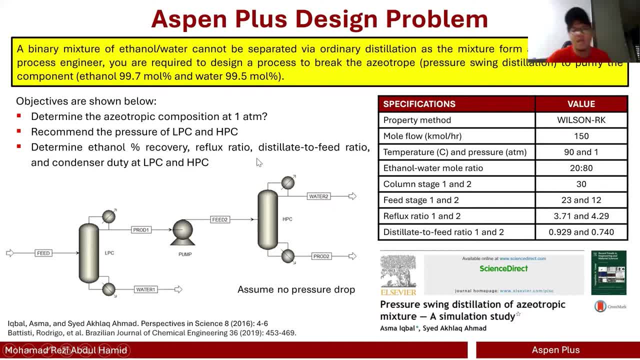 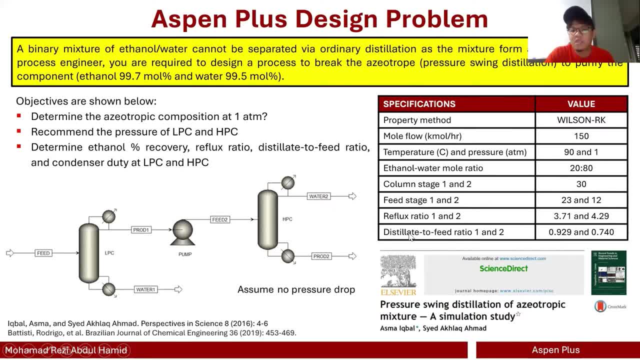 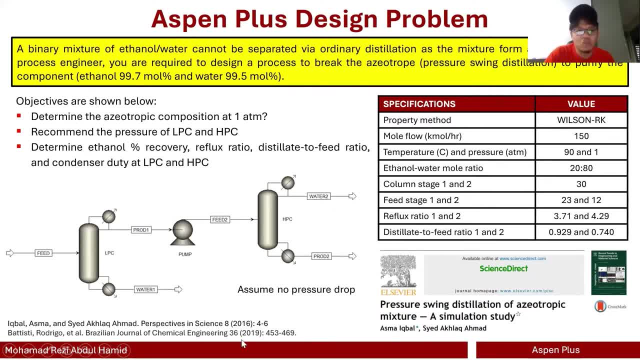 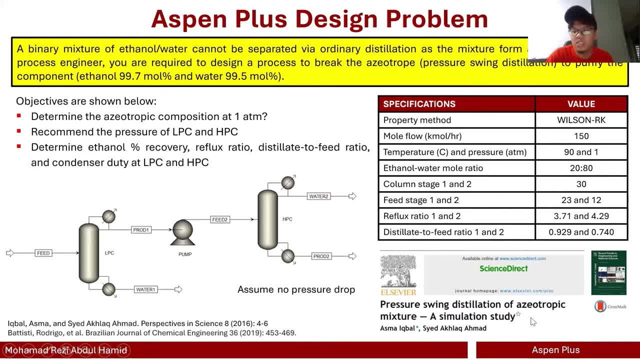 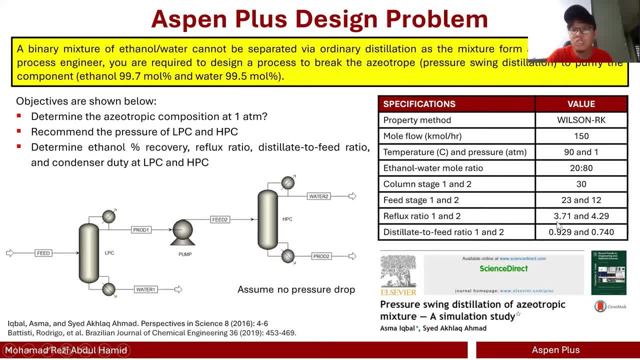 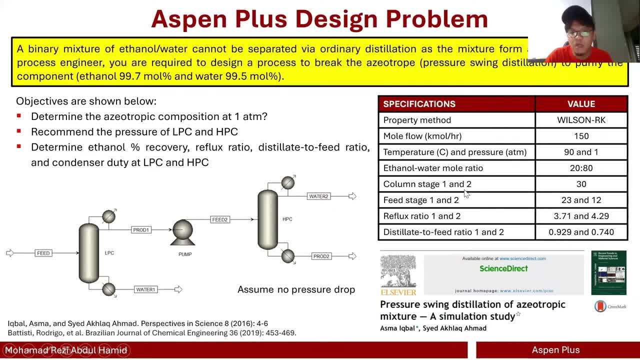 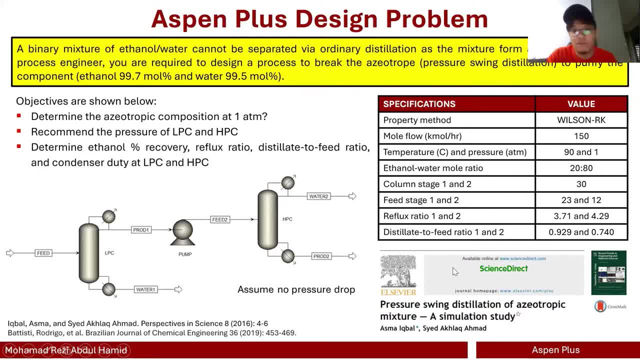 At this condition, the mixtures behave okay, even though we have two mixtures, two components, details. you can just have a look at this simulation specification and try to do it by own. That will be all for the design problem. Let's move on to our simulation. 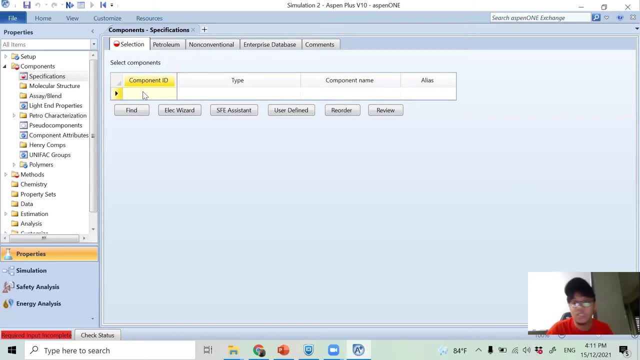 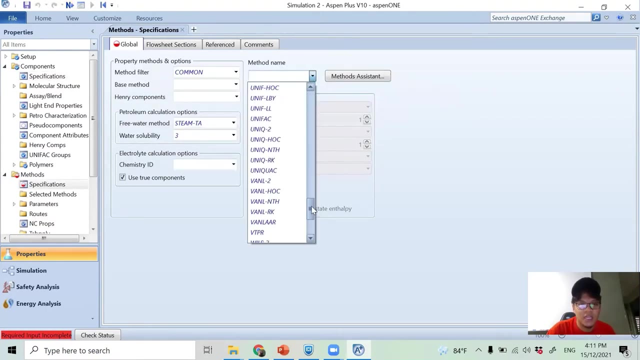 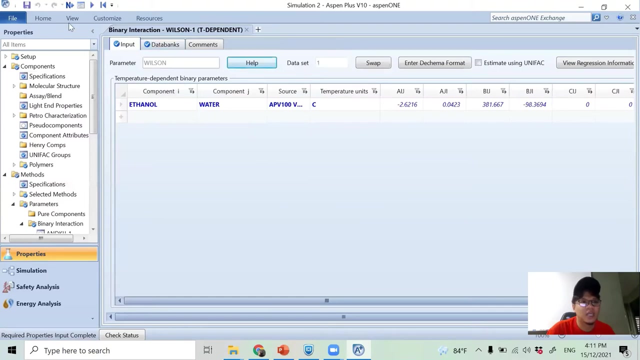 This is my AspenPlus graphical user interface. As usual, just input our component. Our component is ethanol- Enter and then water Enter And then hit next. We will be using Wilson RK- Let's see which is this one- And then I hit next, and then I hit next. 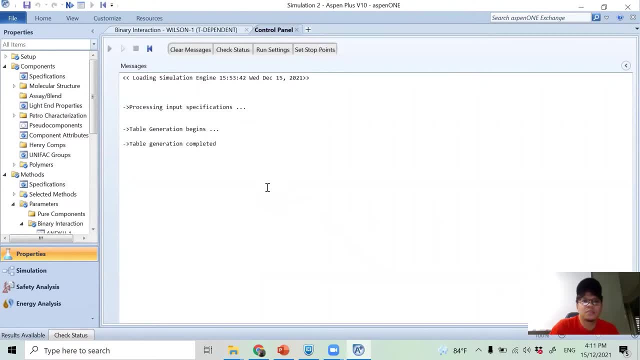 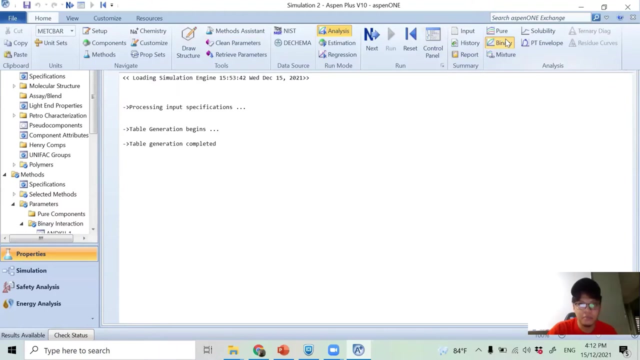 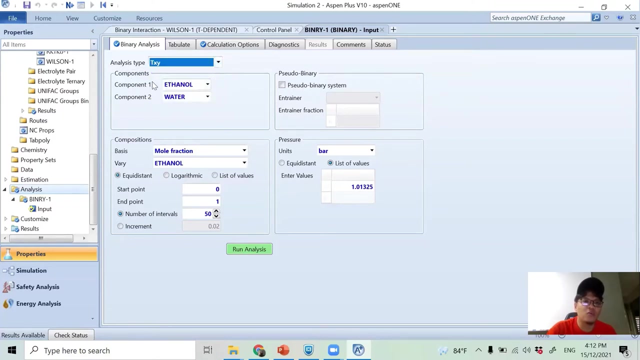 and then hit OK, Okay, next, If you remember our objective, our objective was to determine what is the azeotropic composition of ethanol-water mixture. So to do that, just go to home and then go to analysis, choose binary analysis and then choose TXY diagram. Component one should be ethanol. 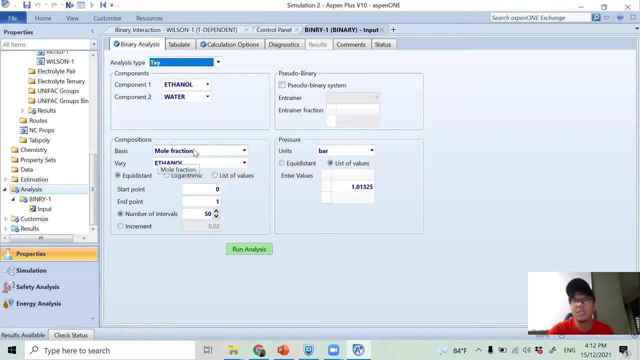 component two- water, and then more fraction. We're going to on the x-axis. you will see component one, component two- water and then more fraction. We're going to on the x-axis. you will have a more fraction, but we will use more fraction of ethanol. Basically, we will vary. 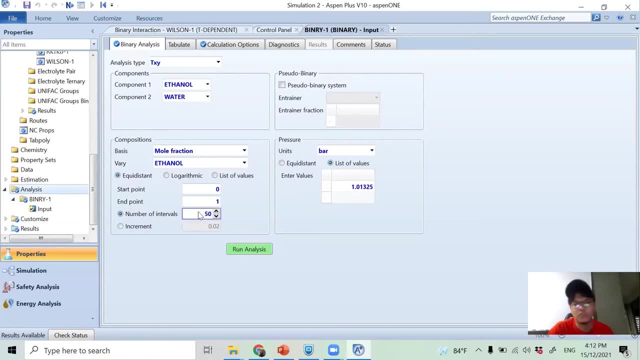 more fraction of ethanol from 0 to 1.. Maybe I will choose around 100 number of points At 1 ATM. actually this is already 1 ATM, but just want to use 1 ATM just to make sure that the numbers are not like a lot of significant figures of this. Okay, 1 ATM and then just run analysis. 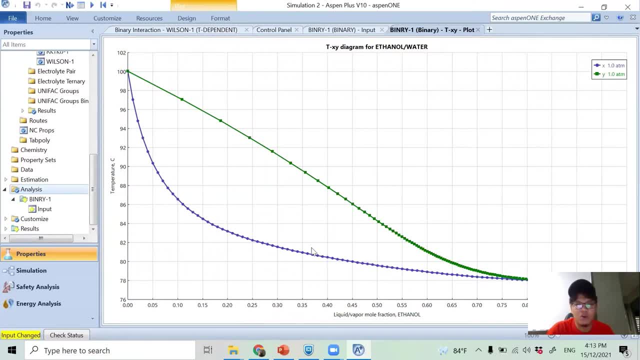 Okay, this is my TXY diagram of ethanol-water mixtures. Well, obviously, initially they have this liquid phase and vapor phase and co-existent phase, and then up to the point where I don't know. you don't see it behind the videos, but later I will show you the presentation. 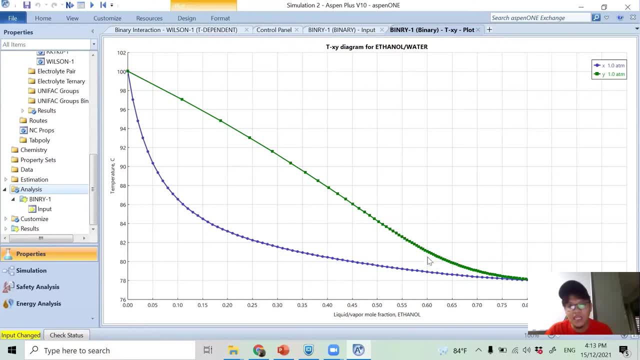 You will see that they merge these two lines, the green line and the blue line. they merge at one single point. at one single point around 0.86 dBT and the corresponding temperature is around 78. So that's our azeotropic mixture composition, in a sense. 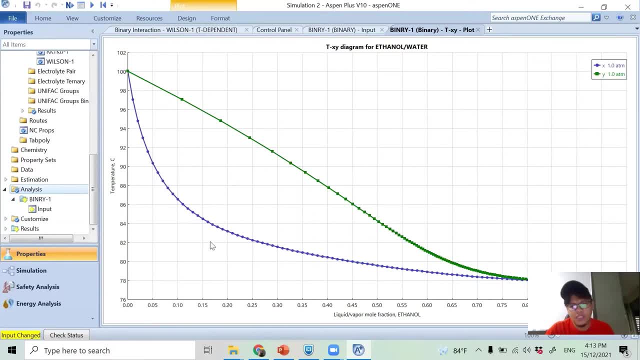 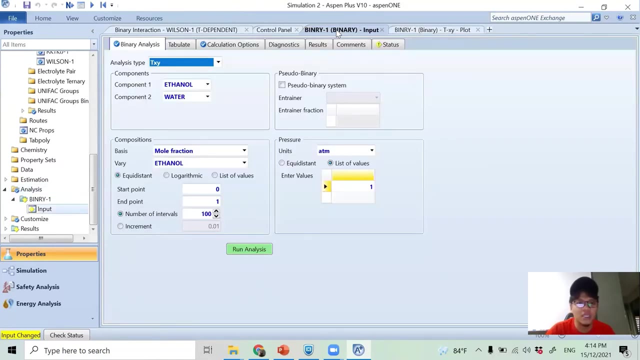 Now, well, obviously, this is quite a zoomed-out kind of graph, so what I'm going to do is I'm going to focus more on this region. Now, well, obviously, this is quite a zoomed-out kind of graph, so what I'm going to do is I'm going to focus more on this region. 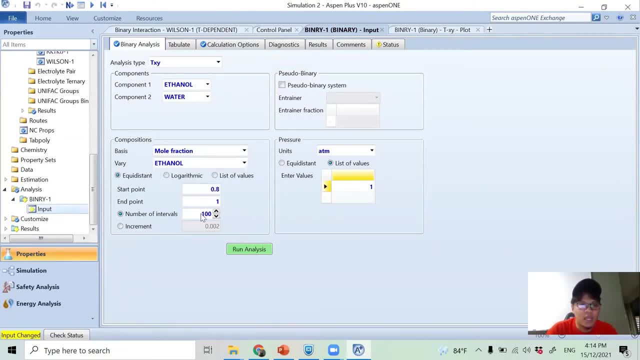 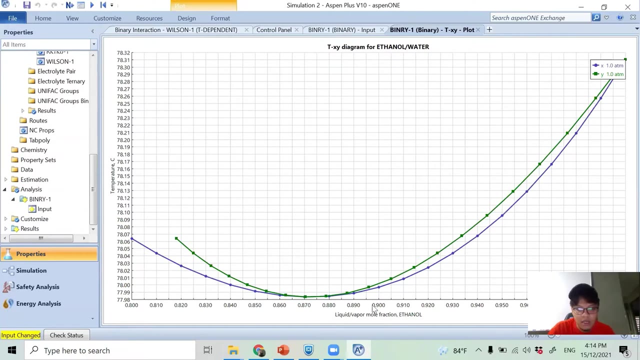 I will switch to 0.8 until 1, and then maybe have around 20 number of data points. I will switch to 0.8 until 1, and then maybe have around 20 number of data points. So, as you can see here, these are temperatures. Okay, these are the vapor. 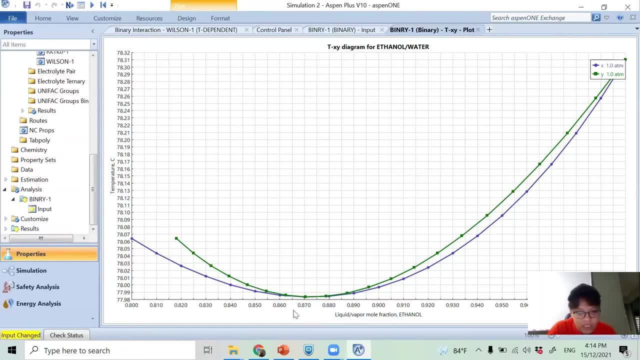 the mole fraction of ethanol. So, as you can see, the azeotropic is around 87 dBT. So, as you can see, the azeotropic is around 87 dBT. So, as you can see, the azeotropic is around 77 dBT. 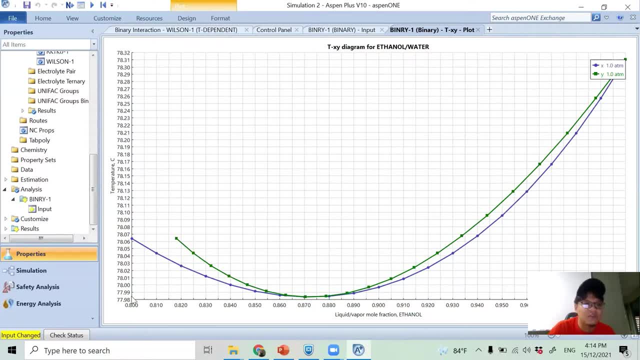 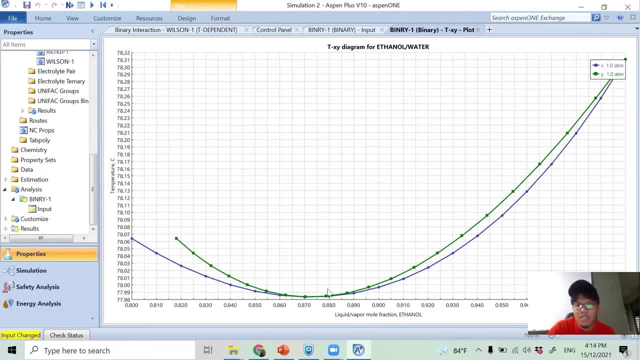 So, as you can see, the azeotropic is around 77 dBT. Okay, you have to remember that. Okay, you have to remember that. Okay, you have to remember that. Now, this is our azeotropic composition. 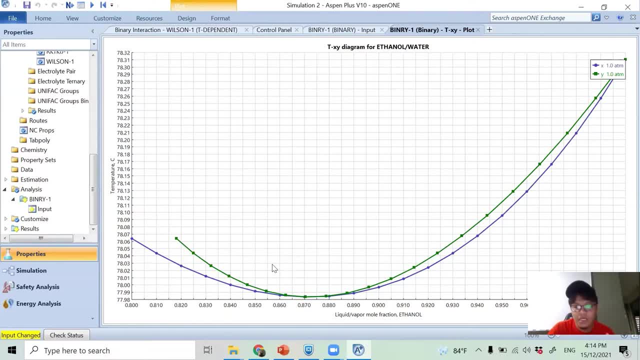 Now, this is our azeotropic composition. Now, this is our azeotropic composition. Okay, I'm gonna move on to the second. Okay, I'm gonna move on to the second. Okay, I'm gonna move on to the second, to the second objective, which is to find: 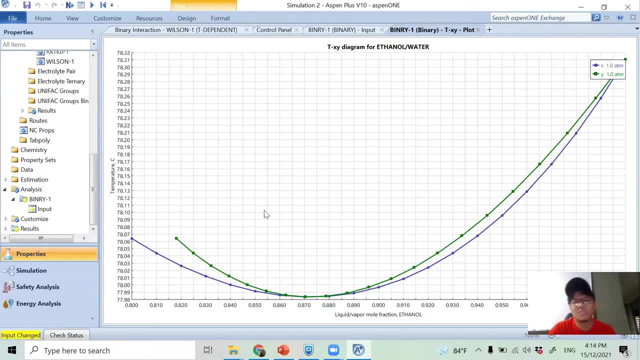 to the second objective, which is to find. to the second objective, which is to find, to recommend: what's the temperature to recommend? what's the temperature to recommend? what's the temperature or no? what's the pressure of our or no? what's the pressure of our? 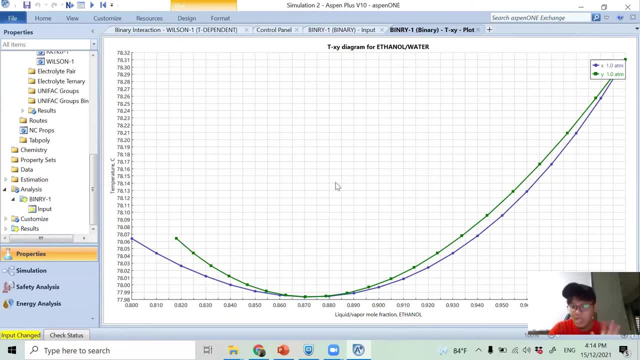 or no? what's the pressure of our high-pressure column? high-pressure column, high-pressure column. Don't worry, I will explain about this. Don't worry, I will explain about this. Don't worry, I will explain about this one later in the slide. 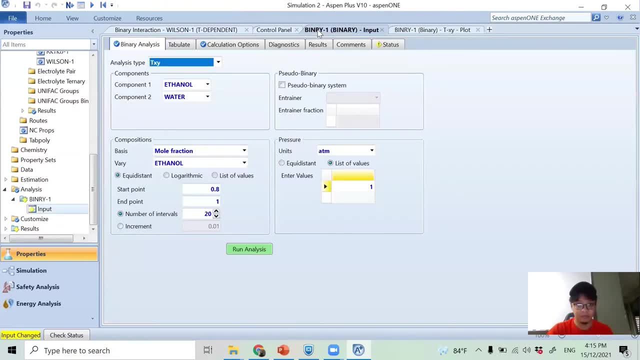 one later in the slide, one later in the slide. Just bear with me for a second. Just bear with me for a second, Just bear with me for a second. And now you just go back to this. And now you just go back to this. 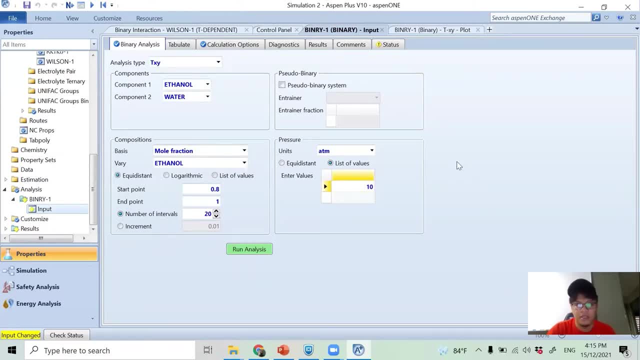 And now you just go back to this input form. You switch to 10. input form. You switch to 10. input form, You switch to 10. 10 bar, then ATM, and then run the 10 bar, then ATM, and then run the. 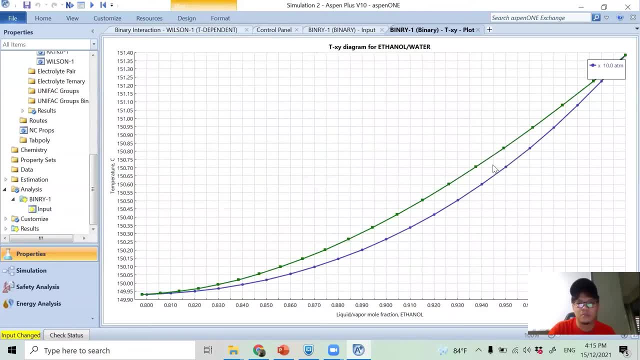 10 bar, then ATM and then run the analysis: Okay, 0.8 something here, right. Maybe. Okay, 0.8 something here, right, Maybe Okay, 0.8 something here, right. Maybe it's better for me if I 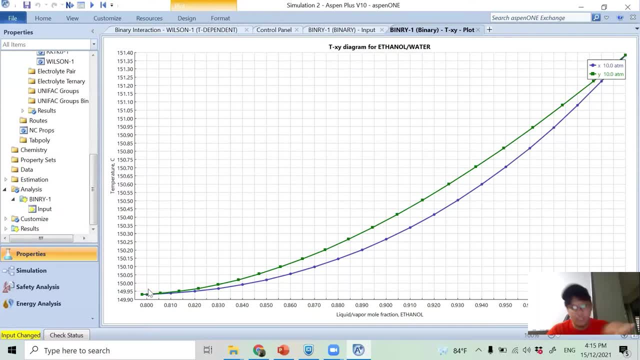 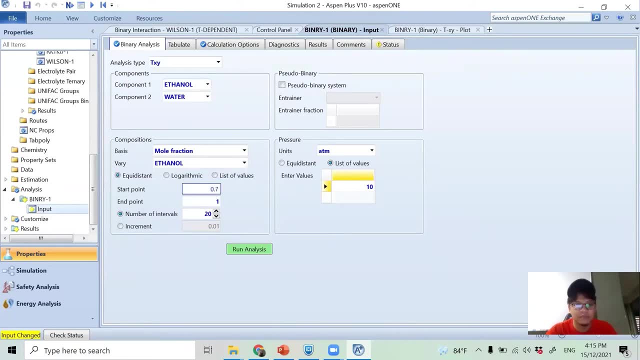 it's better for me if I, it's better for me if I choose a slightly lower value, so that, choose a slightly lower value, so that, choose a slightly lower value so that you can see the curve. you can see the curve. I'll switch it to 0.7, I guess. 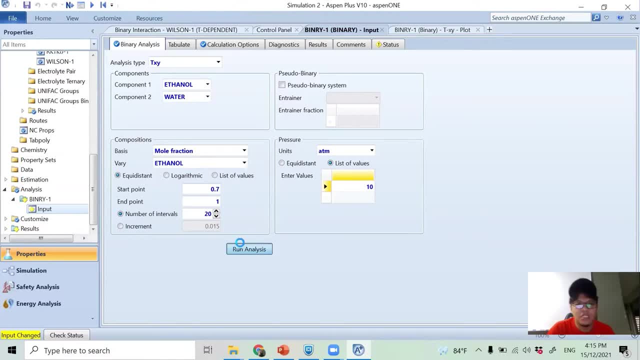 I'll switch it to 0.7. I guess I'll switch it to 0.7. I guess Maybe it's a lot better that way. Maybe it's a lot better that way. Maybe it's a lot better that way. Run analysis. 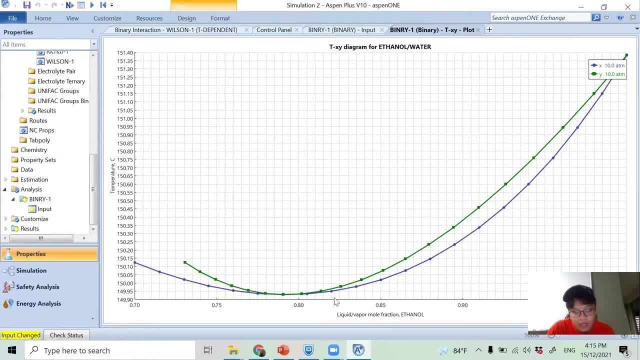 Run analysis. Run analysis. give a second Now, as you can see. give a second Now, as you can see. give a second Now, as you can see. the, the, the in the one atmosphere condition, the in the one atmosphere condition, the. 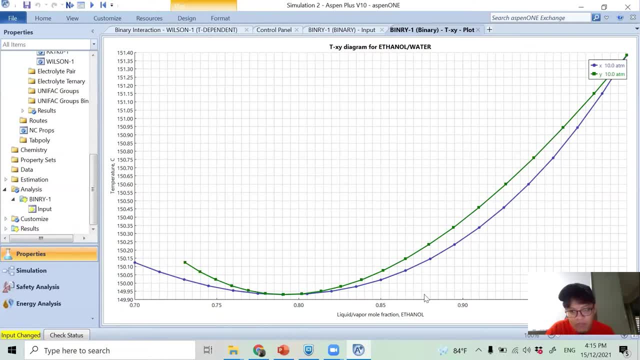 in the one atmosphere condition the azeotrope was around here. 0.87,. maybe azeotrope was around here. 0.87,. maybe azeotrope was around here. 0.87, maybe here. 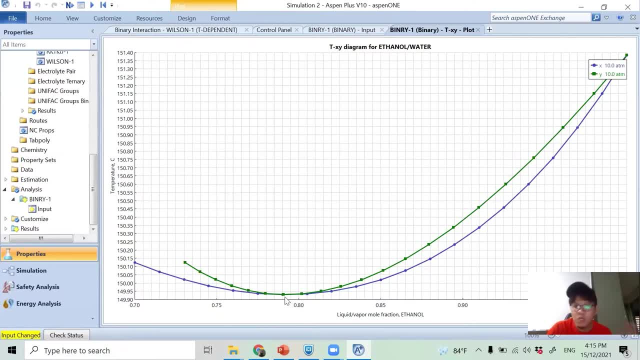 here, here, But then at high pressure, the azeotrope. But then at high pressure, the azeotrope, But then, at high pressure, the azeotrope shifted to a lower value which is shifted to a lower value which is. 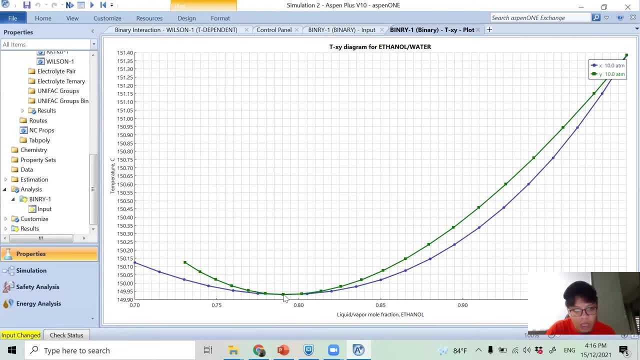 shifted to a lower value, which is around, around, around around 0.79,- okay, which, and then the 0.79, okay, which, and then the 0.79,- okay which, and then the temperature is around 150 degrees Celsius. 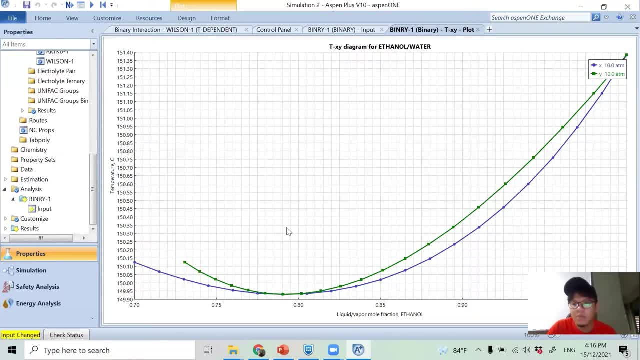 temperature is around 150 degrees Celsius. temperature is around 150 degrees Celsius. Okay, I'm not going to explain the. Okay, I'm not going to explain the. Okay, I'm not going to explain the result here, result here, result here. but I will explain the result in the. 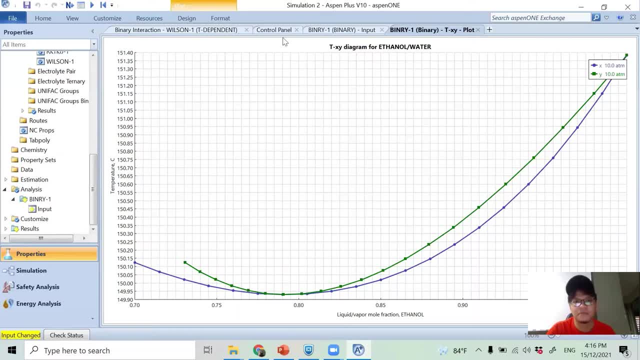 but I will explain the result in the, but I will explain the result in the presentation. So let's go back to our presentation presentation. So, as you can see here, this is the TXY presentation. So, as you can see here, this is the TXY. 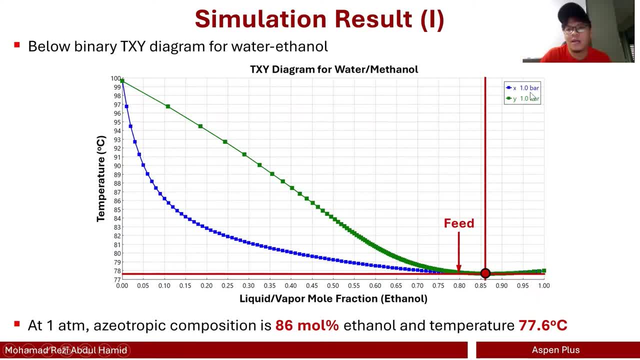 presentation. So, as you can see here, this is the TXY diagram for water and methanol at one. diagram for water and methanol at one. diagram for water and methanol at one. in this case, one bar of pressure. in this case, one bar of pressure. 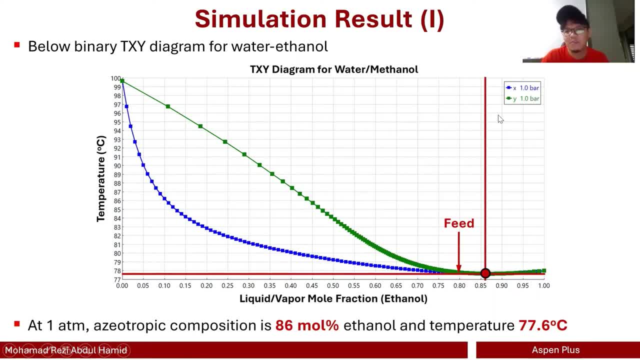 in this case, one bar of pressure. It doesn't really matter, it's fine. So It doesn't really matter, it's fine. So It doesn't really matter, it's fine. So one bar, one atm. The curve is more. 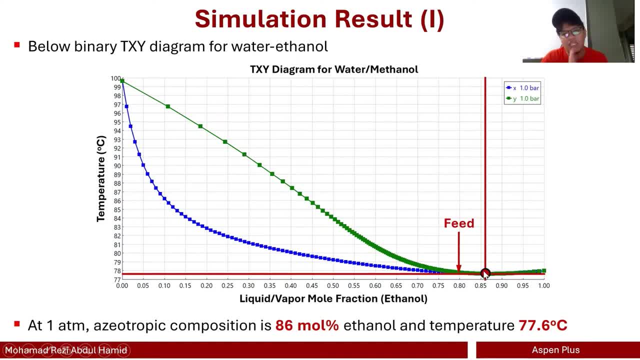 one bar, one atm, The curve is more. one bar, one atm, The curve is more or less the same, or less the same, or less the same, And then maybe the point is slightly, And then maybe the point is slightly, And then maybe the point is slightly shifted a bit. but one bar, one atm. 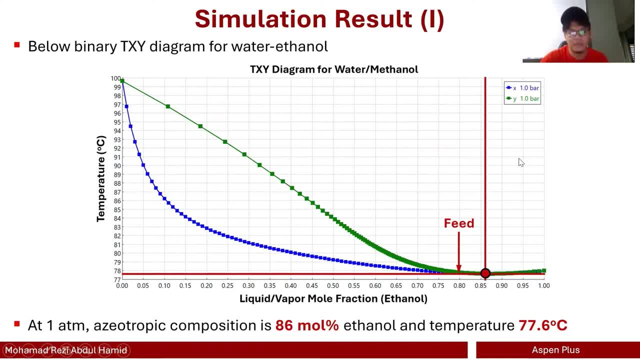 shifted a bit, but one bar, one atm- shifted a bit, but one bar, one atm. I think it's not going to make too much. I think it's not going to make too much. I think it's not going to make too much of a significant difference. 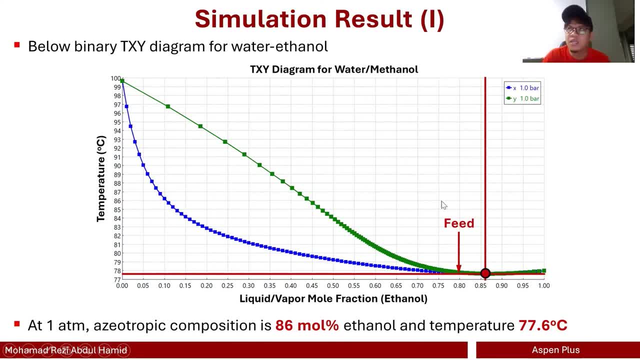 of a significant difference, of a significant difference. So you have to understand here our. So you have to understand here our. So you have to understand here our feed, which is the ethanol water feed, which is the ethanol water feed, which is the ethanol water mixture is around 80 to 20. 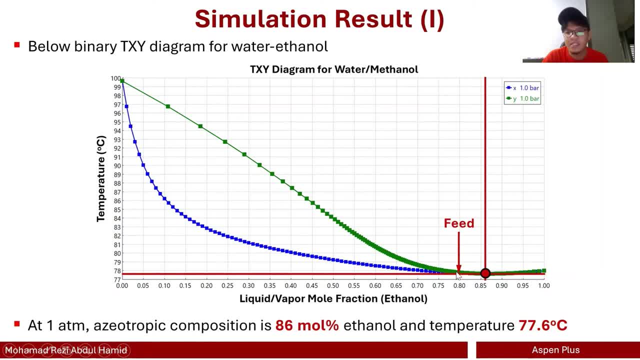 mixture is around 80 to 20. mixture is around 80 to 20 mole percent, So our feed goes here. mole percent, So our feed goes here. mole percent, So our feed goes here. and, as I said, if it's. 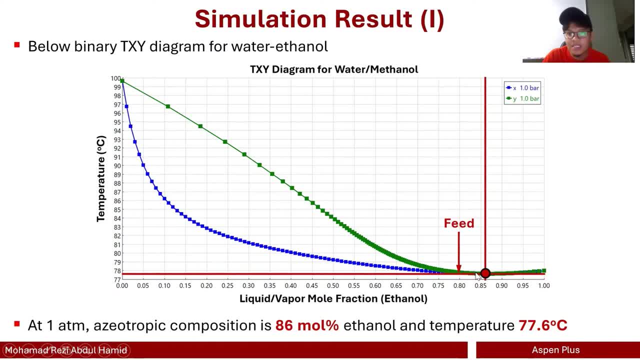 and, as I said, if it's, and as I said, if it's, go here and the isotope is around 86,, go here and the isotope is around 86,, go here and the isotope is around 86,. you cannot do further enrichment beyond. 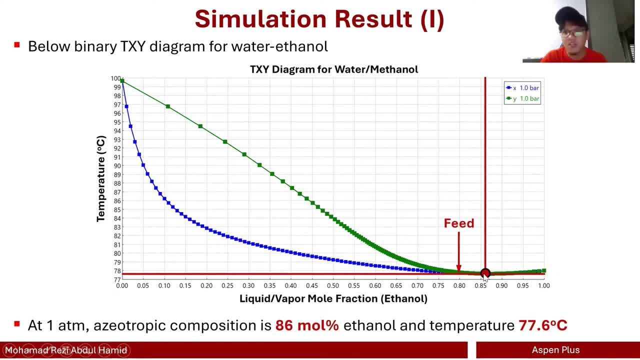 you cannot do further enrichment beyond. you cannot do further enrichment beyond 86.. 86.. 86.. More percent of ethanol, More percent of ethanol, More percent of ethanol. which is the reason why, which is the reason why, which is the reason why we do pressure swing distillation at 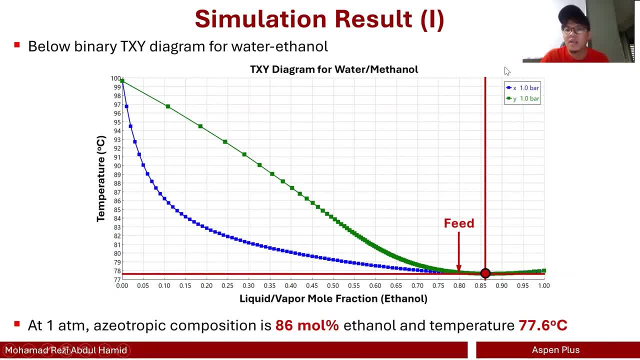 we do pressure swing distillation at. we do pressure swing distillation at one pressure At one pressure, one pressure At one pressure At one pressure At one one pressure At one pressure, At one value of pressure. okay, which is at. 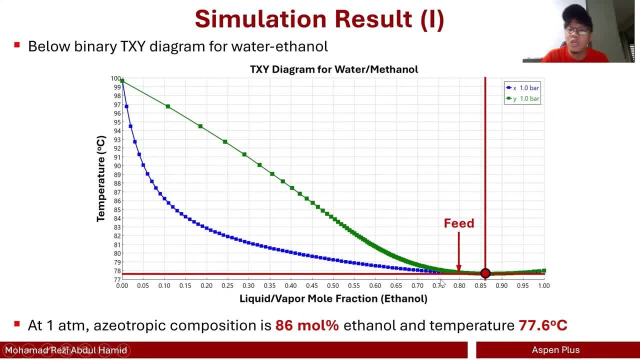 value of pressure. okay, which is at value of pressure. okay, which is at one bar condition. if you use one column, one bar condition. if you use one column, one bar condition. if you use one column, you cannot do any further. enrichment: 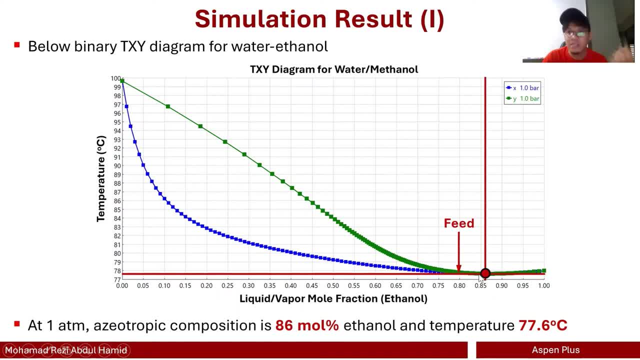 you cannot do any further enrichment, you cannot do any further enrichment between 86%, because that's the limit between 86%, because that's the limit between 86%, because that's the limit. Now in here, we have determined that. Now in here, we have determined that. 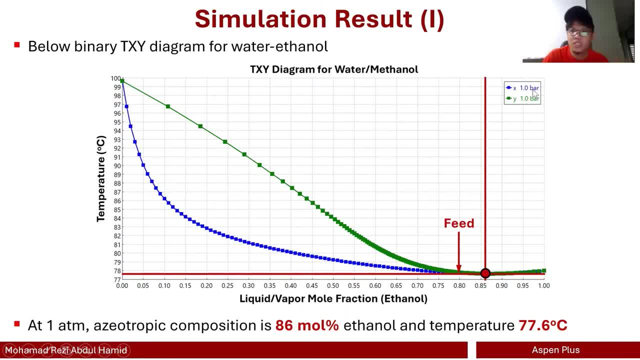 Now in here we have determined that at one bar pressure or one atmosphere, at one bar pressure or one atmosphere, at one bar pressure or one atmosphere, pressure, pressure, pressure, you will have, you will have, you will have isotropic composition around 86%. 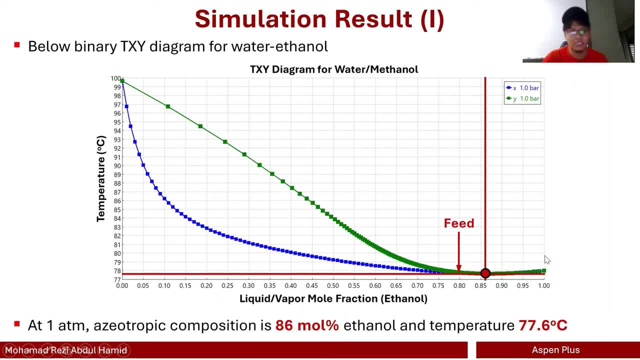 isotropic composition around 86%. isotropic composition around 86%. and temperature around 77.6 degrees and temperature around 77.6 degrees and temperature around 77.6 degrees Celsius. Now if you see, if you remember, Celsius. Now if you see, if you remember. 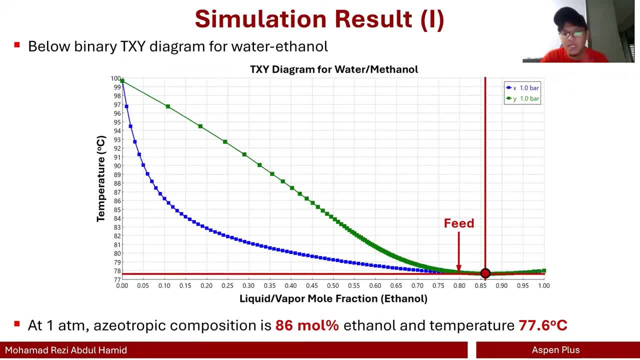 Celsius. Now, if you see, if you remember what I did, I do I zoom in into this what I did, I do, I zoom in into this what I did, I do, I zoom in into this particular region and I analyze. 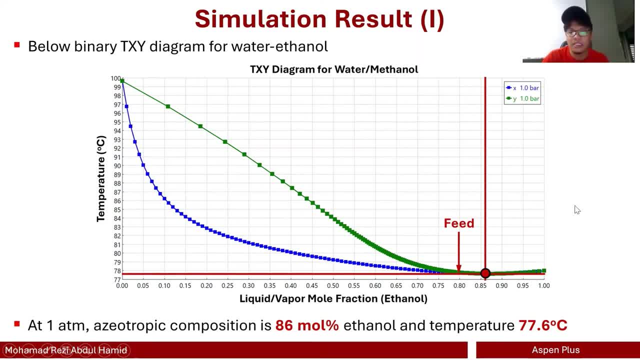 particular region and I analyze particular region and I analyze the values in more details, the values in more details, the values in more details. So these are the values. So these are the values. So these are the values. these are the values for TXY diagram for. 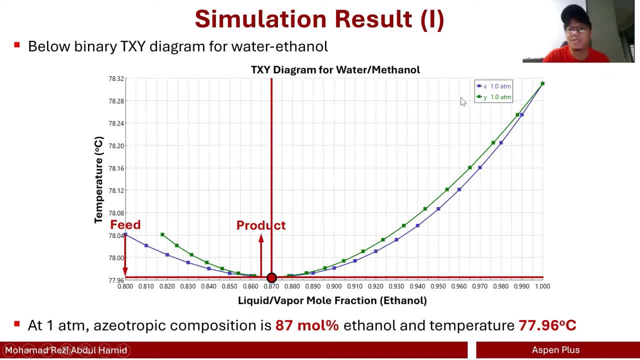 these are the values for TXY diagram. for. these are the values for TXY diagram for water-methanol mixtures at 1 atm. water-methanol mixtures at 1 atm. water-methanol mixtures at 1 atm. The previous one is 1 bar, this one 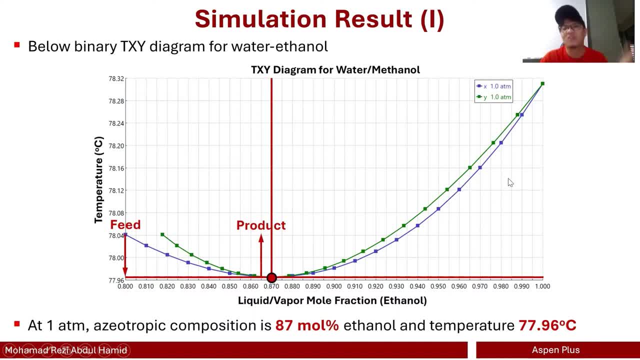 The previous one is 1 bar, this one. The previous one is 1 bar, this one is 1 atm. I think actually I do it is 1 atm. I think actually I do it is 1 atm. I think actually I do it two times, but I forgot to switch. 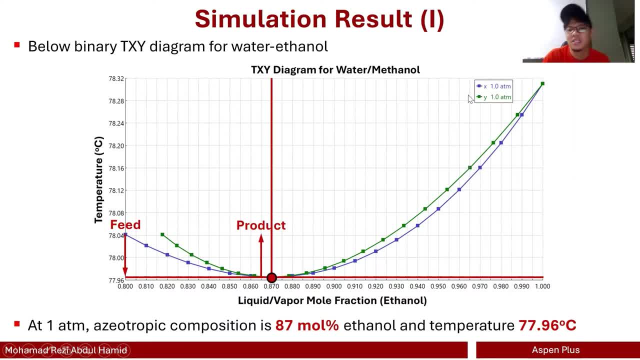 two times. but I forgot to switch two times. but I forgot to switch the values: the pressure actually, the values, the pressure actually, the values, the pressure actually. But, as I said, 1 bar 1 atm. But as I said, 1 bar 1 atm. 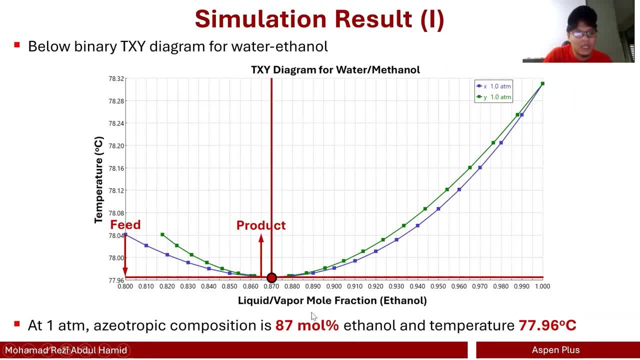 But, as I said, 1 bar, 1 atm doesn't really matter. I guess doesn't really matter, I guess doesn't really matter. I guess Now, at this one again, Now at this one again. 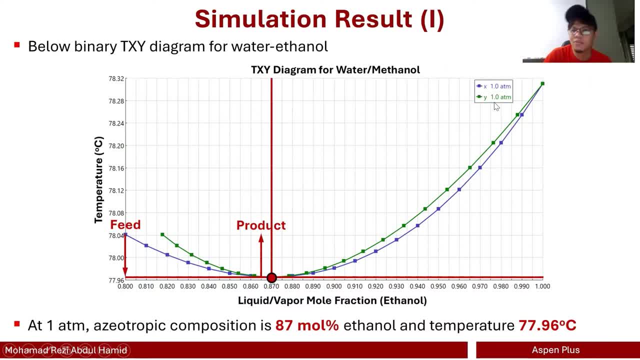 Now at this one again: isotopy is about 87,. maybe this one isotopy is about 87,. maybe this one isotopy is about 87,. maybe this one is 1 atm, so the data set is 1 atm. so the data set. 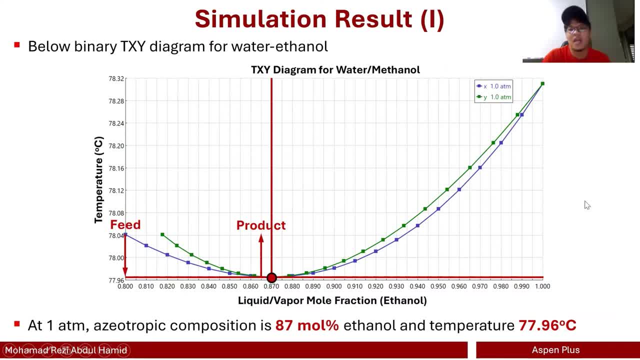 is 1 atm. so the data set changed and the temperature is 77.96.. changed and the temperature is 77.96.. changed and the temperature is 77.96.. Now, as I said before, if you are relying, Now, as I said before, if you are relying, 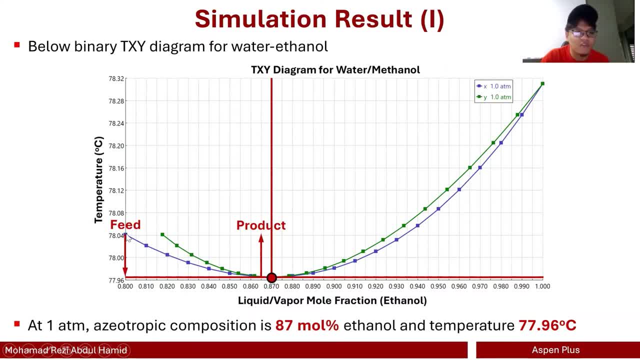 Now, as I said before, if you are relying on one distillation column, and you are on one distillation column, and you are on one distillation column and you are feeding your component at 80, feeding your component at 80, feeding your component at 80 weight percent, 80 more percent of 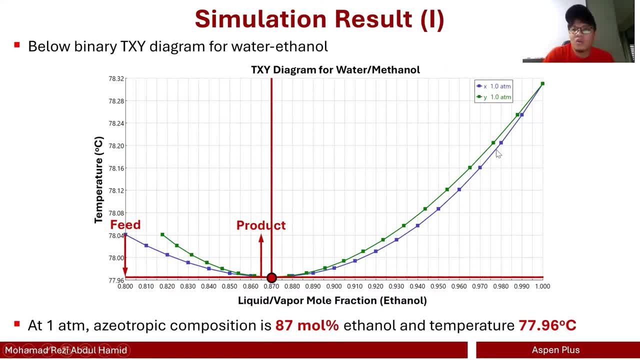 weight percent, 80 more percent of weight percent, 80 more percent of ethanol, ethanol, ethanol. if you're just focusing on, if you're just, if you're just focusing on, if you're just, if you're just focusing on, if you're just relying on one distillation column at relying on one distillation column, at relying on one distillation column, at most you will get around 87 percent. most you will get around 87 percent. most you will get around 87 percent. more percent of ethanol enrichment. 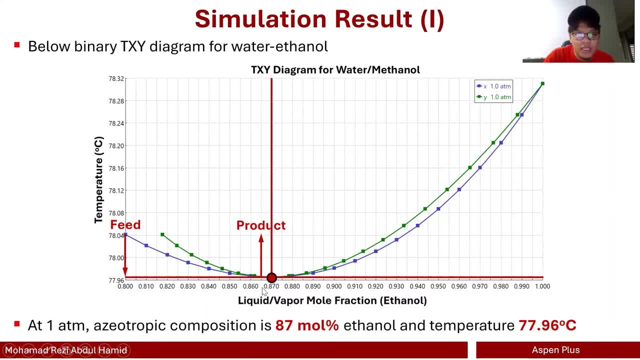 more percent of ethanol enrichment, more percent of ethanol enrichment, But in this case, maybe I will target, But in this case, maybe I will target, But in this case, maybe I will target around 80,, around 80,, around 80,, 86, or, in this case, 86.5. 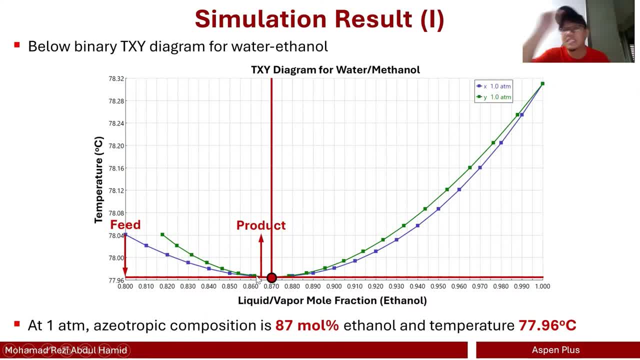 86, or, in this case, 86.5, 86, or, in this case, 86.5 more percent of the product, leaving my more percent of the product, leaving my more percent of the product, leaving my first distillation column. first distillation column. 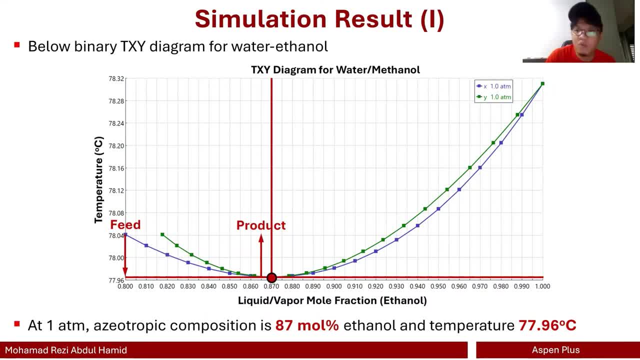 first distillation column: Okay, that's the. that's basically the Okay, that's the. that's basically the Okay, that's the. that's basically the objective number one. we determine what objective number one. we determine what objective number one. we determine what is the composition or azeotropic. 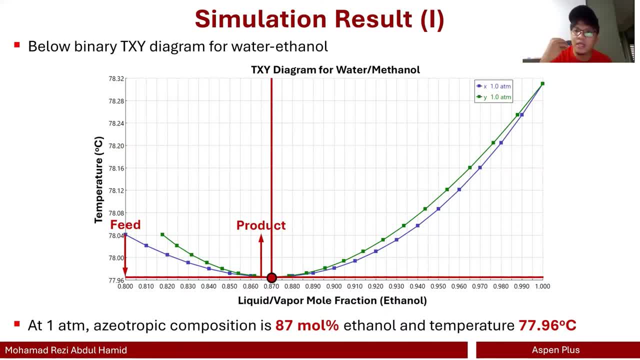 is the composition or azeotropic? is the composition or azeotropic composition at one composition? at one composition at one uh one- uh 180 and pressure- uh one- uh 180 and pressure- uh one uh 180 and pressure. The second objective was: 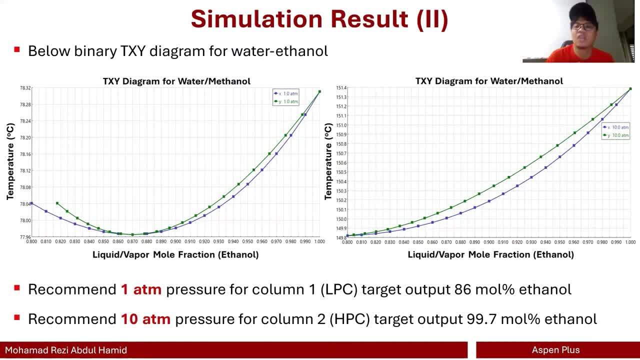 The second objective was: The second objective was to recommend what is the temperature to recommend. what is the temperature to recommend, what is the temperature and what's now what's the pressure of, and what's now what's the pressure of and what's now what's the pressure of our azeotrope of what is the pressure of? 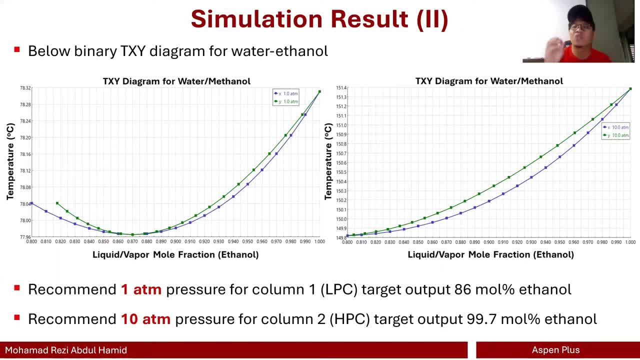 our azeotrope of what is the pressure of our azeotrope of what is the pressure of our second column, so that we uh in order our second column, so that we uh in order our second column, so that we uh in order to break this azeotrope for further. 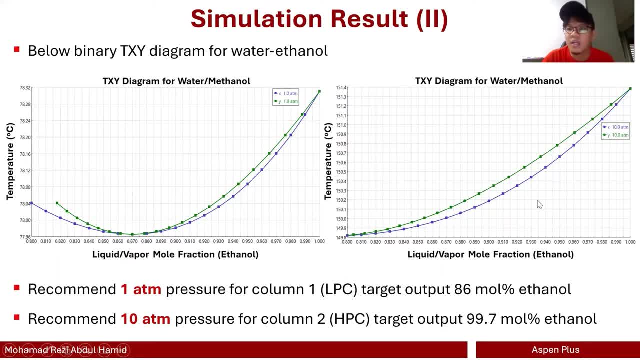 to break this azeotrope for further, to break this azeotrope for further: enrichment, enrichment, enrichment. all the way to 99.7 or more percent. so all the way to 99.7 or more percent. so all the way to 99.7 or more percent. so, as you can see here, this is the txy. 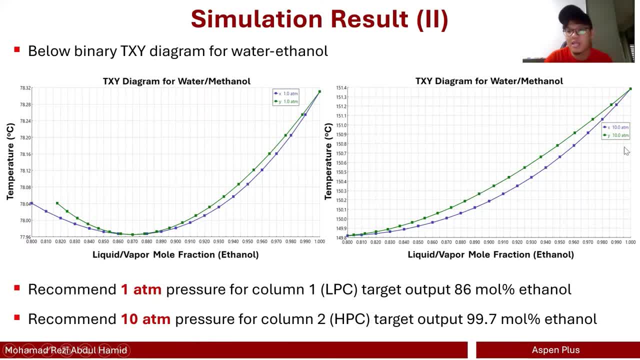 as you can see here, this is the txy. as you can see here, this is the txy diagram at one atmosphere pressure and diagram at one atmosphere pressure and diagram at one atmosphere pressure. and one on the right hand side is the txy, one on the right hand side is the txy. 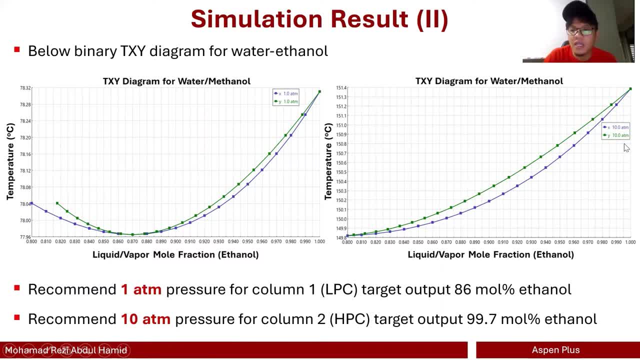 one on the right hand side is the txy diagram at diagram at diagram at um, um, um, 10 atmosphere pressure and it's and if you 10 atmosphere pressure and it's, and if you 10 atmosphere pressure and it's and if you see see, 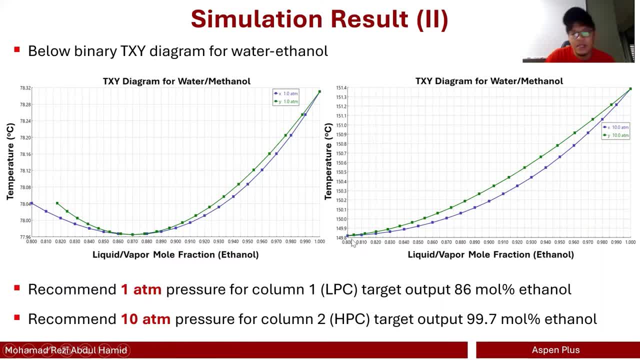 see the azeotrope here is 87 and the azeotrope here is 87 and the azeotrope here is 87 and in in the high pressure condition, the. in in the high pressure condition, the. in in the high pressure condition, the azeotrope is 1.8. 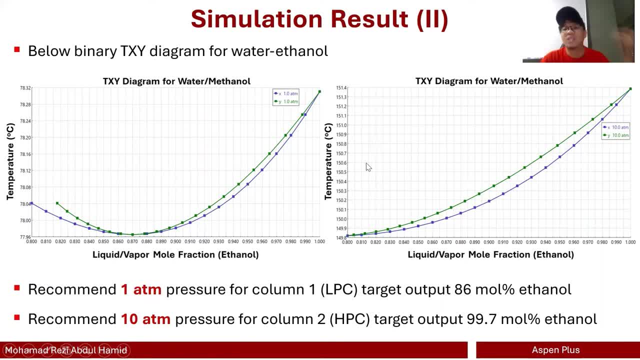 azeotrope is 1.8. azeotrope is 1.8. so what i will do is so, what i will do is so. what i will do is to allow for the enrichment. what i will to allow for the enrichment, what i will do is. 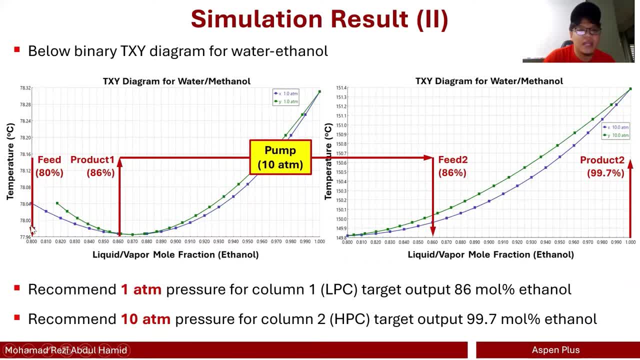 do is do is. i will do like this. my feed enters it. i will do like this. my feed enters it. i will do like this. my feed enters it: at the first column, at one atmosphere, at the first column, at one atmosphere, at the first column, at one atmosphere, operating at one atmospheres. 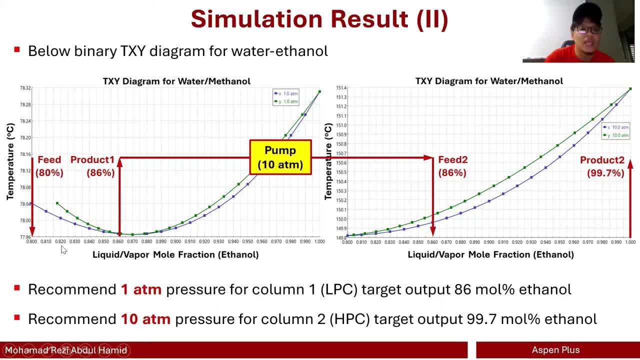 operating at one atmospheres. operating at one atmospheres, the feed is 80 percent. more percent of the feed is 80 percent, more percent of the feed is 80 percent, more percent of ethanol, and then i will do enrichment- ethanol, and then i will do enrichment. 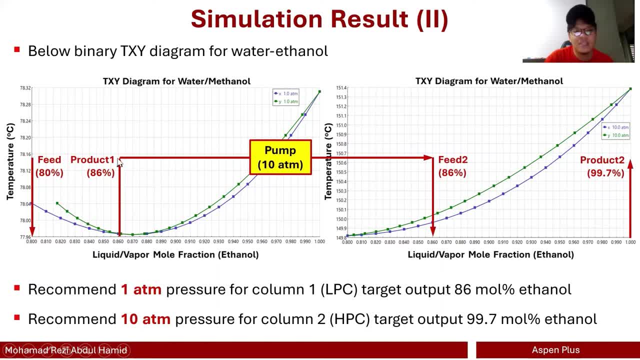 ethanol, and then i will do enrichment all the way to 86 percent, all the way to 86 percent, all the way to 86 percent, and then i will send the same component, and then i will send the same component, and then i will send the same component. okay, i don't do any, any enrichment, and 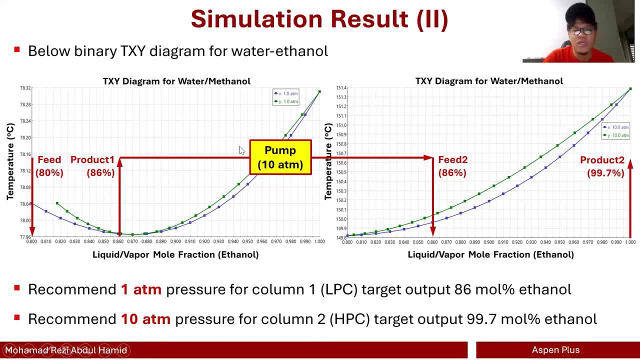 okay, i don't do any any enrichment. and okay, i don't do any any enrichment and send it to pump, send it to pump, send it to pump and will increase the pressure to 10 and will increase the pressure to 10 and will increase the pressure to 10. atmospheric pressure and in this case, 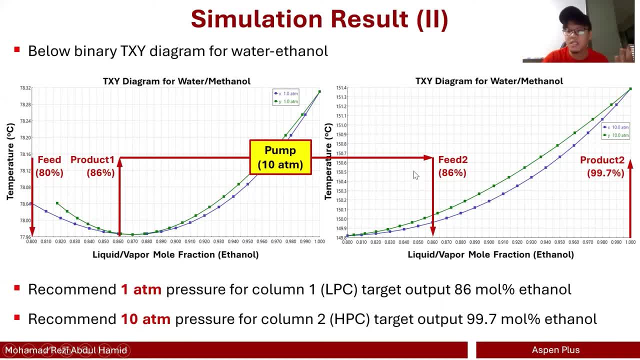 atmospheric pressure and in this case, atmospheric pressure, and in this case they are still 86 percent. they are still 86 percent. they are still 86 percent. more percent purity of ethanol, more percent purity of ethanol, more percent purity of ethanol. and in here and in here, 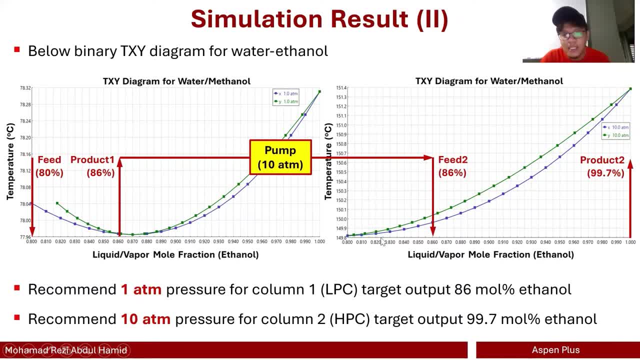 and in here it will enter high pressure column and it will enter high pressure column and it will enter high pressure column. and in this case, in this case, in this case, the azotope is in here, i am no longer at. the azotope is in here, i am no longer at. 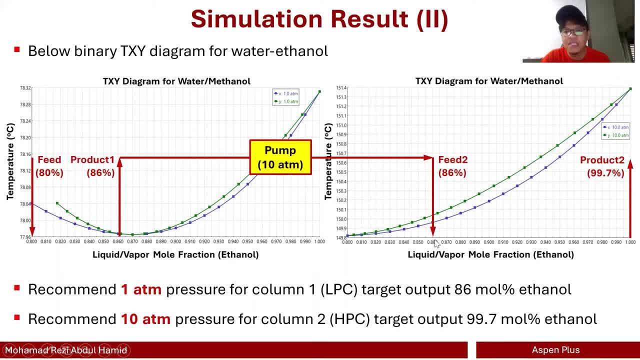 the azotope is in here. i am no longer at the azotropic point, so i can do for the. the azotope is in here. i am no longer at the azotropic point, so i can do for the enrichment from 86 all the way to 99.7. 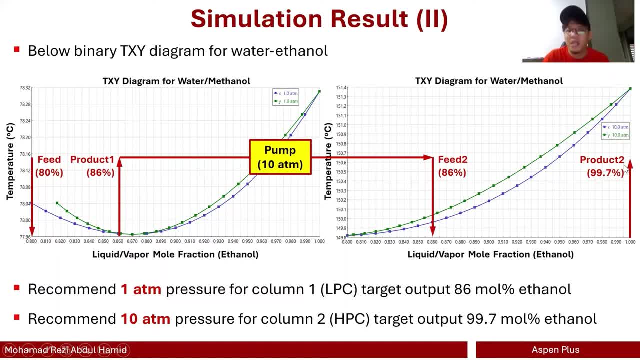 enrichment from 86 all the way to 99.7. enrichment from 86 all the way to 99.7. percent of percent of percent of uh purity that i want. so in this case, i uh purity that i want. so in this case, i uh purity that i want. so in this case, i am recommending one atmosphere pressure. 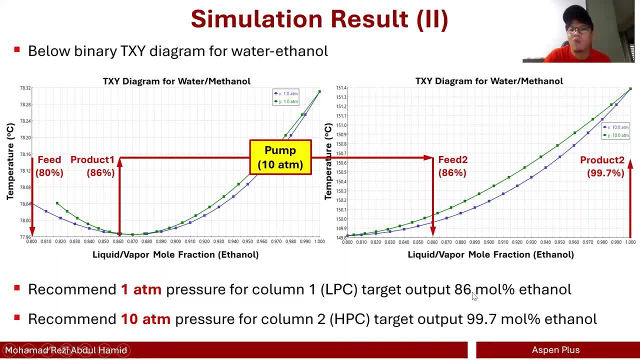 am recommending one atmosphere pressure, am recommending one atmosphere pressure for column number one, which is low. for column number one which is low. for column number one, which is low. pressure column and target output which pressure column and target output which pressure column? and target output which is the distillate part. 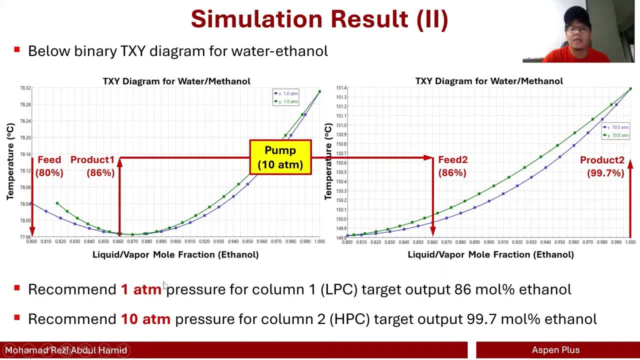 is the distillate part. is the distillate part around 86 more percent of ethanol and around 86 more percent of ethanol and around 86 more percent of ethanol, and then the distillate part will enter, will be sent to pump and then they will. 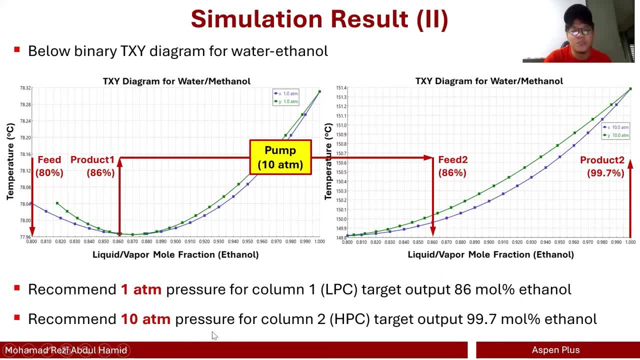 will be sent to pump and then they will will be sent to pump and then they will enter the high pressure column operating. enter the high pressure column operating. enter the high pressure column operating at 10 atmosphere pressure. at 10 atmosphere pressure, at 10 atmosphere pressure and the target output: uh 99.7 more. 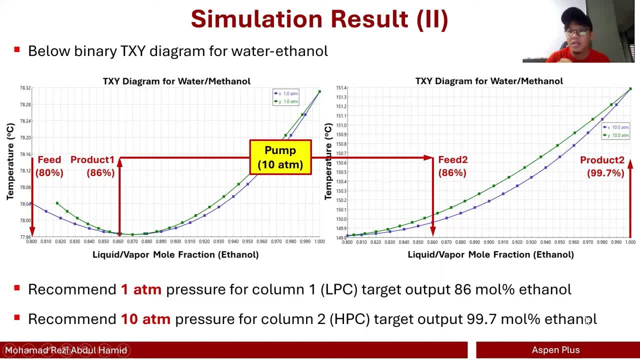 and the target output uh 99.7 more and the target output uh 99.7 more percent of ethanol at the bottom percent of ethanol at the bottom percent of ethanol at the bottom section of the part of the of the column section of the part of the of the column. 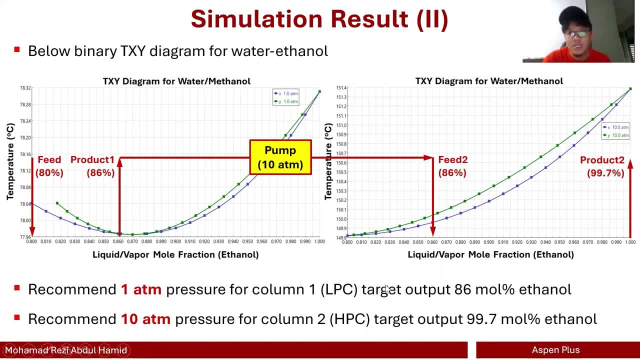 section of the part of the of the column, not at the distillate part. the reason is not at the distillate part. the reason is not at the distillate part. the reason is because, because, because, as you see here, uh, at this point, as you see here, uh, at this point, 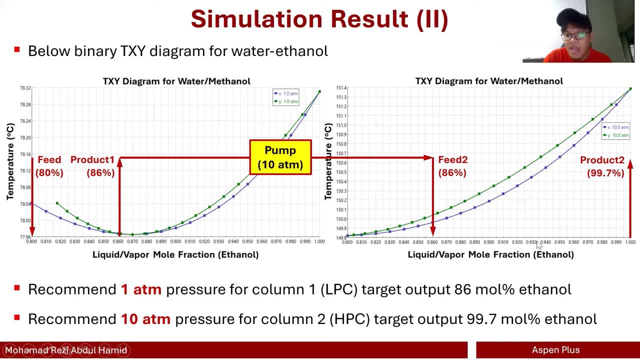 as you see here. uh, at this point it is 150 degrees celsius, but at the it is 150 degrees celsius, but at the it is 150 degrees celsius, but at the higher purity of ethanol, the temperature. higher purity of ethanol, the temperature. higher purity of ethanol, the temperature is here 151. so 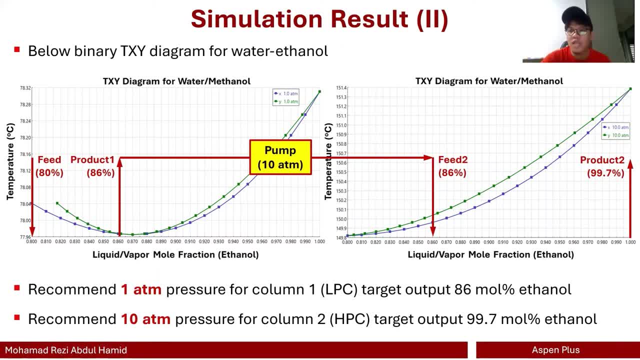 is here 151, so is here 151. so we all know that the reboiler or bottom, we all know that the reboiler or bottom, we all know that the reboiler or bottom section is always higher, section is always higher, section is always higher, higher temperature than the uh distillate. 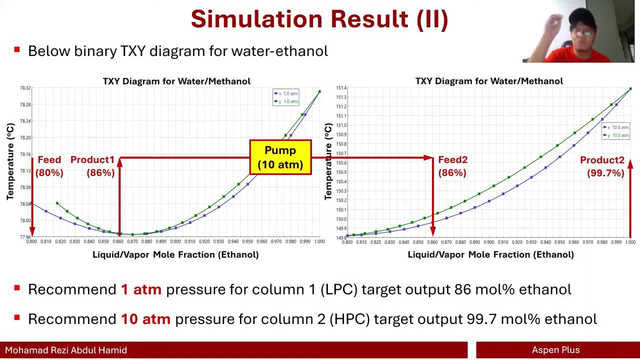 higher temperature than the uh distillate higher temperature than the uh distillate uh, uh distillate uh, uh distillate uh distillate part. so in this case, our distillate part, so in this case, our distillate part. so in this case, our ethanol will live at the. 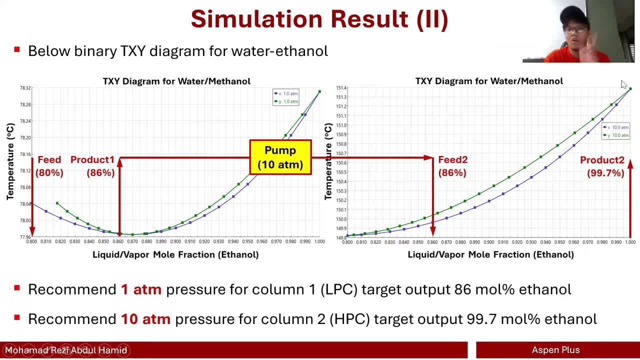 ethanol will live at the. ethanol will live at the bottom section of our high pressure, bottom section of our high pressure, bottom section of our high pressure column, not at the top section. column not at the top section. column not at the top section for this one, for the first low pressure, 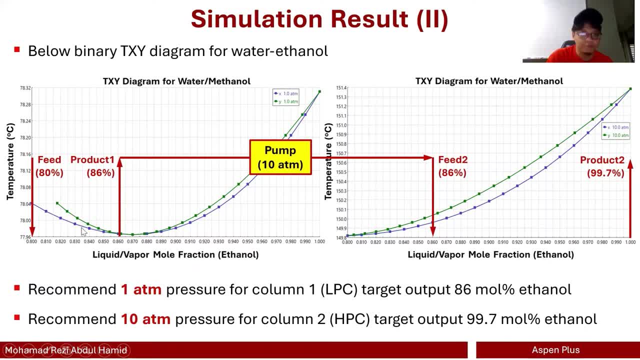 for this one, for the first low pressure. for this one for the first low pressure column. yes, they will live at uh column. yes, they will live at uh column. yes, they will live at uh. they will live at the distillate at the. they will live at the distillate at the. 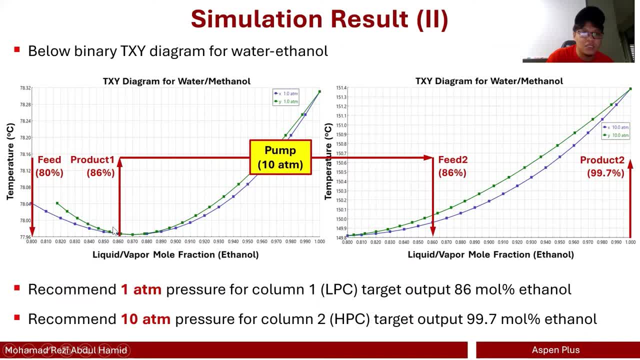 they will live at the distillate, at the distillate section. because this is at distillate section, because this is at distillate section, because this is at lower temperature, lower temperature, lower temperature compared to the uh the initial one, compared to the uh the initial one. 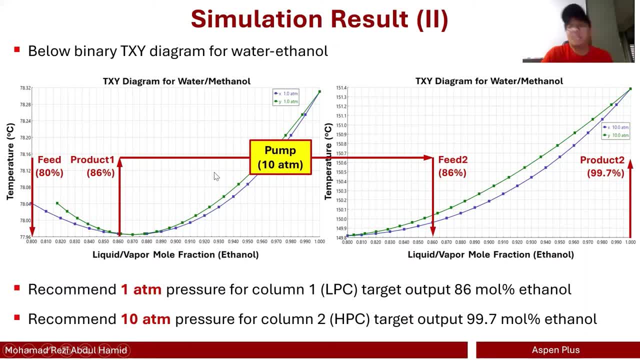 compared to the uh- the initial one. compared to the feed one: okay. compared to the feed one: okay. compared to the feed one: okay. um, that's how i'm gonna design my uh. compared to the uh- the initial one: okay. um, that's how i'm gonna design my uh. 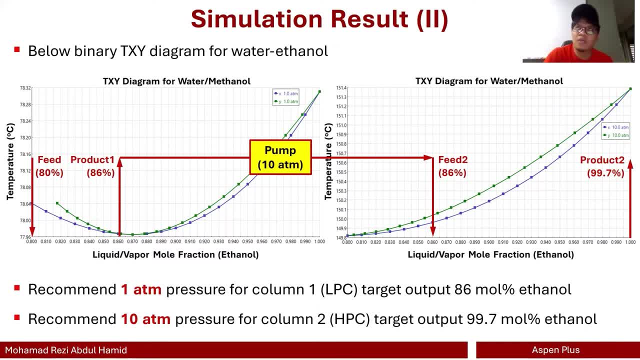 compared to the uh, the initial one. okay, um, that's how i'm gonna design my uh, pleasure swing distillation. so, uh, pleasure swing distillation. so, uh, pleasure swing distillation. so, uh, going back to our s1 plus, and we will going back to our s1 plus and we will. 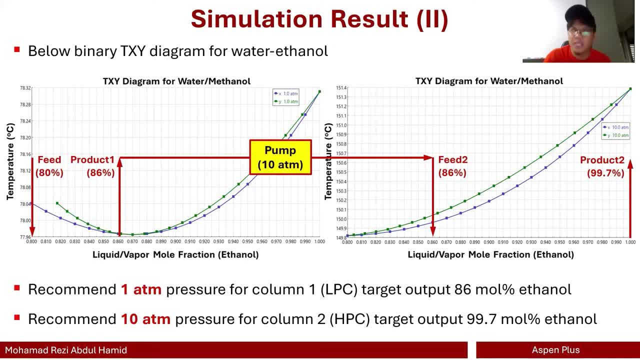 going back to our s1 plus and we will try to do simulation and see whether we try to do simulation and see whether we try to do simulation and see whether we can get 99.7, can get 99.7, can get 99.7 more percent purity of ethanol. 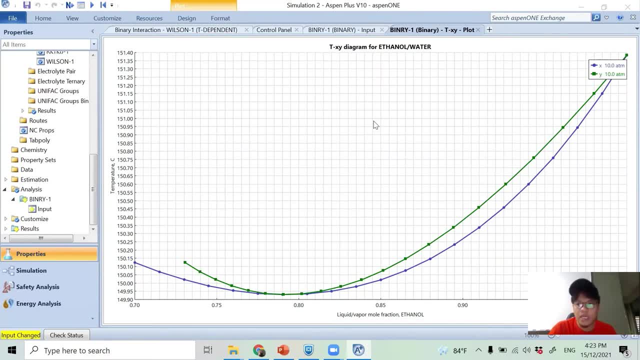 okay, uh, coming back to our s10 plus. okay, uh, coming back to our s10 plus. okay, uh, coming back to our s10 plus. gui, graphical user interface. um, i'm gui graphical user interface. um, i'm gui graphical user interface. um, i'm pretty much done with the, with the. 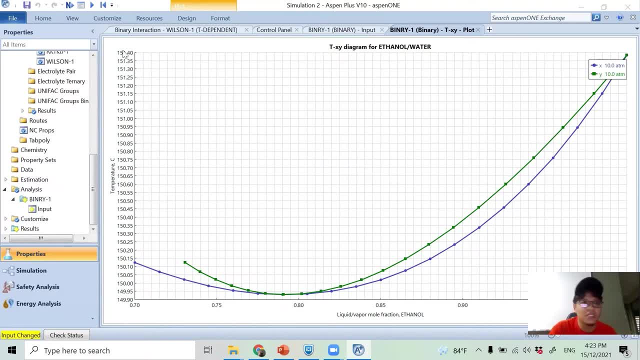 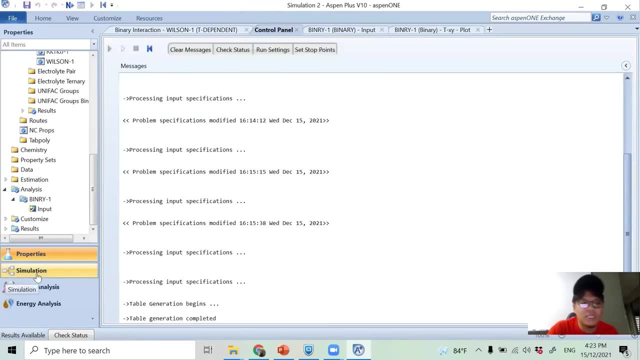 pretty much done with the, with the property section of the property section of the property section of the s1 plus. just hit next, i guess, and then i'm gonna switch to the, and then i'm gonna switch to the, and then i'm gonna switch to the simulation environment and create my own. 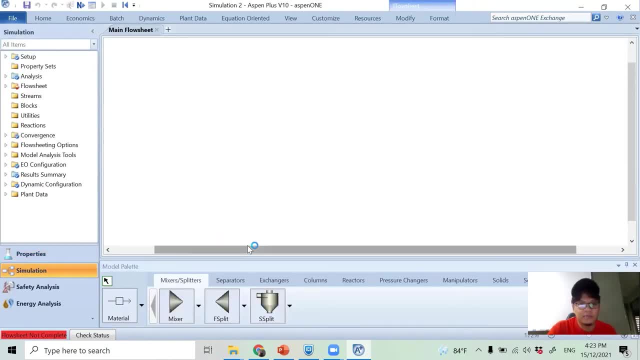 simulation environment and create my own simulation environment and create my own afro sheet. afro sheet, afro sheet, um, um, um. okay, i'm gonna use the column uh red flag. okay, i'm gonna use the column uh red flag. okay, i'm gonna use the column uh red flag column. i put one column here. maybe i will. 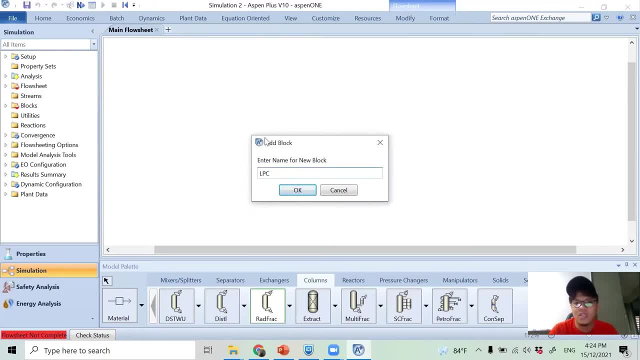 column. i put one column here, maybe i will column. i put one column here. maybe i will write down a low piece lpc representing: write down a low piece lpc representing. write down a low piece lpc representing low pressure column and then i will have low pressure column and then i will have. 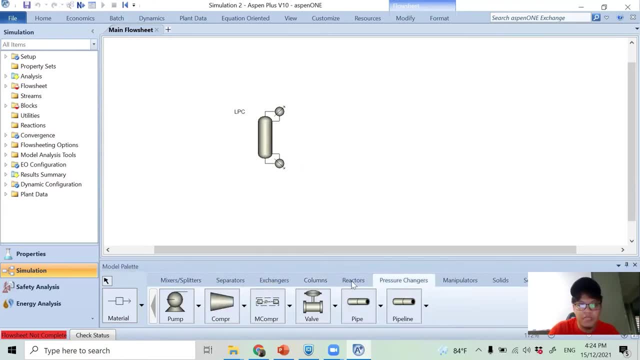 low pressure column. and then i will have a pump uh which is under a pump uh, which is under a pump uh which is under pressure changes. i'll put pump here, pressure changes. i'll put pump here, pressure changes. i'll put pump here empty, empty, empty. and then i will choose another column. 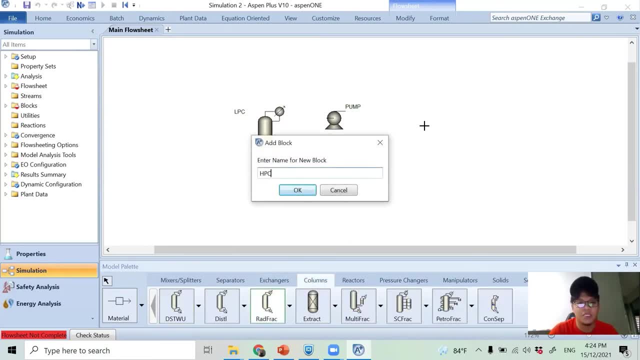 and then i will choose another column, and then i will choose another column. red flag, red flag, red flag here, hbc, here, hbc, here, hbc as usual. connect as usual. connect as usual. connect. this is my feed, this is my feed, this is my feed, feed one: 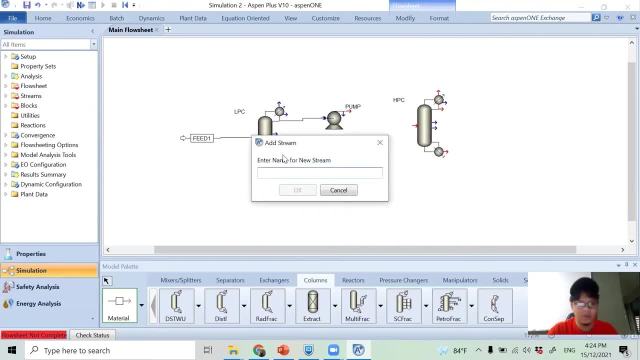 feed one, feed one. this is my distillate. this is my distillate. this is my distillate. i will let down this product one. i will let down this product one. i will let down this product one, and then this one, and then this one. 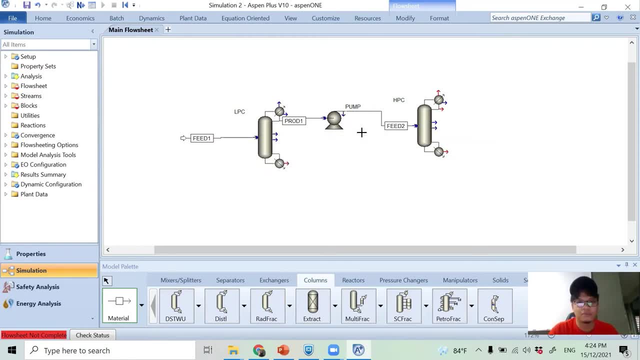 and then this one i will write down as feed two: i will write down as feed two. i will write down as feed two. this one i will write down as a water. this one i will write down as a water. this one i will write down as a water one. 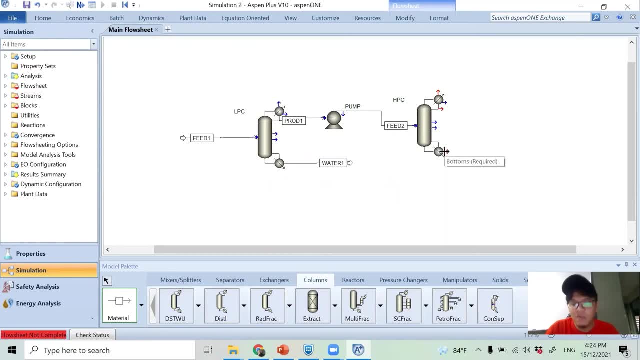 one one. water one now. if you remember the product, water one now. if you remember the product, water one now. if you remember the product is at higher temperature, is at higher temperature, is at higher temperature. so it should the ethanol should live at. so it should, the ethanol should live at. 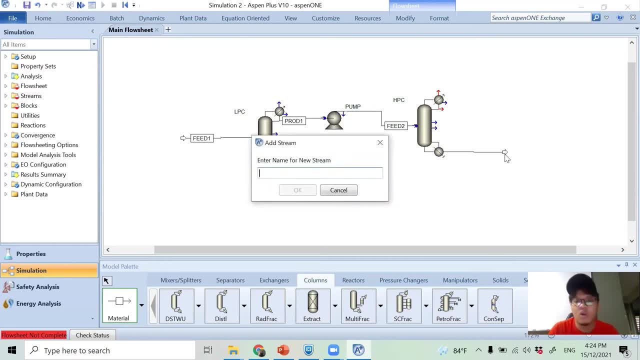 so it should. the ethanol should live at the bottom, the bottom, the bottom section of the uh, of the column, section of the uh, of the column, section of the uh of the column. so here we'll write down product two. so here we'll write down product two. 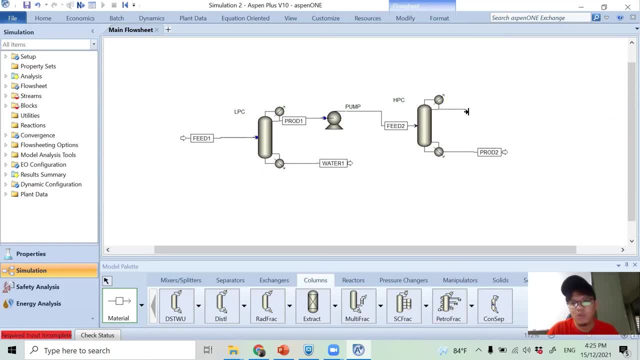 so here we'll write down product two: and water remainder of the water, i guess. and water remainder of the water, i guess. and water remainder of the water, i guess. distribute subjects of water, distribute subjects of water, distribute subjects of water. um, so let me zoom in a bit. 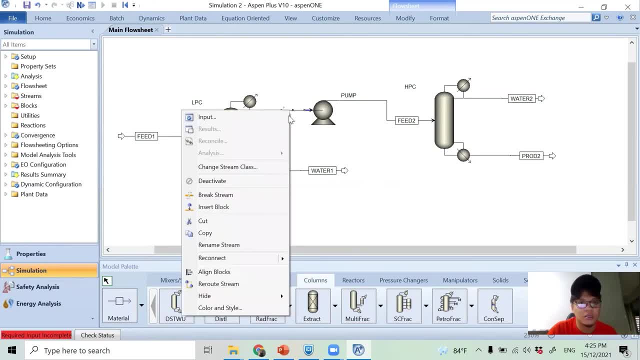 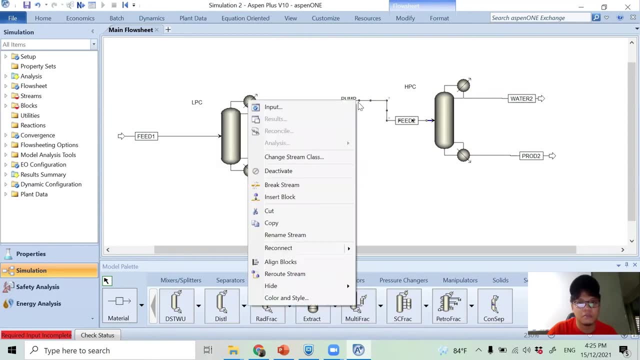 um so, let me zoom in a bit. um so, let me zoom in a bit, let me make it nicer. okay, okay, okay, uh, just uh hit next or just double click. uh, just uh hit next or just double click. uh, just uh hit next or just double click feed. 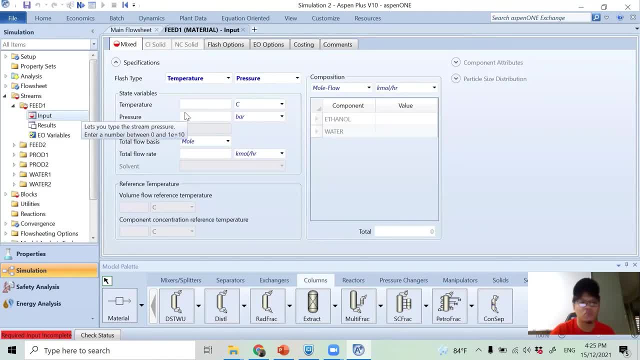 feed feed. uh feed stream it will. it will redirect you. uh feed stream it will. it will redirect you uh feed stream it will. it will redirect you to the same, to the same, to the same input form. so our feed is enters at 90 input form. so our feed is enters at 90. 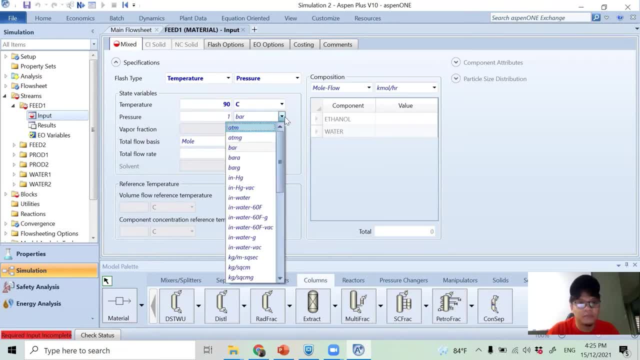 input form, so our feed is enters at 90 degrees celsius and pressure of one degrees celsius and pressure of one degrees celsius and pressure of one atmosphere, atmosphere, atmosphere. uh more mole flow is 150 kilomoles per? uh more mole flow is 150 kilomoles per. 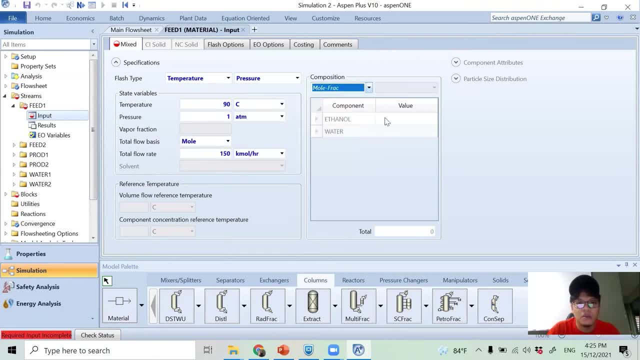 uh more, mole flow is 150 kilomoles per hour. this one is mole fraction hour. this one is mole fraction hour. this one is mole fraction: ethanol is 80 percent and then water is ethanol is 80 percent, and then water is ethanol is 80 percent and then water is 20 percent. now 80 and 20 is basically. 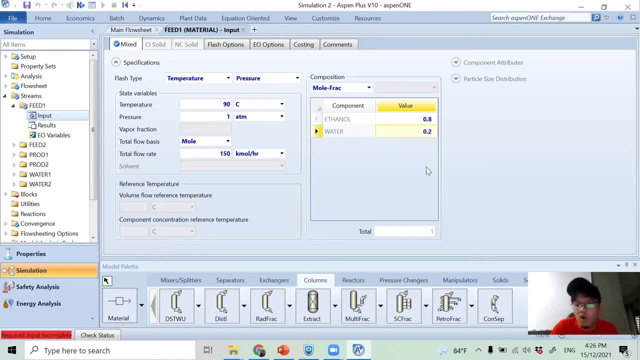 20 percent now 80, and 20 is basically 20 percent, now 80, and 20 is basically representing the representing the representing the output of the ethanol production, output of the ethanol production, output of the ethanol production processes, normally from fermentation processes, normally from fermentation. 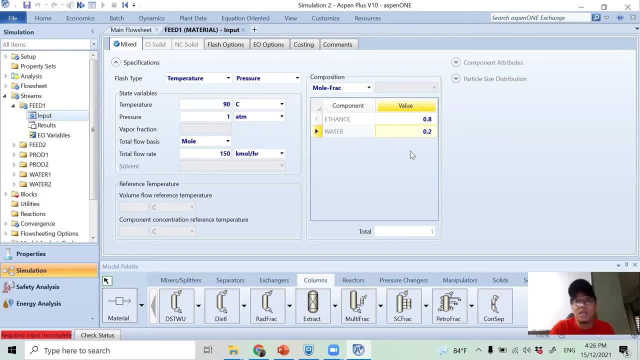 processes normally from fermentation, like fermentation of corn, like the like fermentation of corn, like the like fermentation of corn, like the united states or maybe a more commercial united states or maybe a more commercial united states, or maybe a more commercial if you, if you're talking about, uh, a more? 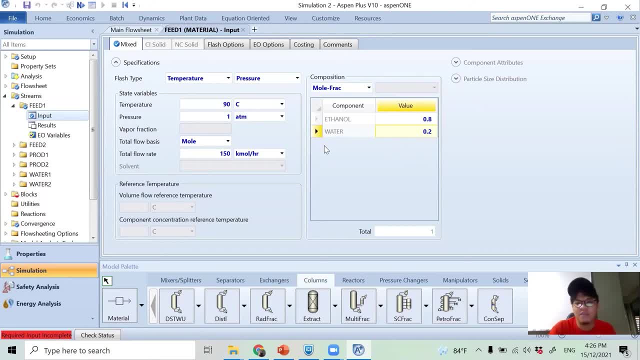 if you, if you're talking about uh a more, if you, if you're talking about uh a more, uh, uh uh. a process processes other than fermentation. a process processes other than fermentation. a process processes other than fermentation. ethanol is normally produced. ethanol is normally produced. ethanol is normally produced. can be produced from the dehydration of. 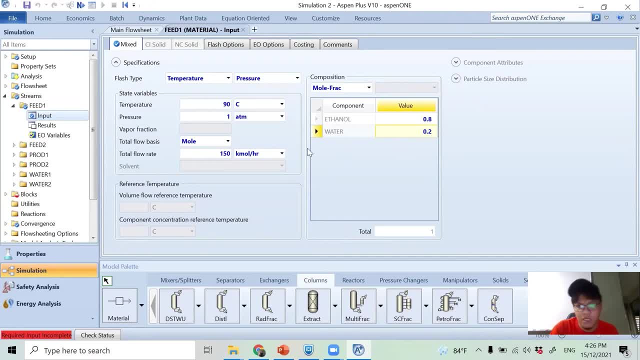 can be produced from the dehydration of. can be produced from the dehydration of 18, i think. if i'm not mistaken. can be produced from the dehydration of 18, i think. if i'm not mistaken, can be produced from the dehydration of 18, i think, if i'm not mistaken. uh, but, but you can have a look. 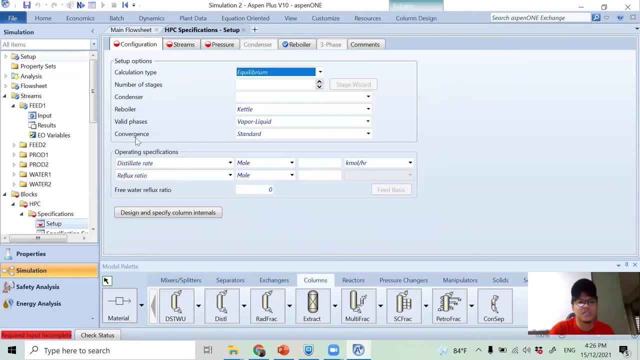 uh, but, but you can have a look. uh, but, but you can have a look. okay, i'm done specifying my feed. uh hit. okay, i'm done specifying my feed, uh hit. okay, i'm done specifying my feed, uh hit. next it will redirect you to my high. 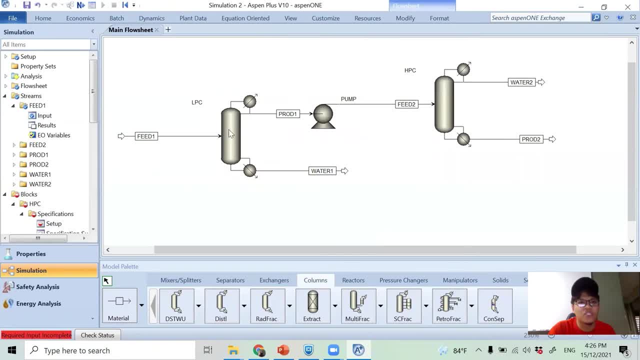 next, it will redirect you to my high. next, it will redirect you to my high pressure column. okay, you know what i'm pressure column. okay, you know what i'm pressure column. okay, you know what i'm gonna do a low pressure column first. gonna do a low pressure column first. 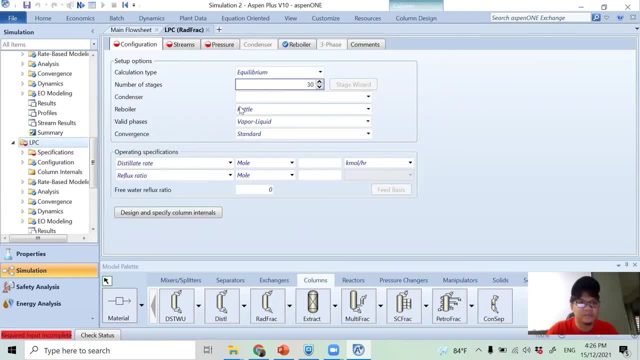 gonna do a low pressure column first. let me click low pressure column number. let me click low pressure column number. let me click low pressure column. number of stages is 30.. of stages is 30.. of stages is 30.. condensate is total. total condenser. 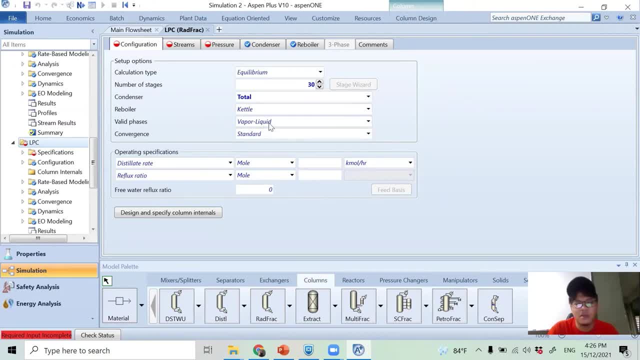 condensate is total total condenser. condensate is total total condenser because, if it's like a partial, because if it's like a partial, because if it's like a partial, the different uh different uh type of the different uh different uh type of. 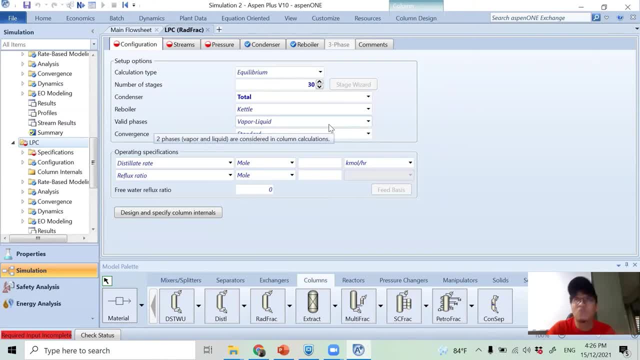 the different uh, different uh type of condenser. i'm afraid it's gonna go to condenser. i'm afraid it's gonna go to condenser. i'm afraid it's gonna go to the pump in a two-phase kind of uh two in the pump, in a two-phase kind of uh two in. 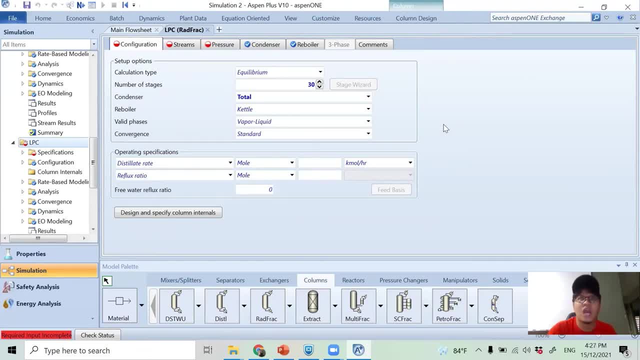 the pump in a two-phase kind of uh, two in in in in two-phase, but but i, i want it in in in in in two-phase, but but i, i want it in in in in two-phase, but but i, i want it. i want only liquid enters the pump. 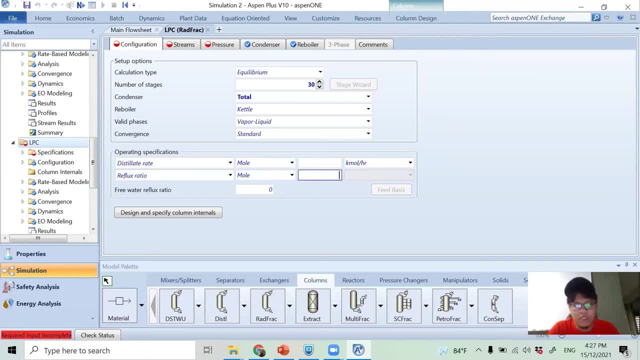 i want only liquid enters the pump. i want only liquid enters the pump. uh reflux ratio here: uh 3.71. uh the uh reflux ratio here: uh 3.71. uh the uh reflux ratio here: uh 3.71. uh the 3.71 here. i took it from the general. 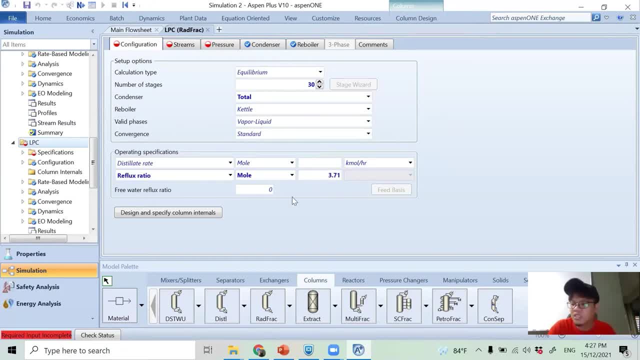 3.71- here i took it from the general. 3.71- here i took it from the general because i'm kind of lazy to figure out, because i'm kind of lazy to figure out, because i'm kind of lazy to figure out what's the best reflux ratio. but uh, 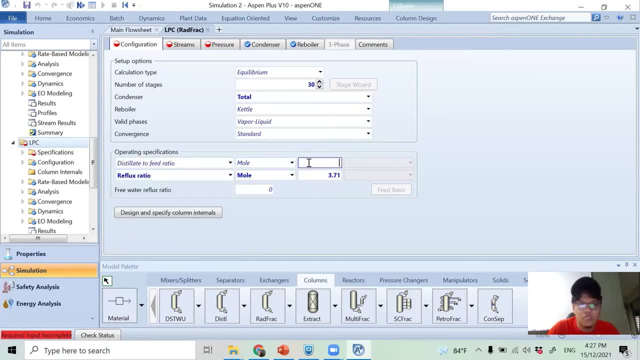 what's the best reflux ratio? but uh, what's the best reflux ratio? but uh, distillate to feed ratio. here i choose distillate to feed ratio. here i choose distillate to feed ratio. here i choose around 0.9 to 9, because 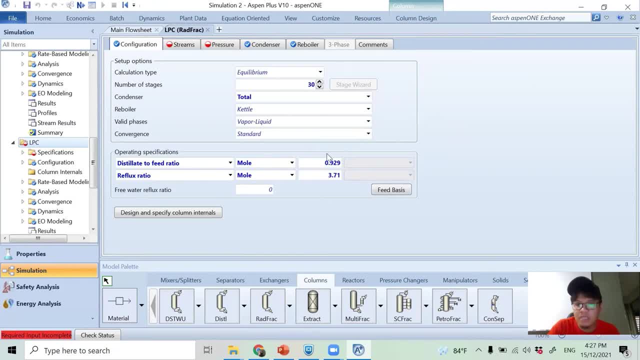 around 0.9 to 9. because around 0.9 to 9, because, uh, this is not the general data by the uh. this is not the general data by the uh. this is not the general data. by the way, this is my own data because from uh. 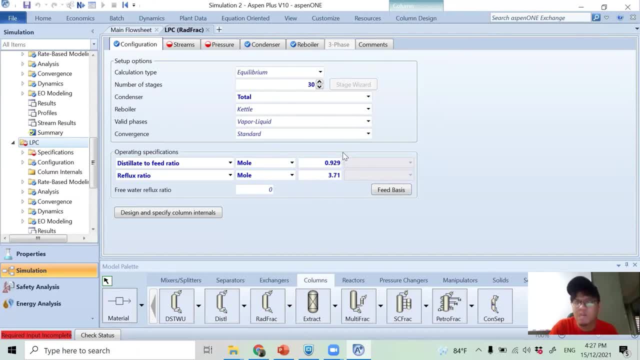 way, this is my own data because from uh. way, this is my own data because from uh. if i'm not mistaken, when i use the, if i'm not mistaken when i use the. if i'm not mistaken when i use the general data, i cannot get around 99.5. 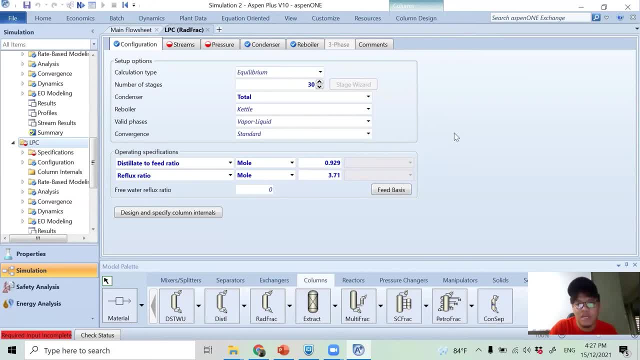 general data. i cannot get around 99.5 general data. i cannot get around 99.5. purity of water. i don't know why, but purity of water. i don't know why, but purity of water. i don't know why, but this is the value that i did. i like it. 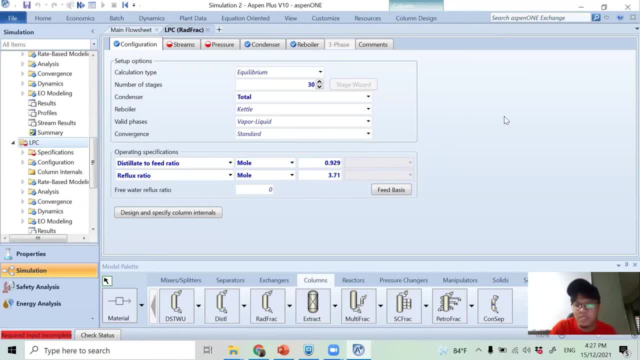 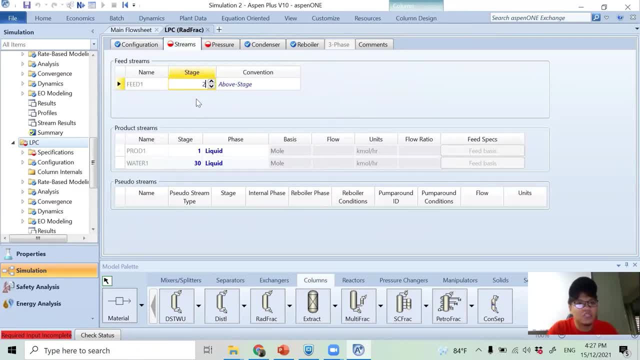 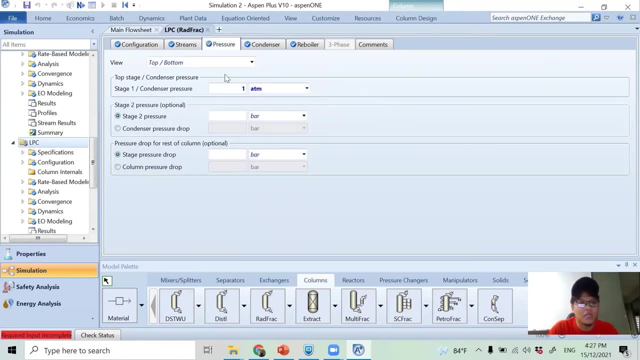 sensitivity analysis: sensitivity analysis and then move to the stream: the stream and then move to the stream. the stream and then move to the stream. the stream enters at stage 23. enters at stage 23. enters at stage 23: pressure: pressure pressure 180m- 180m. 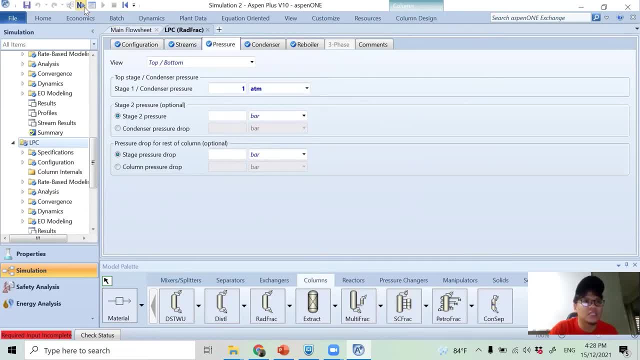 180m. i'm just gonna assume no pressure drop. i'm just gonna assume no pressure drop. i'm just gonna assume no pressure drop. okay, hit next. okay, hit next. okay, hit next. it will redirect me to a high pressure. it will redirect me to a high pressure. 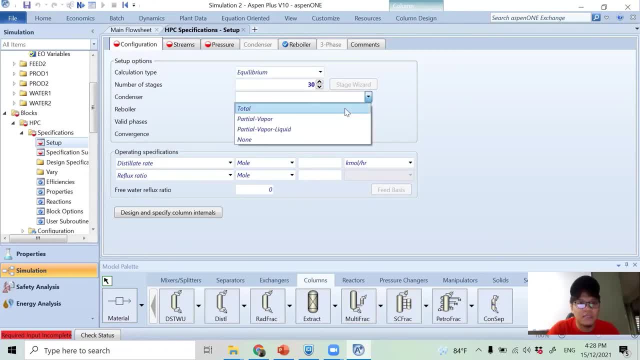 it will redirect me to a high pressure column. the same one, same number of column. the same one, same number of column. the same one, same number of stages. some same condenser reflux ratio stages, some same condenser reflux ratio stages, some same condenser reflux ratio is. 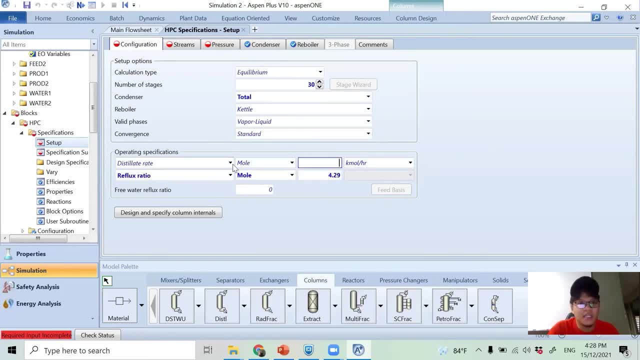 is is 4.29, 4.29, 4.29 distillate rate. uh just use a distillate distillate rate. uh just use a distillate distillate rate. uh just use a distillate to feed ratio around. 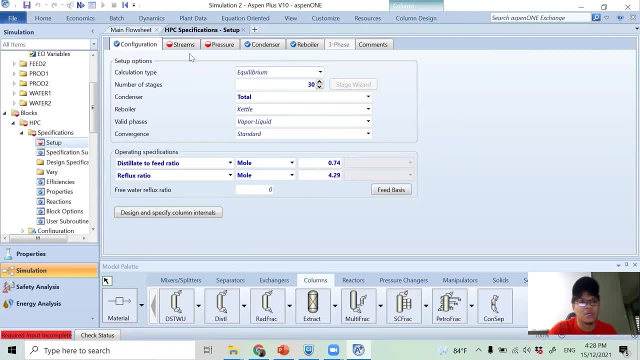 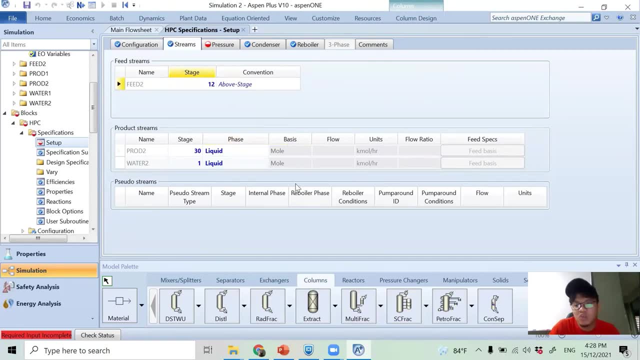 to feed ratio around to feed ratio around 0.74. okay screen coming in at stage number 12. okay screen coming in at stage number 12. okay screen coming in at stage number 12. because, because, because, uh, i decided to not use the stage 23. 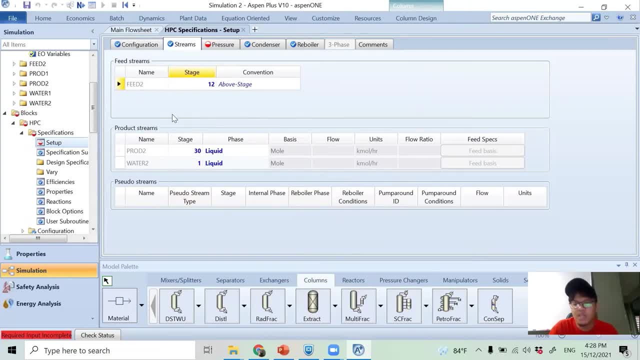 uh, i decided to not use the stage 23. uh, i decided to not use the stage 23 because what i found is at stage 12. they because what i found is at stage 12. they because what i found is at stage 12, they have they allow for a bit higher, higher. 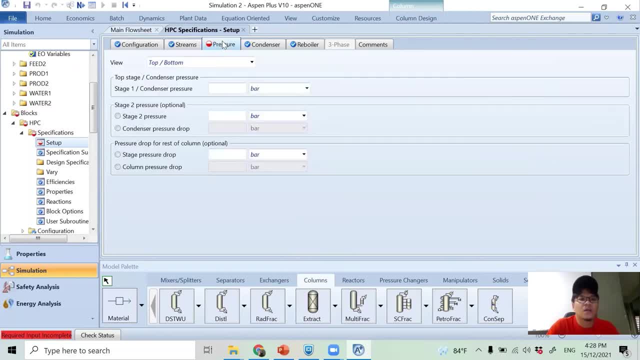 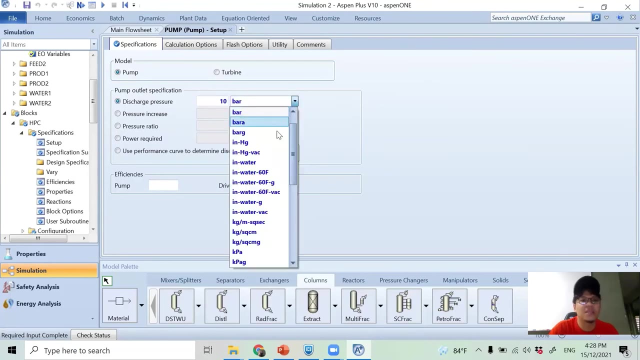 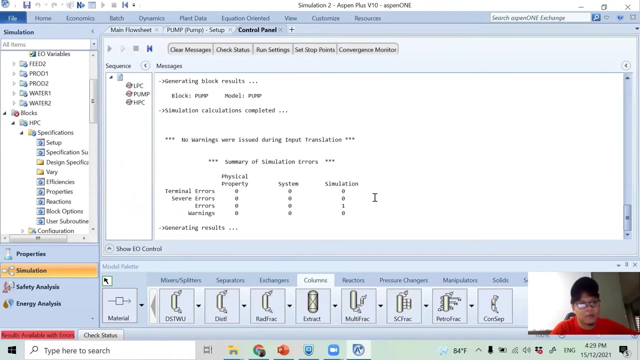 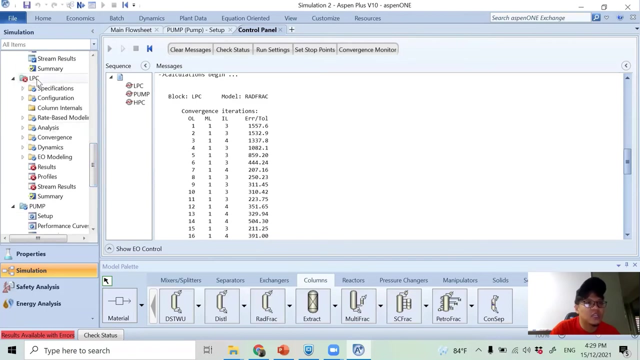 have they allow for a bit higher, higher? have they allow for a bit higher, higher, higher, higher, higher enrichment, uh, uh, uh, pleasure, pleasure, pleasure, 10 atmosphere, pressure, and, and and, and, okay, okay, okay, where is it? it's under? where is it it's under? where is it it's under? the area is under low pressure column. so. 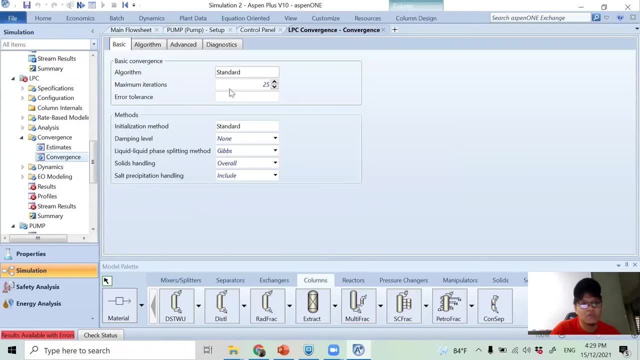 the area is under low pressure column. so the area is under low pressure column. so if that's the case, let me do the. if that's the case, let me do the. if that's the case, let me do the. convergence, convergence, convergence. maybe i'll do 300. 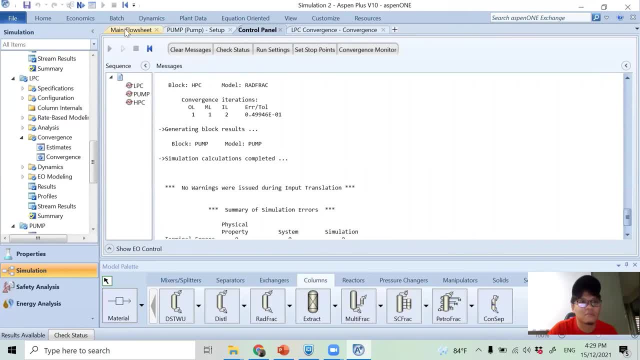 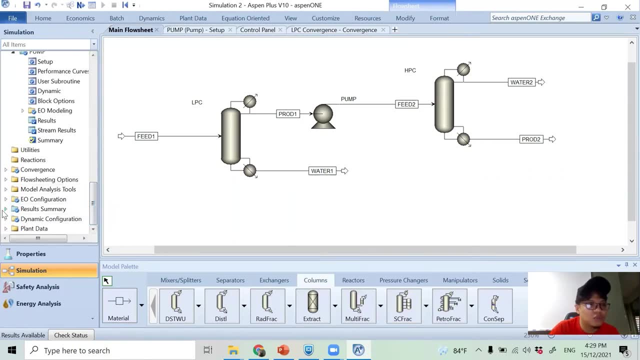 okay, good, okay, i got a result, so let's see the. okay, i got a result, so let's see the. okay, i got a result, so let's see the result. uh, just go to stream summary and then go. uh, just go to stream summary and then go. 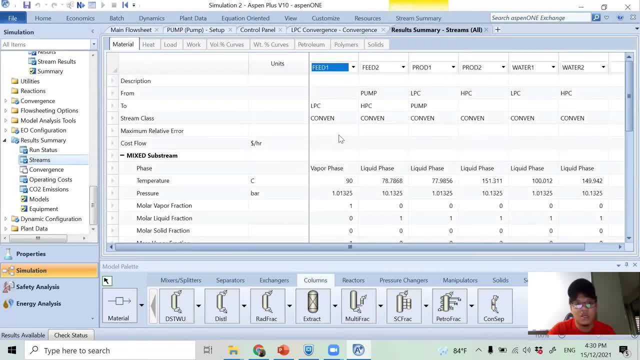 uh, just go to stream summary and then go to screen, and then to screen, and then go to screen, and then to screen and then go to screen, and then you will see the result. you will see the result. you will see the result. um, um, um, as i said, water. 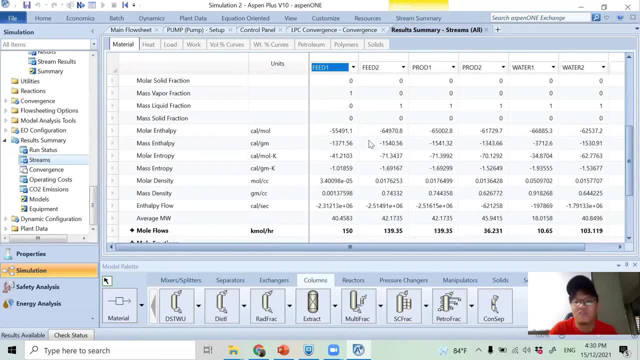 as i said, water. as i said, water should have the purity around 99.5, should have the purity around 99.5, should have the purity around 99.5, but the water should be at the bottom, but the water should be at the bottom. 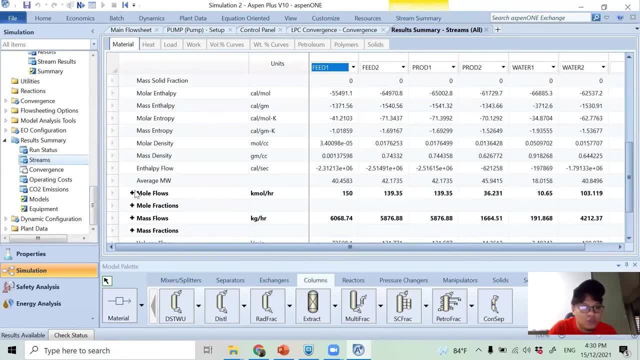 but the water should be at the bottom section of your low pressure column section of your low pressure column, section of your low pressure column. so i choose more flow. i expand more, so i choose more flow. i expand more, so i choose more flow. i expand more fraction here. 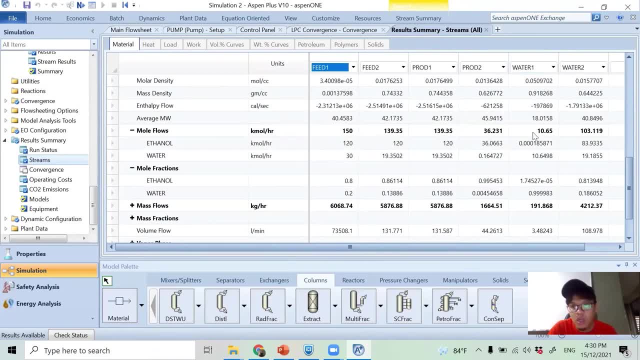 fraction here. fraction here: now the bottom of my low pressure, now the bottom of my low pressure, now the bottom of my low pressure. column should be water one. so i got. column should be water one. so i got. column should be water one. so i got around 99.999. 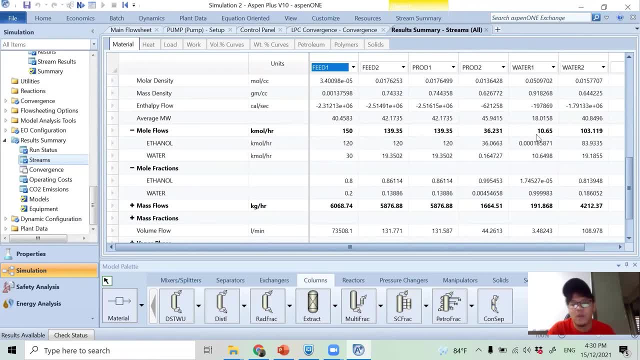 around 99.999, around 99.999, and, and, and just a more flows around 10 more. uh, just a more flows around 10 more. uh, just a more flows around 10 more. uh, kilo mole per hour. kilo mole per hour, kilo mole per hour. now my methanol, no, my ethanol should. 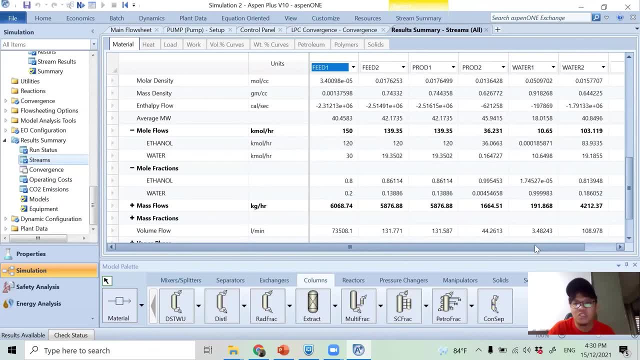 now my methanol? no, my ethanol should now my methanol? no, my ethanol should leave at the bottom section of my high leave, at the bottom section of my high leave, at the bottom section of my high pressure column. so it should be product pressure column. so it should be product. 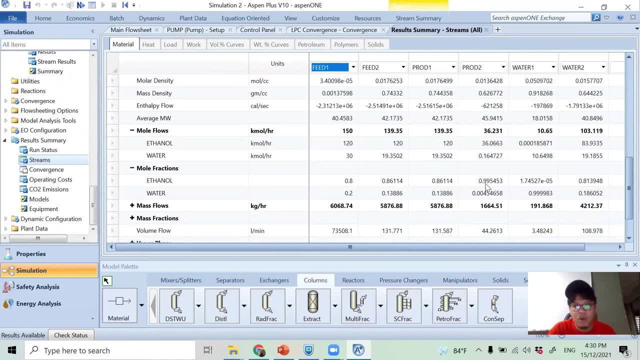 pressure column. so it should be product number two, number two, number two: i got around 99.5, okay, i got around 99.5. okay, i got around 99.5, okay, uh, uh, uh, 0.5, uh, more fraction. 0.5, uh, more fraction. 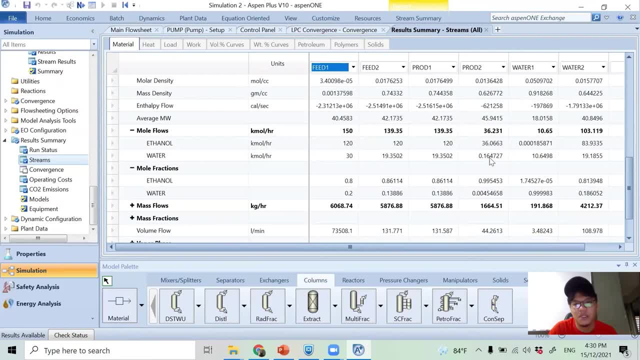 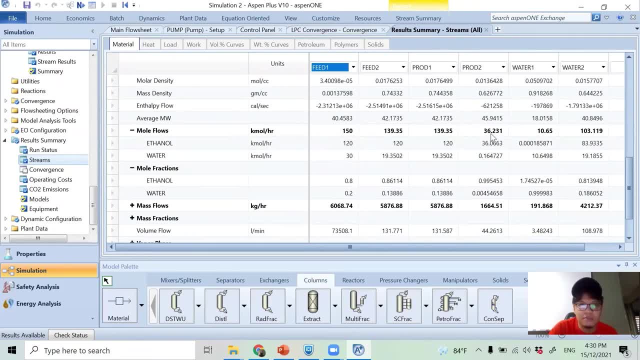 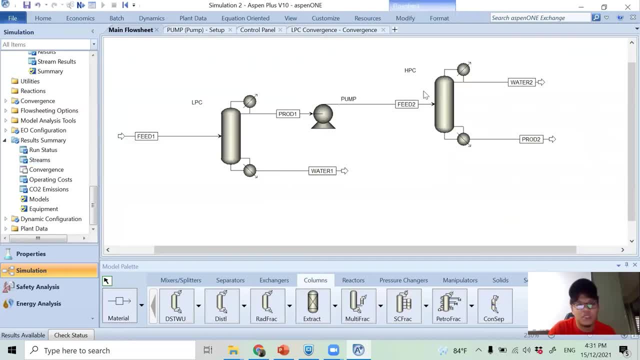 uh, more of product. uh, more of product. okay, if i want to get around 99.5, it's okay. if i want to get around 99.5, it's okay. if i want to get around 99.5, it's not that difficult. just switch this to. 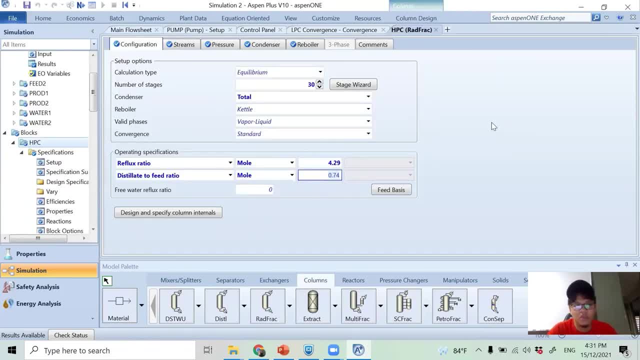 not that difficult, just switch this to. not that difficult, just switch this to: maybe, maybe, maybe, i don't know, i don't know, i don't know- 0.73, 0.739, 0.73, 0.739, 0.73, 0.739, 738, for example. 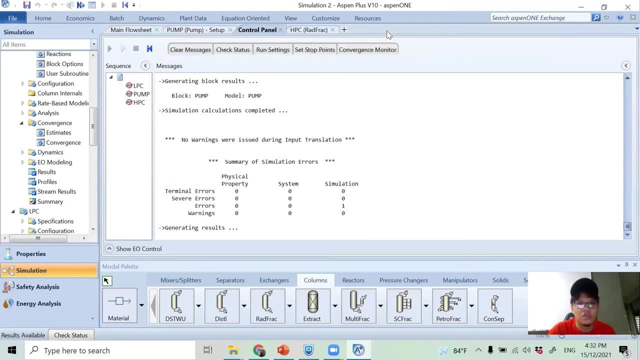 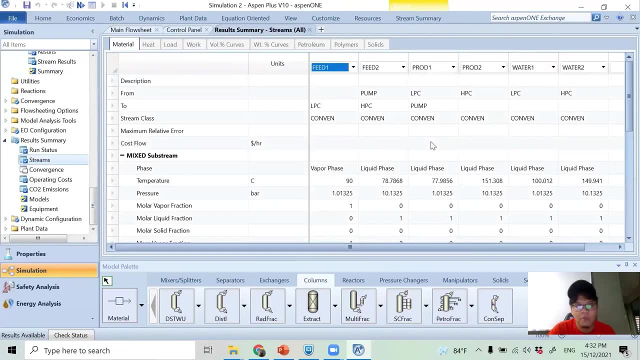 738, for example, 738, for example. okay, and then just go to result: where's my, okay? and then just go to result: where's my, okay? and then just go to result. where's my result? uh, scroll down, go to stream. uh, scroll down, go to stream. 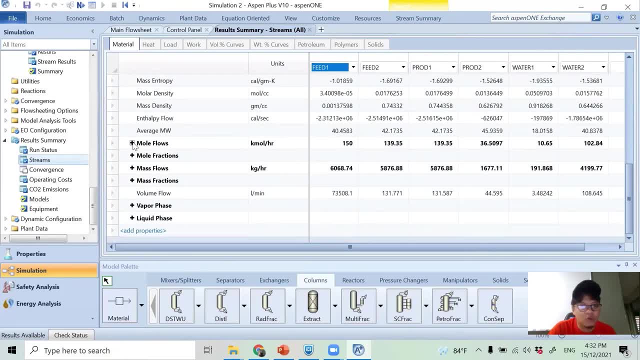 uh, scroll down, go to stream. i should be able to get 99.6 percent. or i should be able to get 99.6 percent, or i should be able to get 99.6 percent or seven percent more affection more. seven percent more affection more. 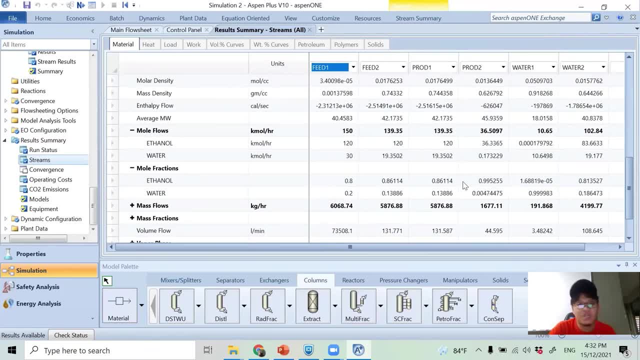 seven percent. more affection, more affection, affection, affection. ah, still 99.5, ah, still 99.5. ah, still 99.5. uh, uh, still 99.5. okay, never mind, uh, it's fine. okay, never mind, uh, it's fine. okay, never mind, uh, it's fine. but if you want to get another 9.7, just. 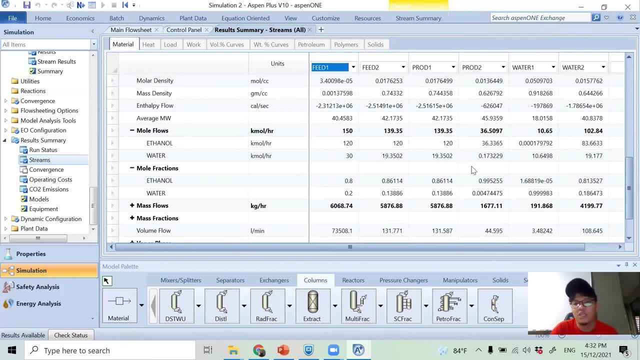 but if you want to get another 9.7, just, but if you want to get another 9.7, just, just tweak the value, the value of a just tweak, the value, the value of a just tweak, the value, the value of a hyperj column, and you should be able to. 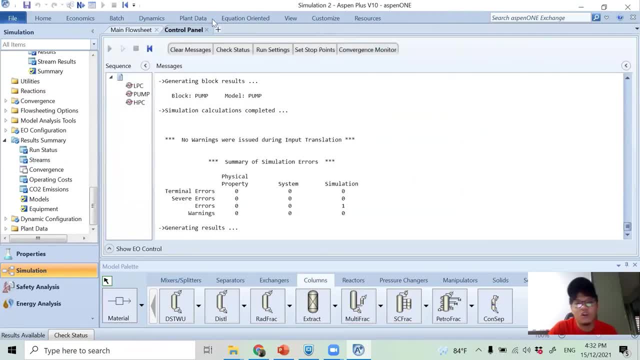 hyperj column and you should be able to hyperj column and you should be able to get it. get it, get it. okay, i'm going to analyze all the result. okay, i'm going to analyze all the result. okay, i'm going to analyze all the result in my simulation sections. actually, i 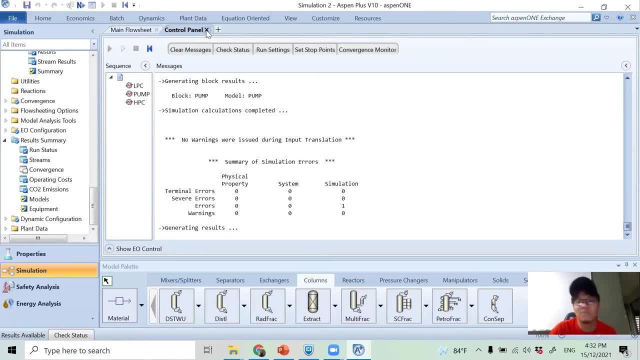 in my simulation sections. actually i in my simulation sections, actually i have done the optimization like in the, have done the optimization like in the, have done the optimization like in the previous previous previous simulation. but uh, maybe for this demo i simulation, but uh, maybe for this demo i. 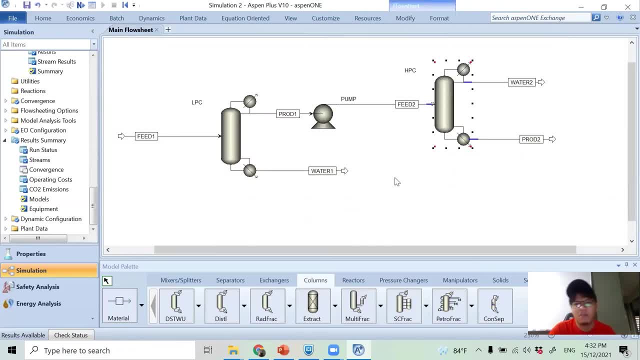 simulation, but, uh, maybe for this demo. i don't get 99.5, don't get 99.5, don't get 99.5, 99.7, but i don't see, i don't see why not 99.7, but i don't see, i don't see why not. 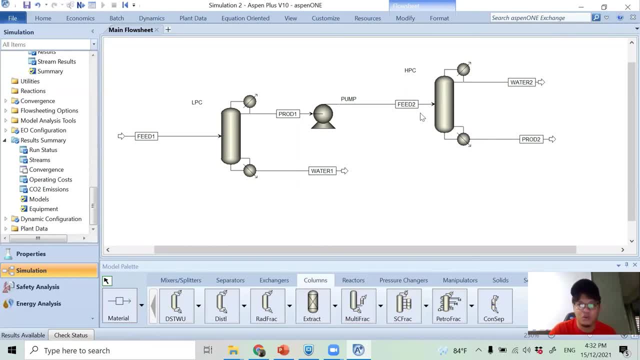 99.7. but i don't see. i don't see why not? because it's just a simple tweaking of, because it's just a simple tweaking of, because it's just a simple tweaking of the condition of the second column. the condition of the second column. 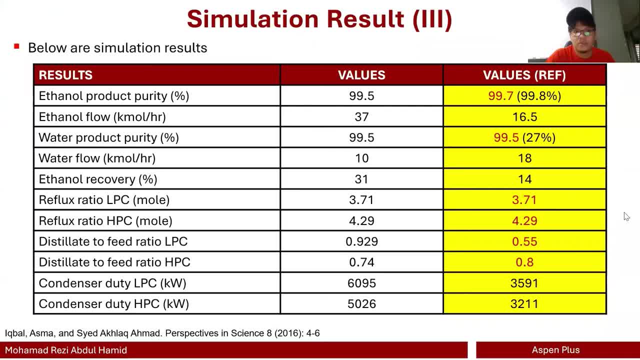 the condition of the second column. so yeah, let's go back to our. so yeah, let's go back to our. so yeah, let's go back to our presentation slides. presentation slides, presentation slides. so, as you can see here, these are the. so, as you can see here, these are the. 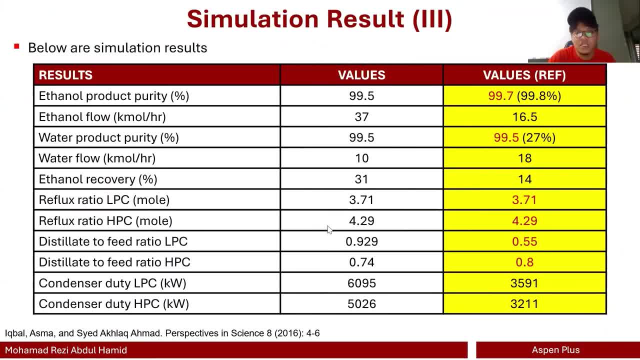 so, as you can see here, these are the tables. all these are the values that are tables. all these are the values that are tables. all these are the values that are obtained from my simulations um. for the obtained from my simulations, um. for the obtained from my simulations um. for the current simulation, i was able to get 99.5. 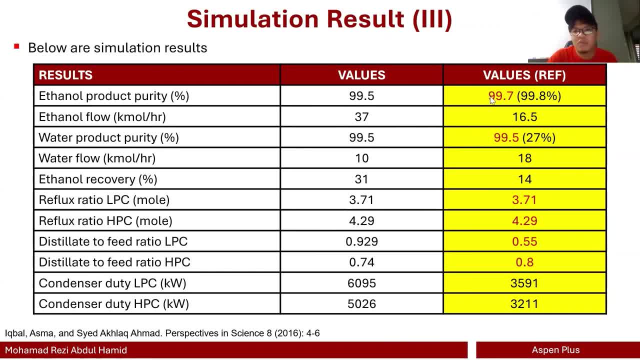 current simulation: i was able to get 99.5. current simulation: i was able to get 99.5. more percent of ethanol, but the more percent of ethanol, but the more percent of ethanol, but the requirement is 99.7 percent. requirement is 99.7 percent. 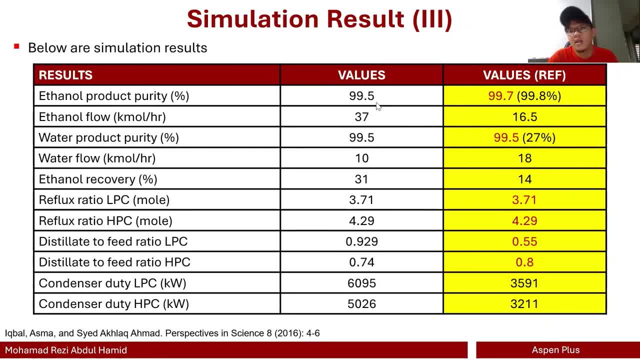 requirement is 99.7 percent. uh, which i think is fine. uh, which i think is fine. uh, which i think is fine. uh, it's a matter of tweaking the the uh. it's a matter of tweaking the the uh. it's a matter of tweaking the. the condition of the high pressure column. 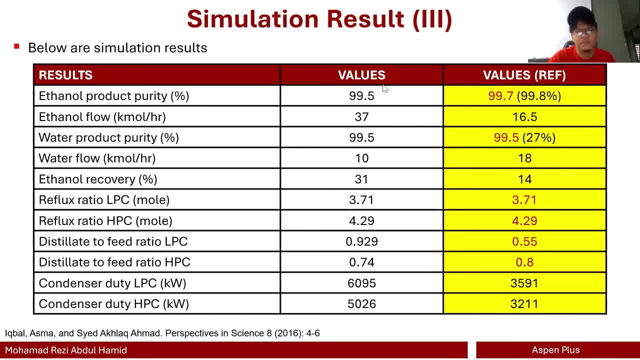 condition of the high pressure column. condition of the high pressure column. it's not that difficult, but if you want, it's not that difficult. but if you want, it's not that difficult. but if you want to use it to use it, to use it, if you want to do it, please go ahead and 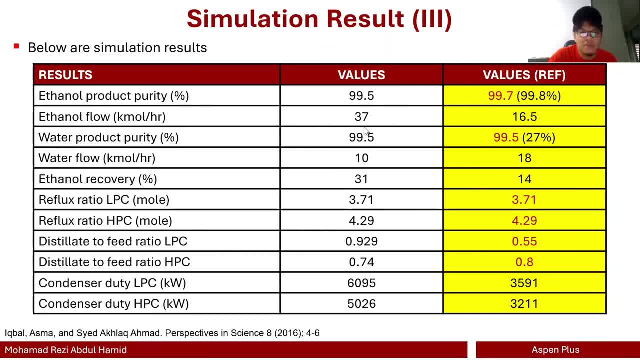 if you want to do it, please go ahead. and if you want to do it, please go ahead and do it. and then the ethanol purity- i got, do it. and then the ethanol purity, i got do it. and then the ethanol purity, i got about 37, about 37. 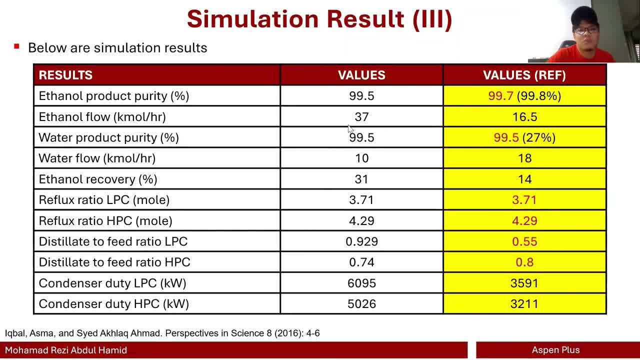 about 37- 37 kilowatt per hour water beauty. i 37 kilowatt per hour water beauty. i 37 kilowatt per hour water beauty. i got 99.5 percent, got 99.5 percent, got 99.5 percent. okay, uh, uh, uh, i got it, uh. following the: 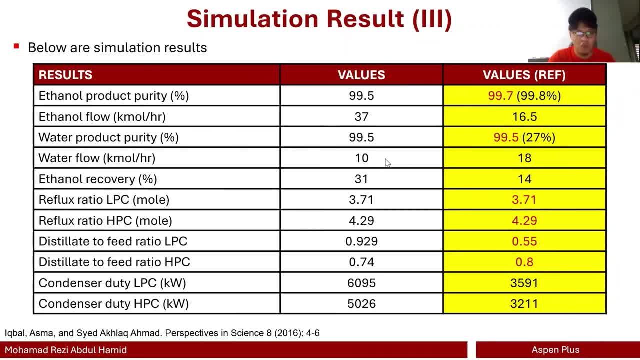 okay, uh, uh uh, i got it uh. following the okay, uh, uh, uh, i got it uh. following the requirement uh water mode flow: i got requirement uh water mode flow. i got requirement uh water mode flow. i got around 10 kilowatt per hours, around 10 kilowatt per hours. 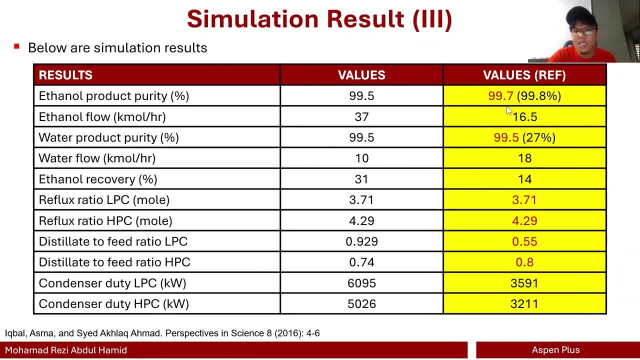 around 10 kilowatt per hours. ethanol recovery here: i got around 31. ethanol recovery here: i got around 31. ethanol recovery here: i got around 31. okay, the one on the right hand side here: okay. the one on the right hand side here: okay, the one on the right hand side here, the one highlighted in yellow. these are 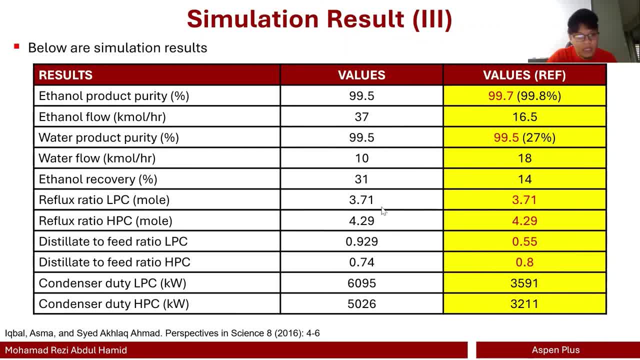 the one highlighted in yellow. these are the one highlighted in yellow. these are the general result, by the way, the general result, by the way, the general result, by the way, and these are my reflux ratio, uh, and these are my reflux ratio. uh, and these are my reflux ratio. uh, obviously, this reflux ratio will be: 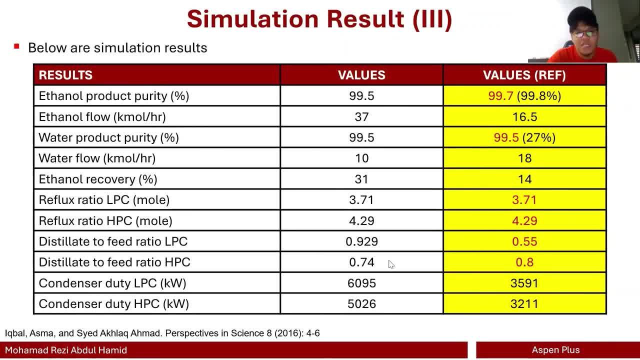 obviously this reflux ratio will be. obviously this reflux ratio will be similar, because i just copy and paste similar, because i just copy and paste similar, because i just copy and paste their result, but the only thing that i their result, but the only thing that i their result, but the only thing that i feel is quite different is this: 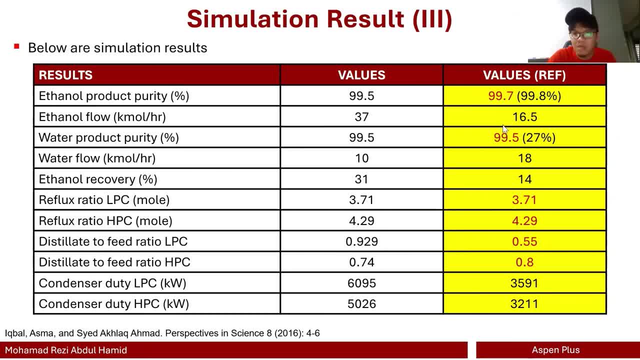 feel is quite different. is this feel is quite different. is this distillate to feed ratio: okay to obtain distillate to feed ratio. okay to obtain distillate to feed ratio. okay to obtain more as the same amount say beauty. more as the same amount, say beauty. 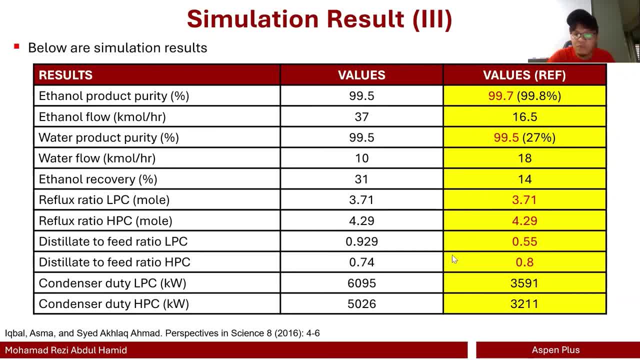 more as the same amount, say beauty. i have to use this one, 0.92 and 0.74. i have to use this one, 0.92 and 0.74. i have to use this one, 0.92 and 0.74, and i have no idea. 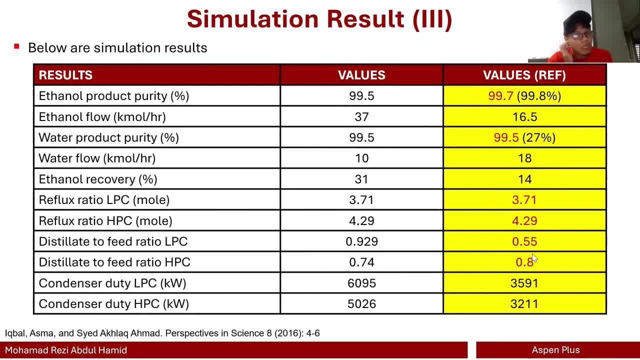 and i have no idea. and i have no idea how they got 0.55 and 0.8, how they got 0.55 and 0.8, how they got 0.55 and 0.8. actually, i did try to use their result. 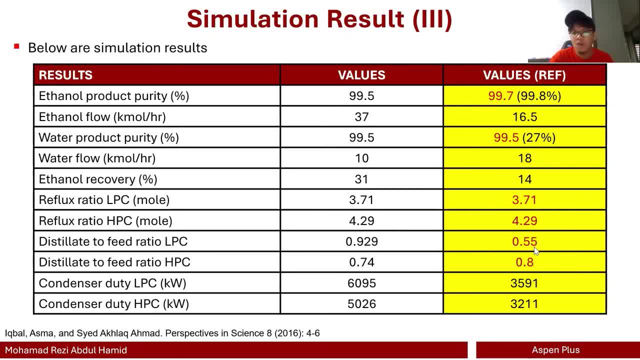 actually, i did try to use their result. actually, i did try to use their result. yeah, yeah, they are distillate to feed. yeah, yeah, they are distillate to feed. yeah, yeah, they are distillate to feed ratio. but what i got is this ratio. but what i got is this: 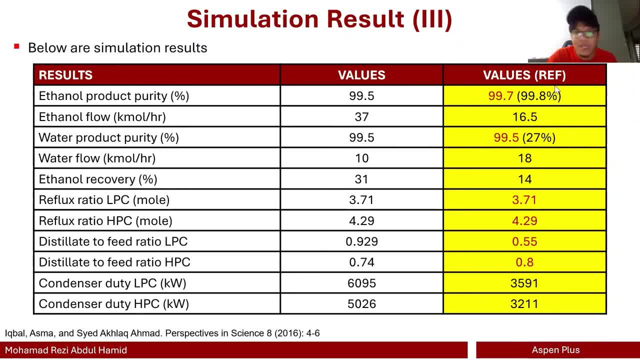 ratio. but what i got is this: is uh is 99.8 percent. is uh is 99.8 percent. is uh is 99.8 percent of ethanol purity- okay, as well as 27 of ethanol purity- okay, as well as 27 of ethanol purity. okay, as well as 27 percent. 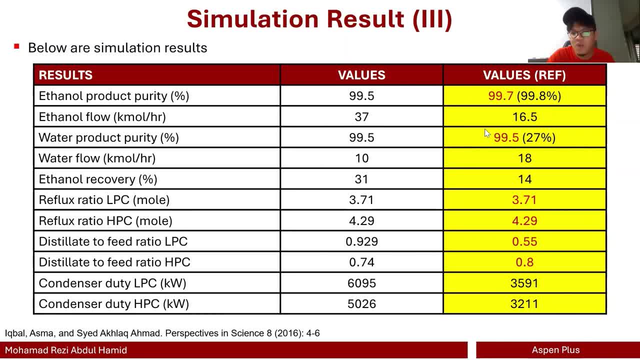 percent, percent of water purity which does not satisfy of water purity which does not satisfy of water purity which does not satisfy their requirement, and i their requirement and i their requirement and i, i don't know why, but this is something. i don't know why, but this is something. 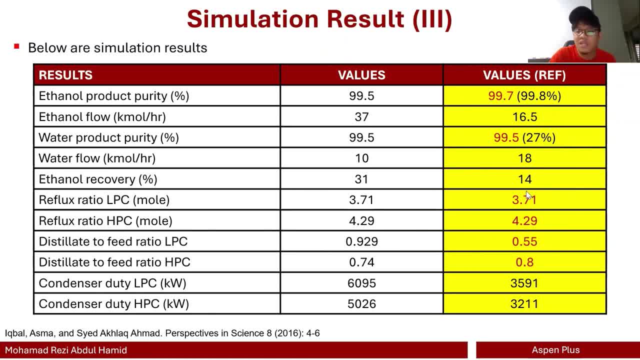 i don't know why, but this is something that i that i feel that that i got when that i that i feel that that i got when that i that i got when i simulate, i simulate, i simulate: uh the the process using their own, uh, the the process using their own. 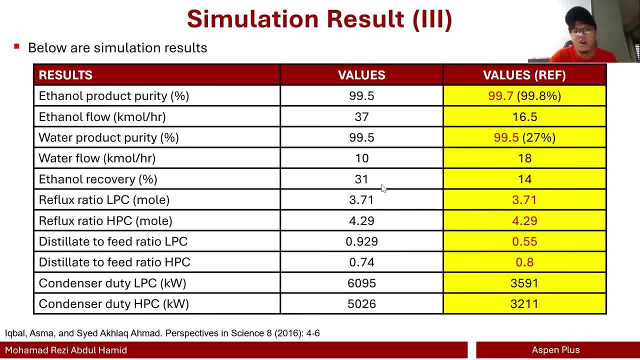 uh, the the process using their own values, which is this one? values which is this one, values which is this one. i don't know why, but uh, but overall i. i don't know why, but uh, but overall i. i don't know why, but uh, but overall i think i, i satisfy the purity requirement. 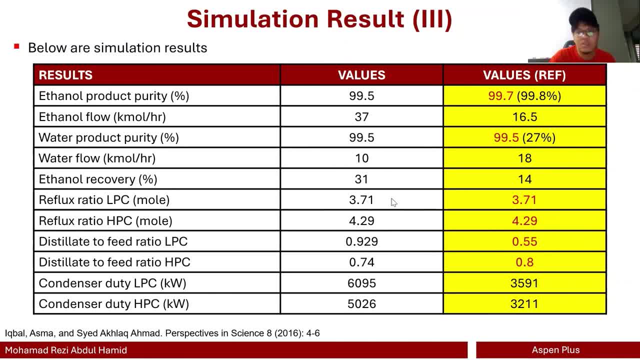 think i i satisfy the purity requirement. think i i satisfy the purity requirement. i have my all. i have my all. i have my all. these are all the condition of my high. these are all the condition of my high. these are all the condition of my high pressure column. 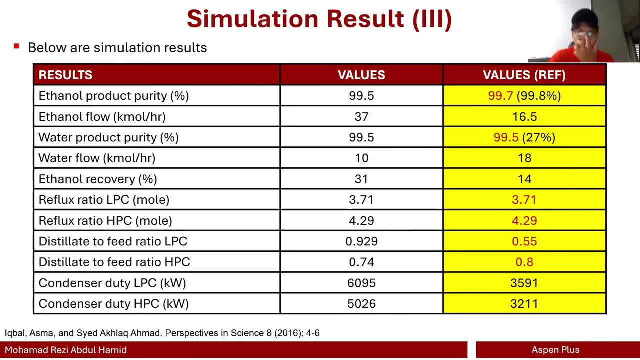 pressure column: pressure column and low pressure column, so to summarize, and low pressure column, so to summarize, and low pressure column, so to summarize. um, um, um. you can always break the azotrope of. you can always break the azotrope of. you can always break the azotrope of ethanol water mixtures by changing the. 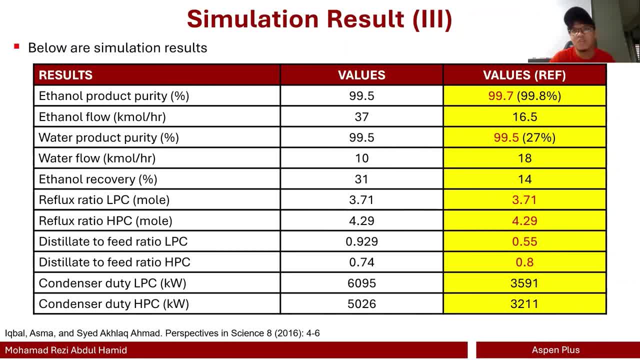 ethanol water mixtures. by changing the ethanol water mixtures, by changing the, the pressure of your, the pressure of your, the pressure of your column, obviously you can use uh, maybe column. obviously you can use uh, maybe column. obviously you can use uh, maybe even lower pressure condition if you. 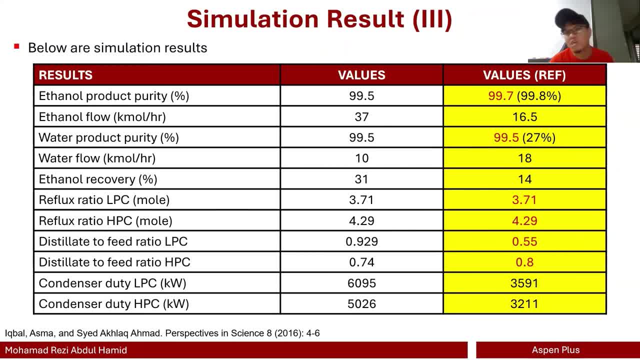 even lower pressure condition, if you even lower pressure condition, if you want, want, want. because you know when we deal with a, because you know when we deal with a, because you know when we deal with a high pressure column, obviously to have a high pressure column, obviously to have a. 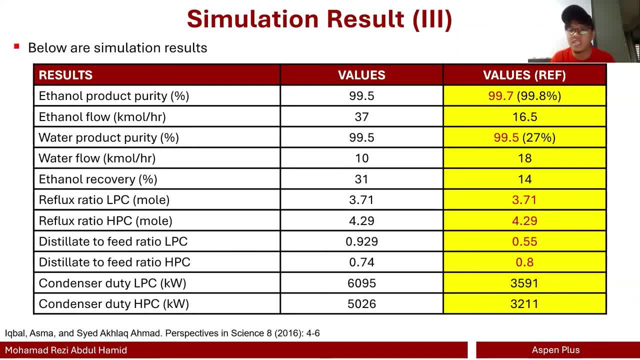 high pressure column. obviously, to have a thicker uh thicker column wall, it costs thicker uh thicker column wall. it costs thicker uh thicker column wall. it costs money and things like that. but maybe you money and things like that, but maybe you money and things like that, but maybe you will save some costs in terms of like. 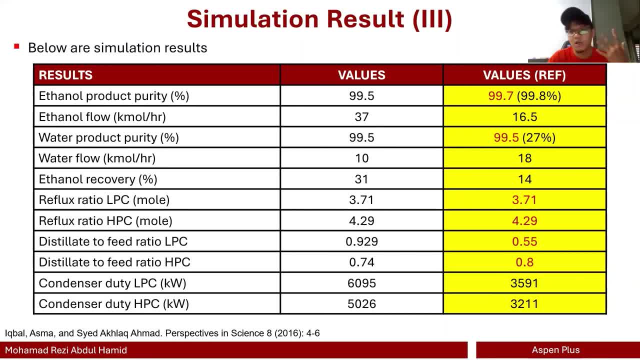 will save some costs in terms of like will save some costs in terms of like, operating costs. who knows i don't know operating costs. who knows i don't know operating costs? who knows, i don't know. but those are, those are the few things, but those are, those are the few things. 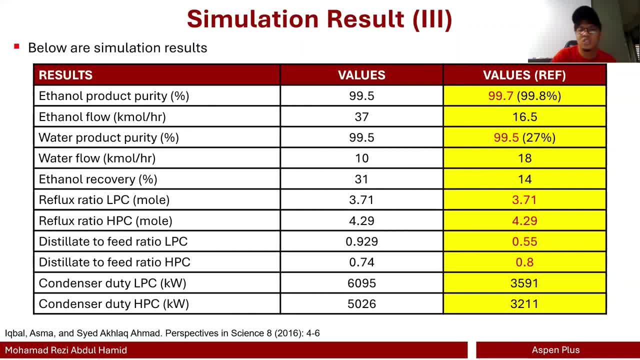 but those are. those are the few things that you need to consider when you uh do that. you need to consider when you uh do that. you need to consider when you uh do this pleasure swing, uh distillation, okay, um, that would be all for me, um, if, 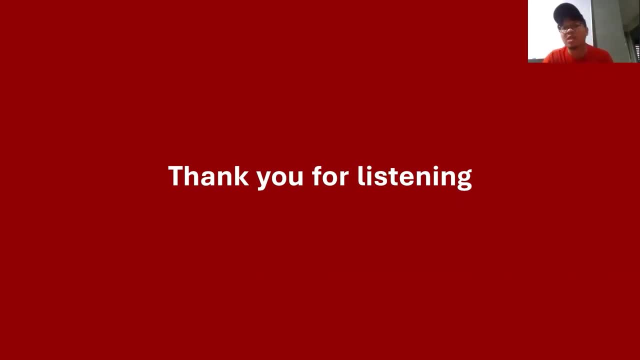 okay, um, that would be all for me, um, if okay, um, that would be all for me. um. if you like the videos, give it a thumbs up. you like the videos? give it a thumbs up. you like the videos, give it a thumbs up. consider subscribing to my channels if. 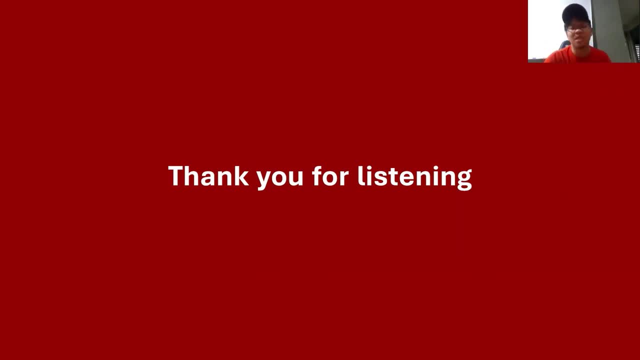 consider subscribing to my channels, if consider subscribing to my channels, if you like, and i will see you again in you like, and i will see you again in you like, and i will see you again in the next video, the next video, the next video, goodbye. 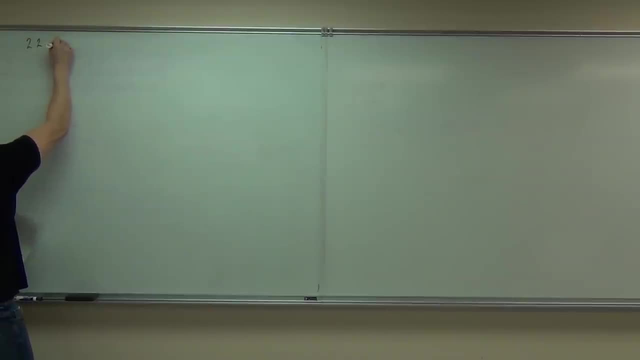 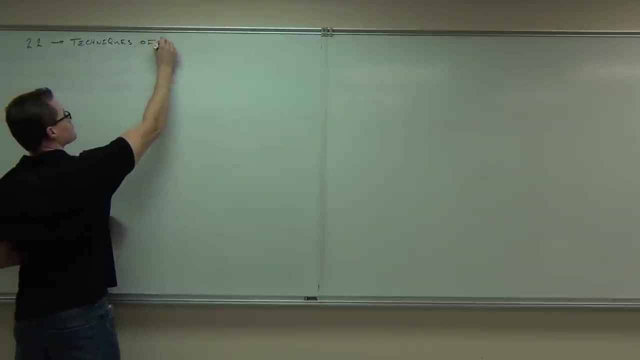 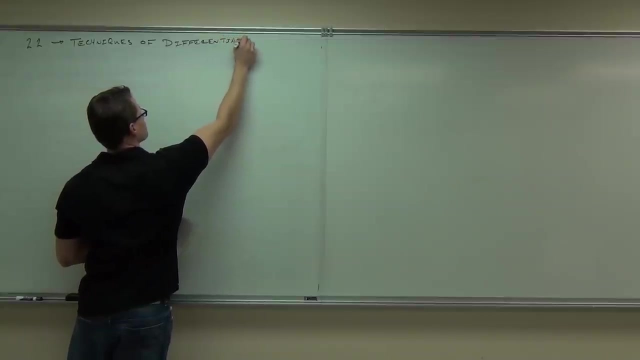 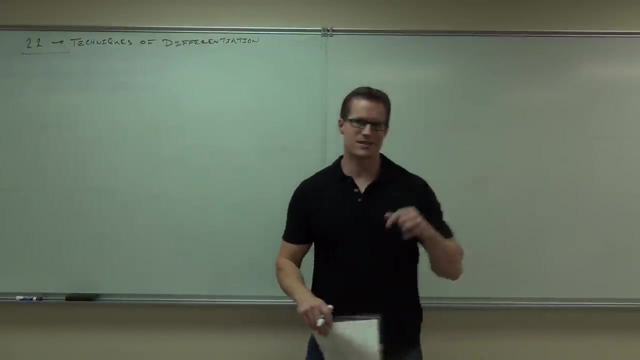 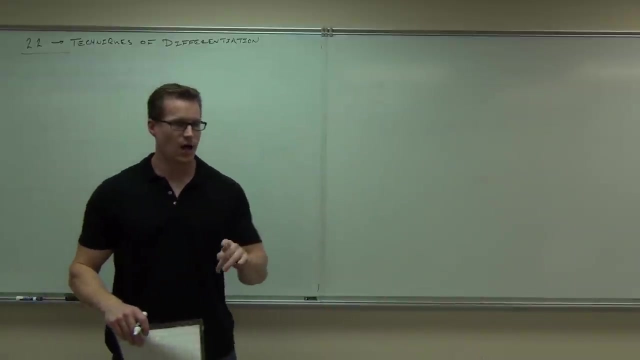 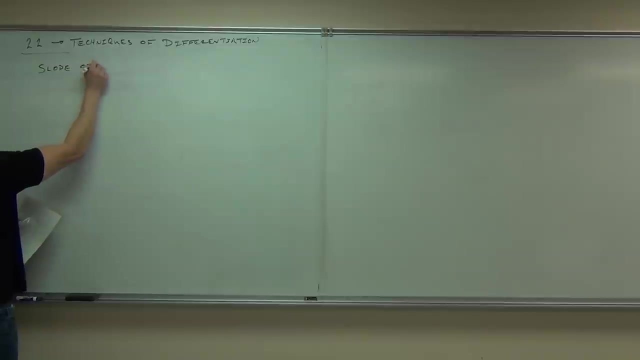 We're going to start off nice and simple. I want to talk about the derivative of any horizontal line. What happens if I try to find the slope of a constant? So, for instance, slope of a constant. when you graph a constant, what do you get?